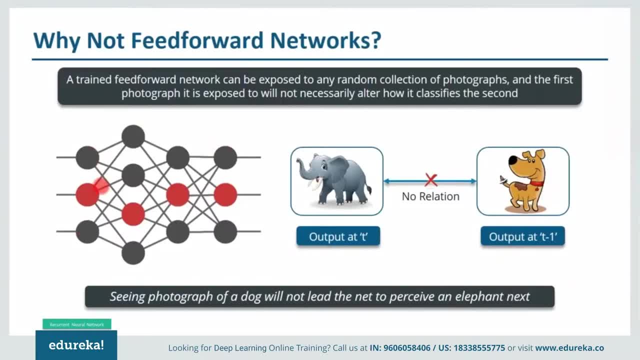 we have trained this particular network for classifying various images of animals. Now, if we feed in an image of a dog, it will identify that image and will provide a relevant label to that particular image. Similarly, if we feed in an image of an elephant, it will provide. 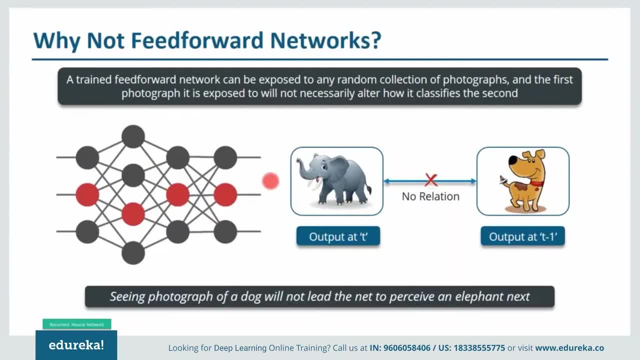 a relevant label to that particular image as well. Now, if you notice, the new output that we have got that is classifying an elephant has no relation with the previous output that is of a dog. Or you can say that the output at time t is independent of output. 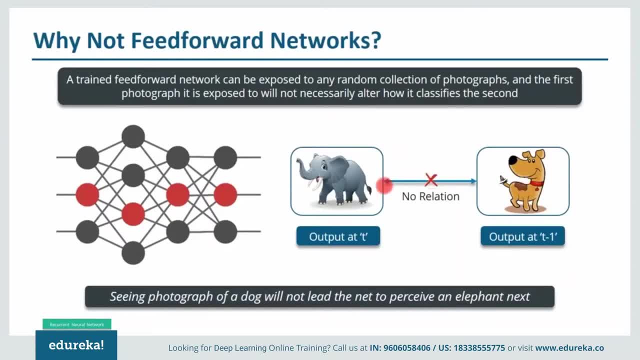 at time t minus one, As we can see that there is no relation between the new output and the previous output, So we can say that in feedforward networks, outputs are independent to each other. Now there are a few scenarios where we actually need the previous output to get the new output. Let 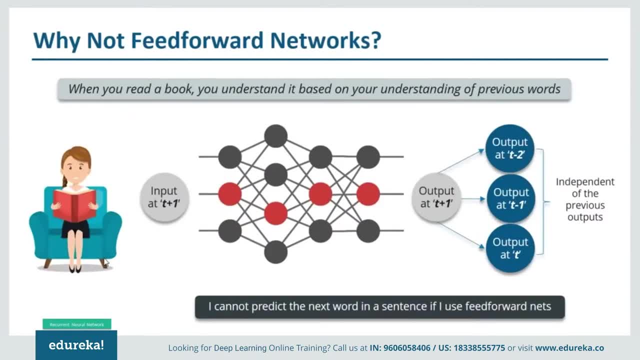 us discuss one such scenario. Now, what happens when you read a book? You'll understand that book only on the understanding of your previous words. Alright, so if I use a feedforward network and try to predict the next word in a sentence, I can't do that. Why can't I do? 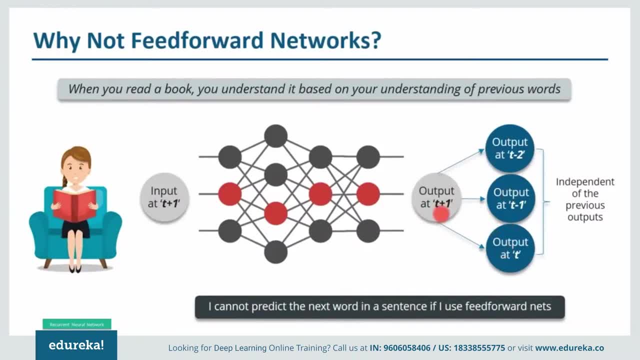 that. Well, you can see that I have to depend on the previous outputs. But in the feedforward network my new output is independent of the previous outputs. that is, output at t plus one has no relation with output at t minus two, t minus one and t. So basically, we cannot. 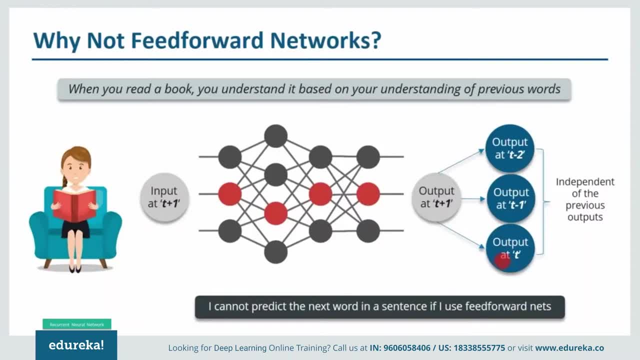 use feedforward networks for predicting the next word in a sentence. Similarly, you can think of many other examples where we need the previous output, some information from the previous output, so as to infer the new output. This is just one small example there. 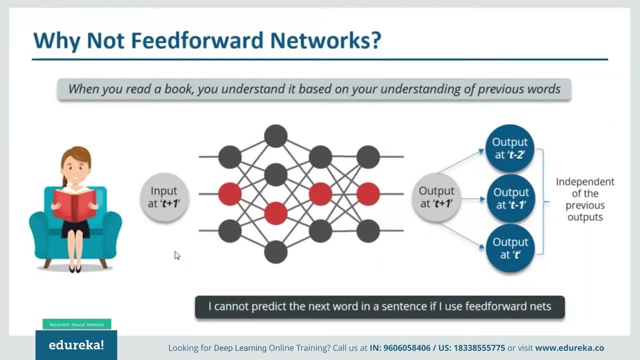 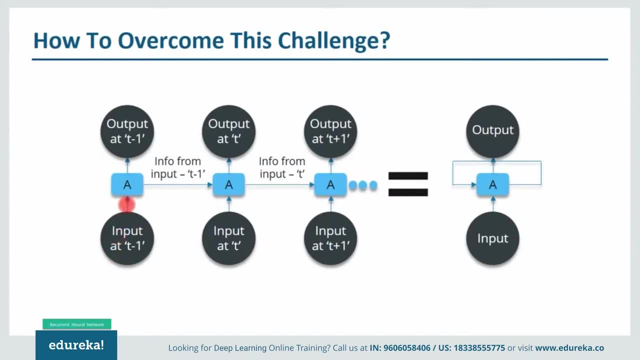 are many other examples that you can think of. So we'll move forward and understand how we can solve this, this particular problem. So over here what we have done: we have input at t minus 1, we'll feed it to our network, then we'll get the output at t minus 1.. Then at the next time stamp, that is, at time t. 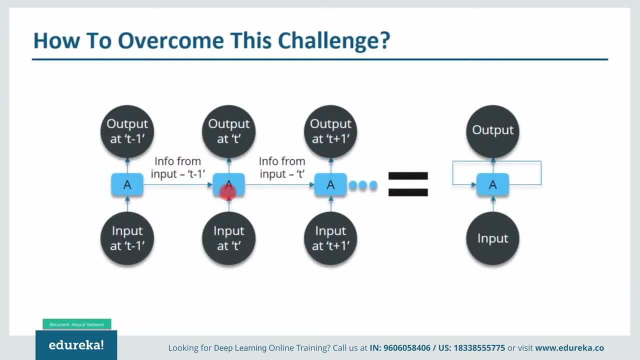 we have input at time t that will be given to our network along with the information from the previous time stamp, that is, t minus 1, and that will help us to get the output at t. Similarly, at output for t plus 1, we have two inputs. one is a new input that we give, another is the information. 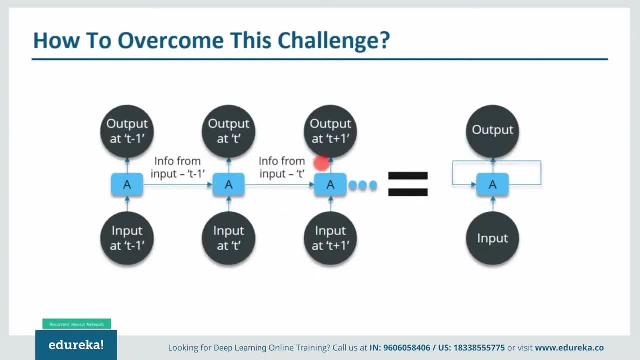 coming from the previous time stamp, that is t, in order to get the output at time, t plus 1.. Similarly, it can go on So over here. I have just written a generalized way to represent it. there's a loop where the information from the previous time stamp is flowing, and this is how. 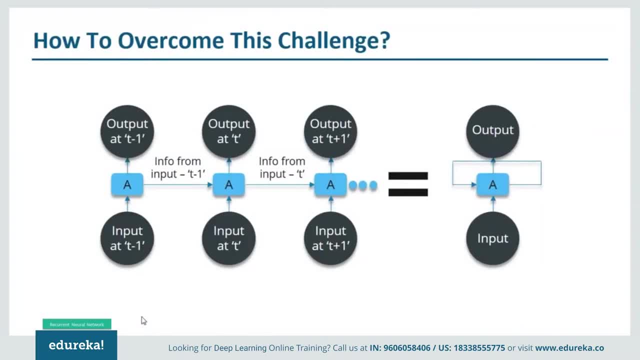 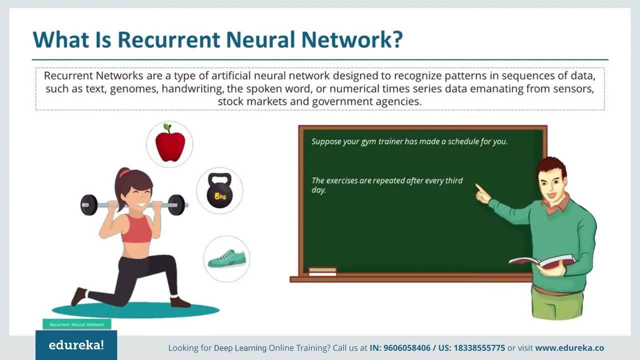 we can solve this particular challenge. Now let us understand what exactly are recurrent neural networks. So for understanding recurrent neural network, I'll take an analogy. Suppose your gym trainer has made a schedule for you. The exercises are repeated after every third day. Now this is. 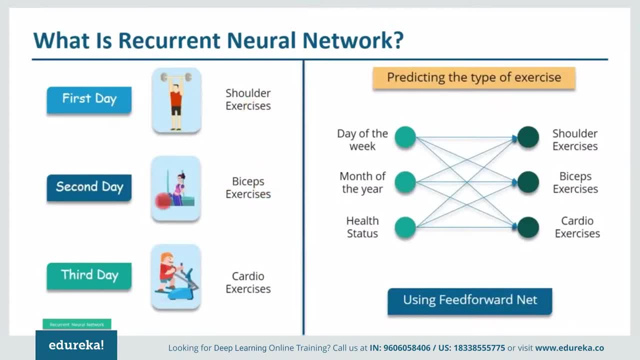 the order of time. So let's say you have a gym trainer and you have a gym trainer and you have your exercises. First day you'll be doing shoulders. Second day you'll be doing biceps. Third day, you'll be doing cardio, And all these exercises are repeated in a proper order. Now what happens? 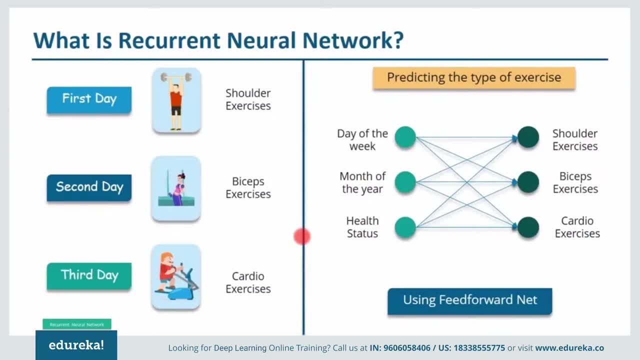 when we use a feed forward network for predicting the exercise today. So we'll provide in the input, such as day of the week, month of the year and health status, All right, And we need to train our model or a network on the exercises that we have done in the past. After that, there'll be a 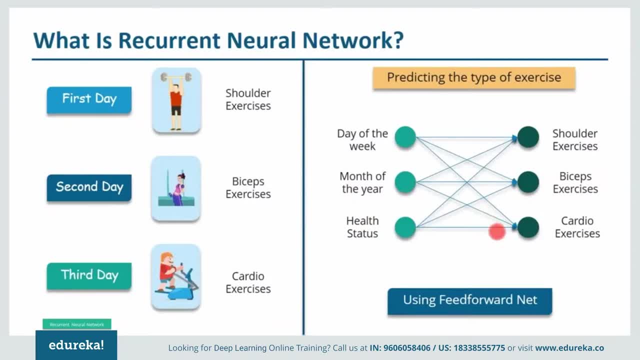 complex voting procedure involved that will predict the exercise for us And that procedure won't be that accurate. The output we'll get won't be as accurate as we want it to be. Now, what if I change my inputs and I make my inputs as what exercise I've done yesterday. So if I've done shoulder, then definitely today I'll be doing. 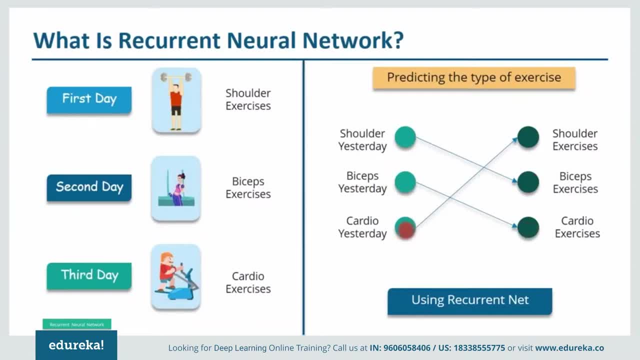 biceps. Similarly, if I've done biceps yesterday, today I'll be doing cardio. Similarly, if I've done cardio yesterday, today I'll be doing shoulder. Now there can be one scenario where you are unable to go to gym for one day, due to some personal reasons. you could not go to the gym Now. what will happen at that? 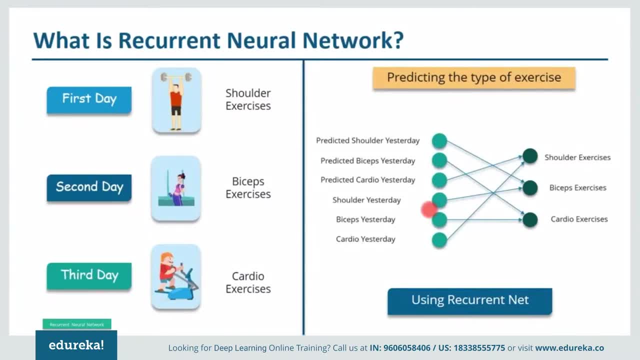 time. We'll go one time stamp back and we'll feed in what exercise we've done in the past And we'll get the result. So if I've done biceps exercise today, I'll be doing shoulder Now. what will happen at that time? We'll get the result. So if I've done biceps exercise today, I'll be doing shoulder Now. 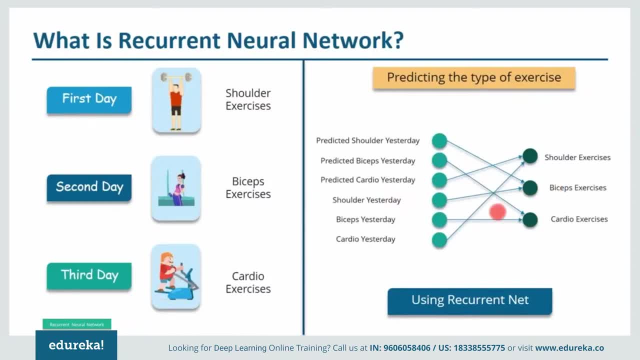 what will happen at that time? We'll get the result. So if I've done biceps exercise today, I'll be doing biceps exercise today, I'll be doing shoulder. Now what will happen at that time? We'll get the result. So 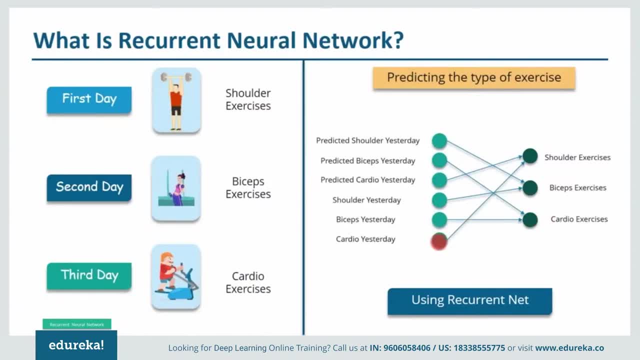 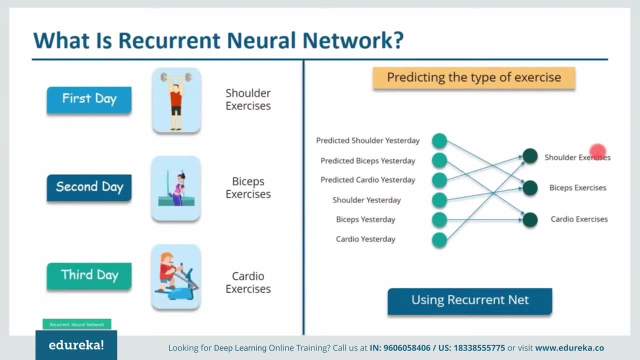 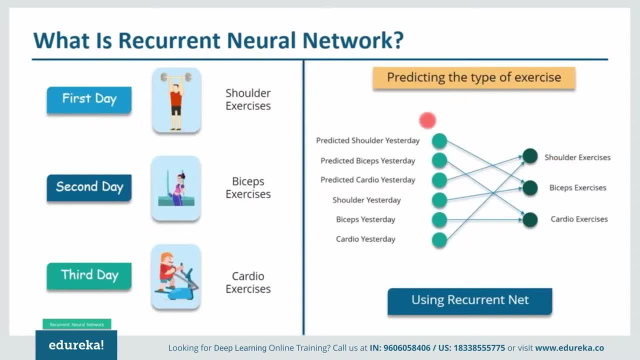 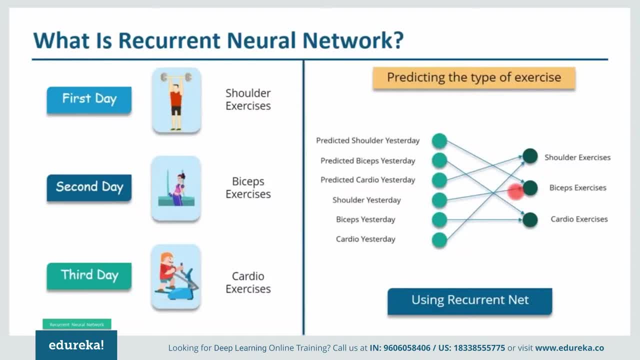 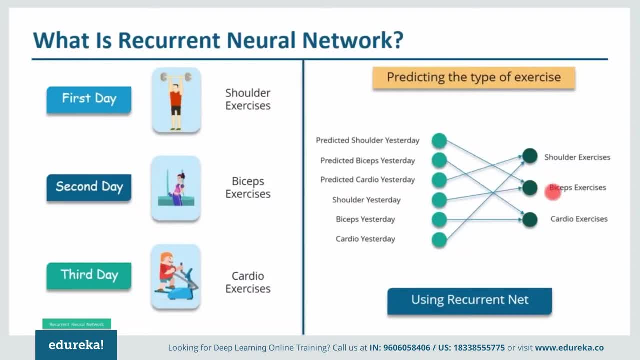 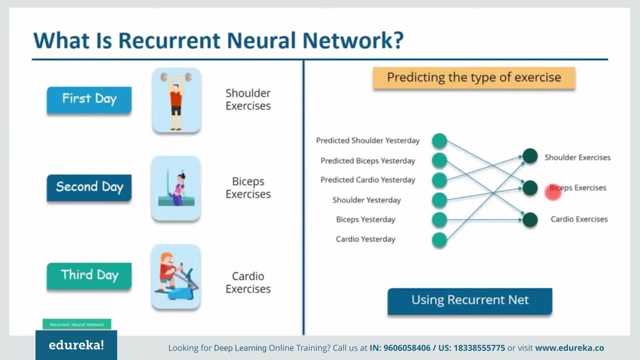 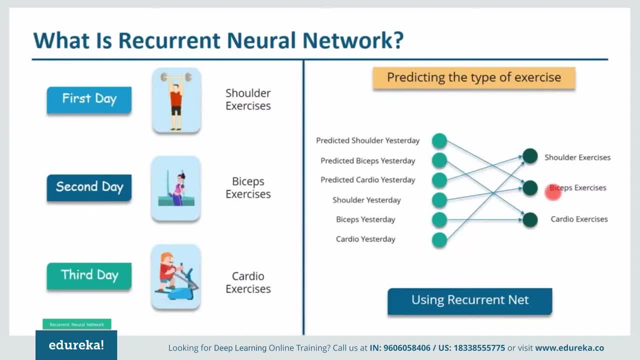 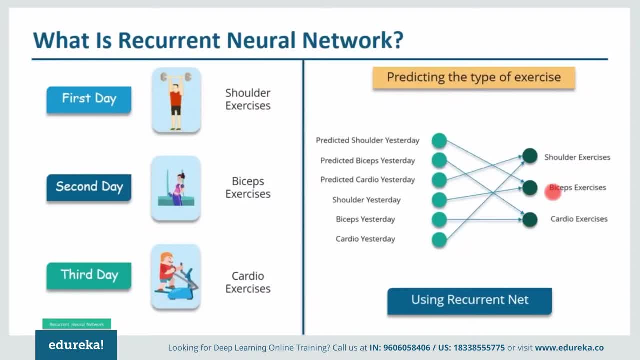 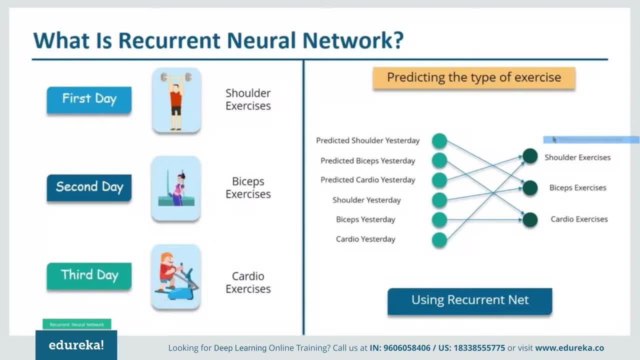 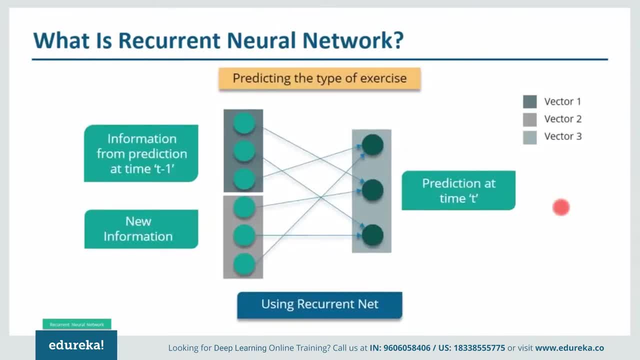 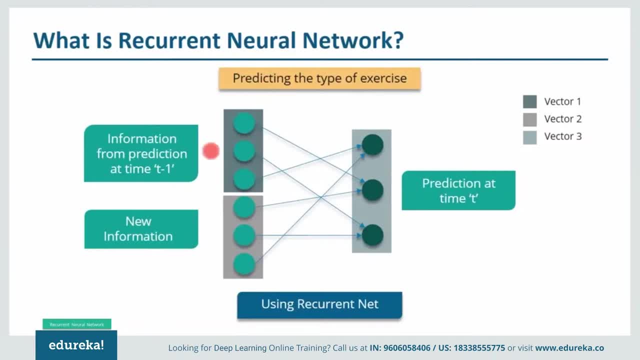 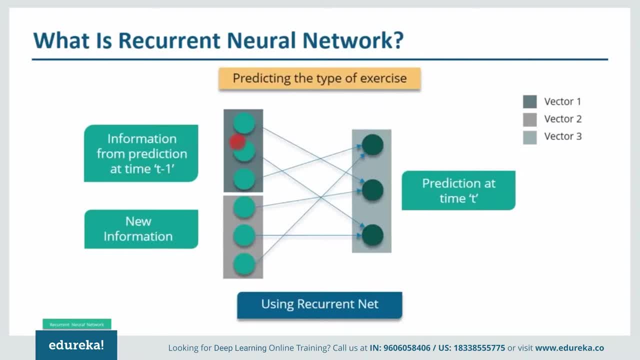 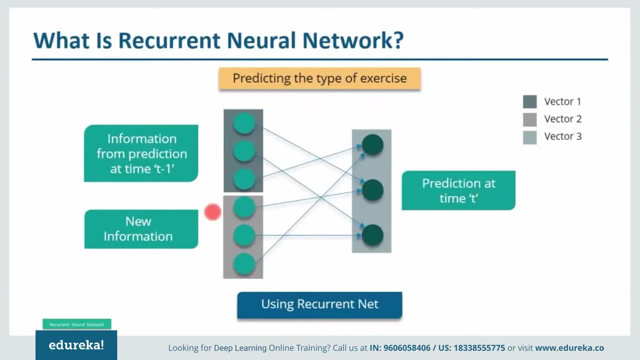 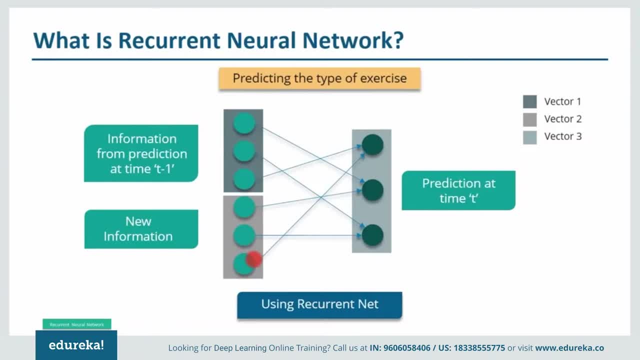 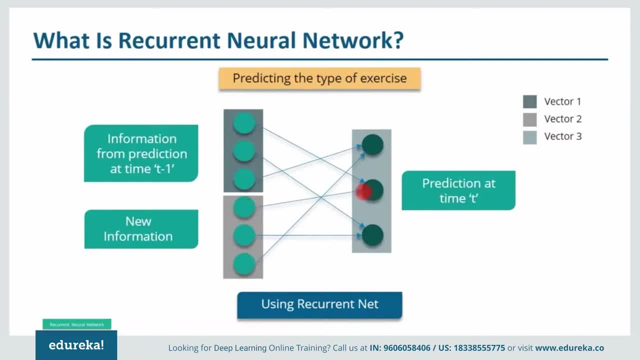 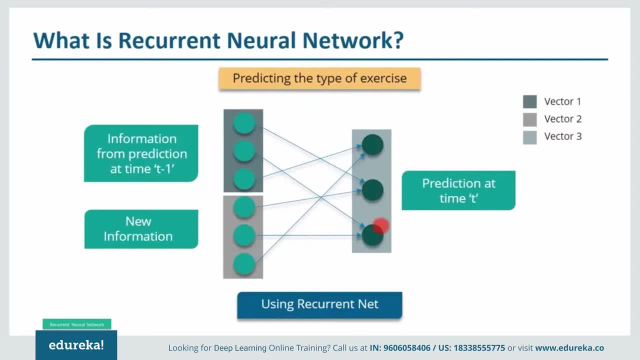 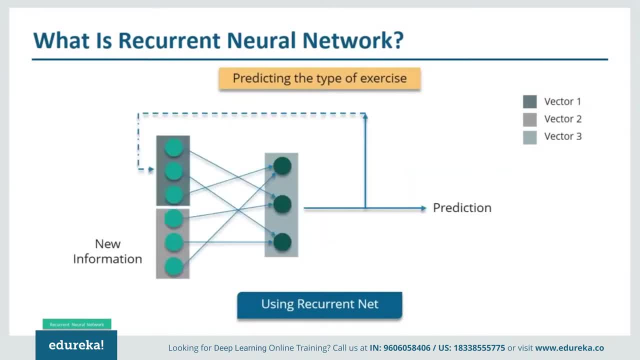 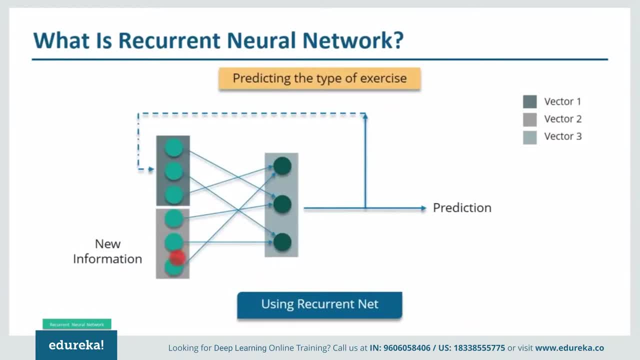 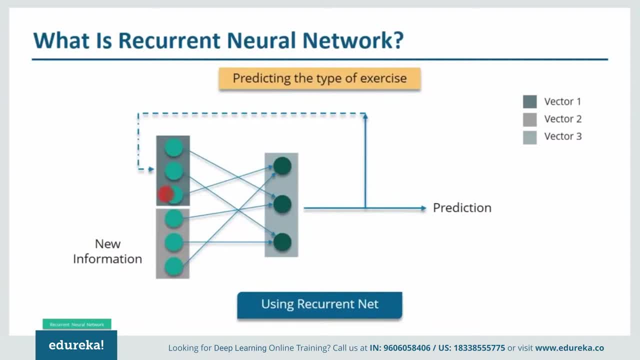 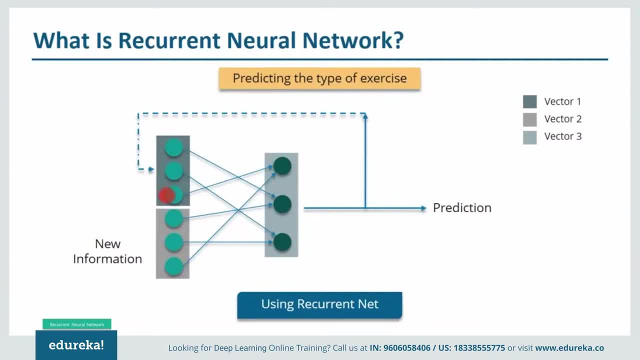 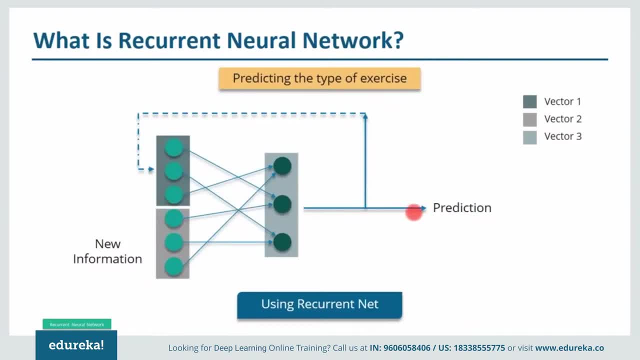 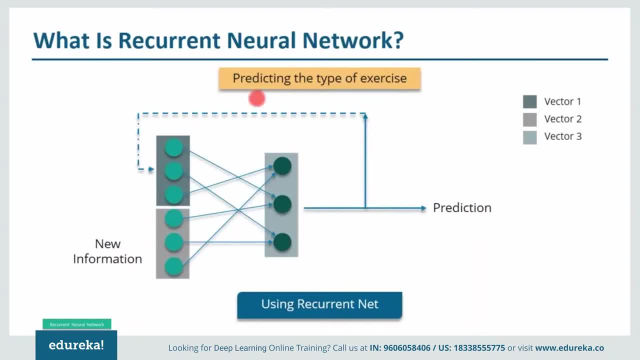 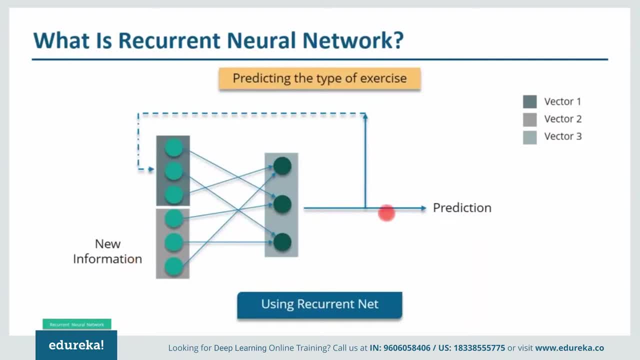 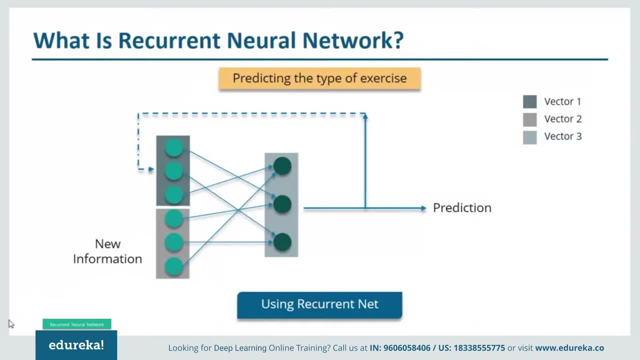 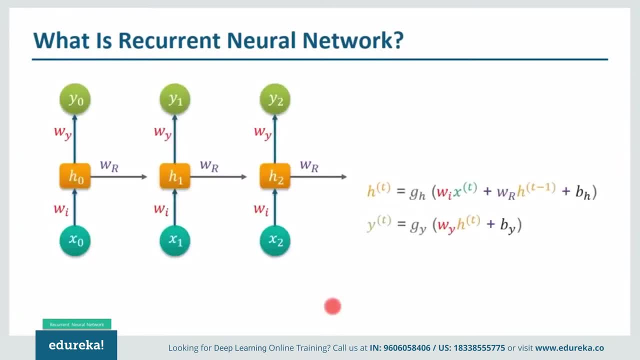 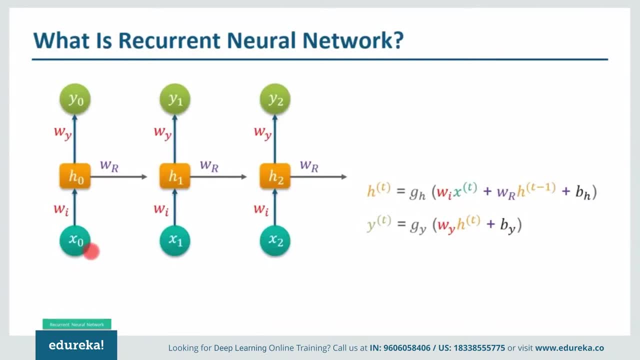 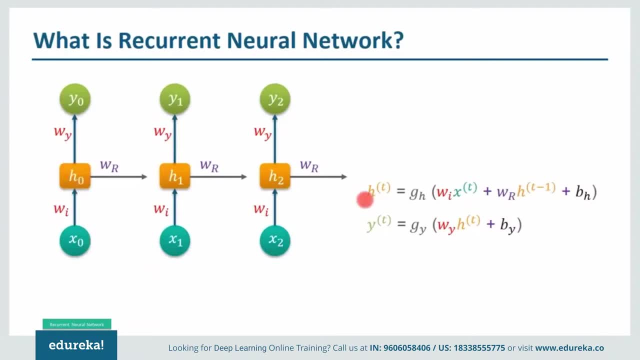 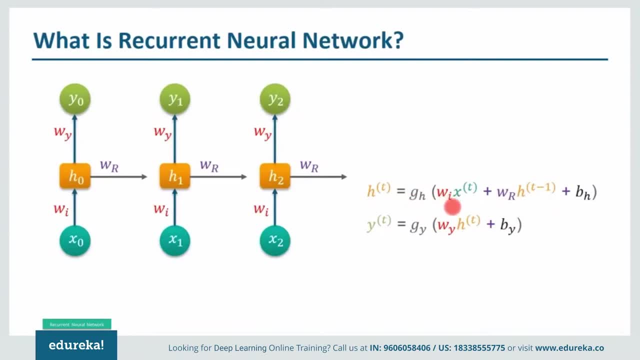 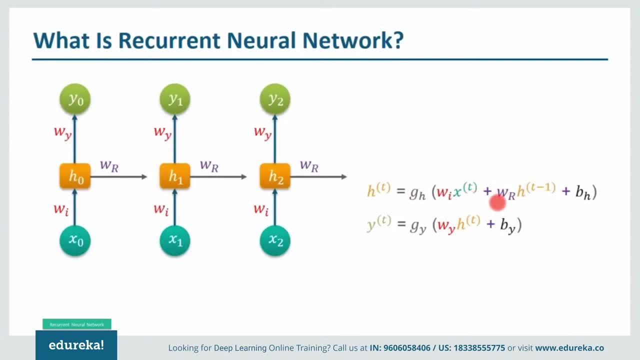 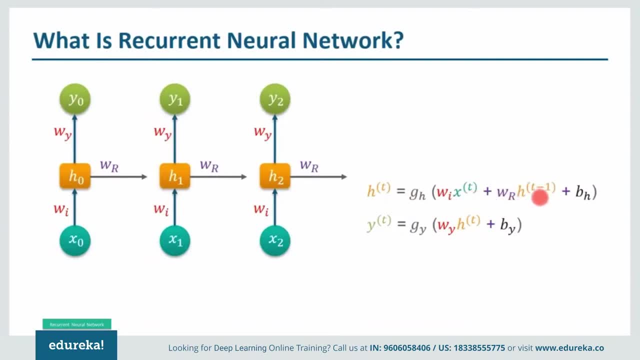 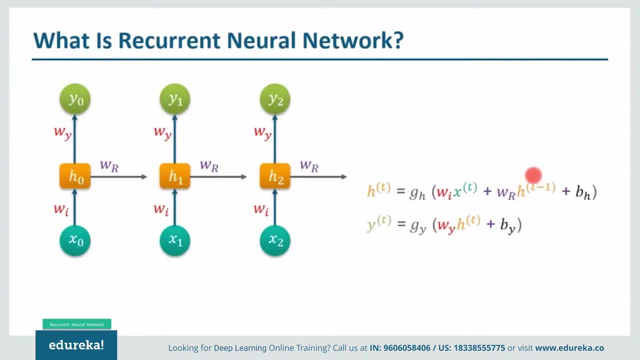 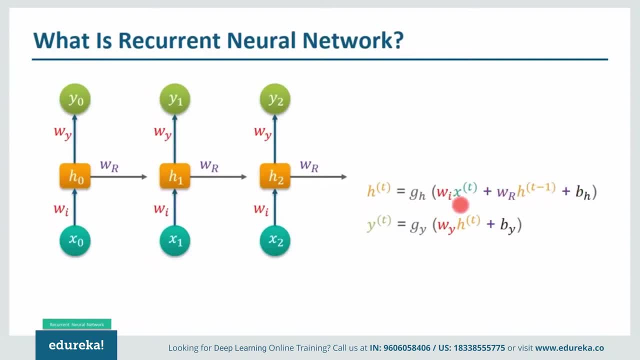 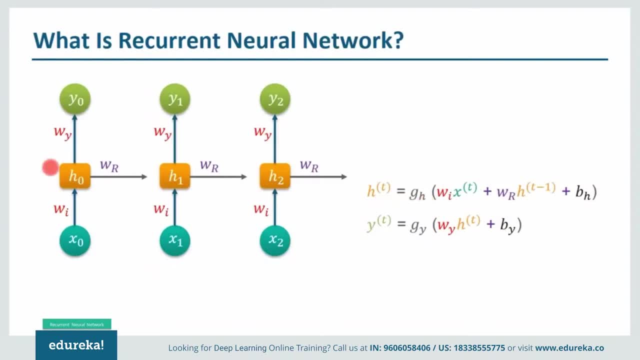 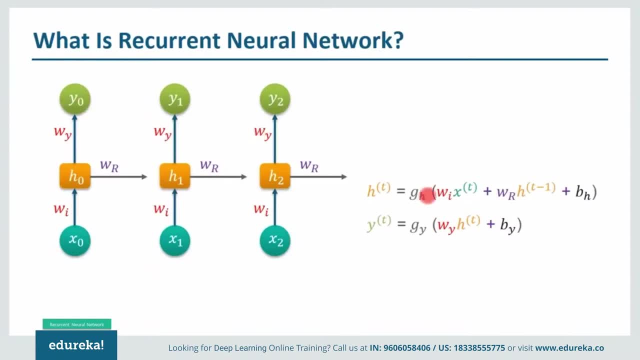 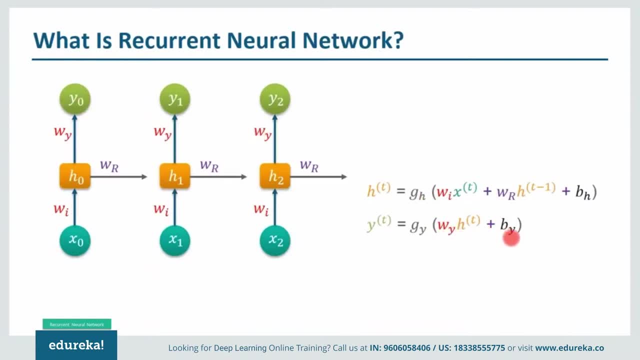 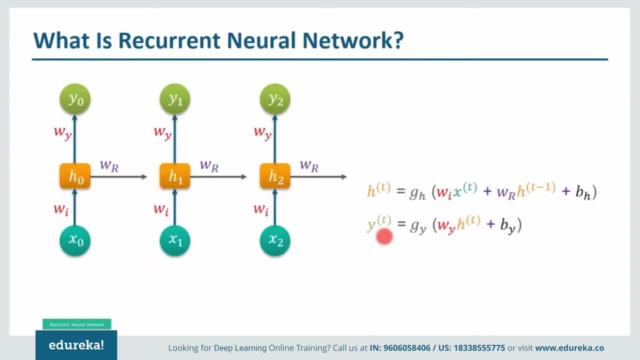 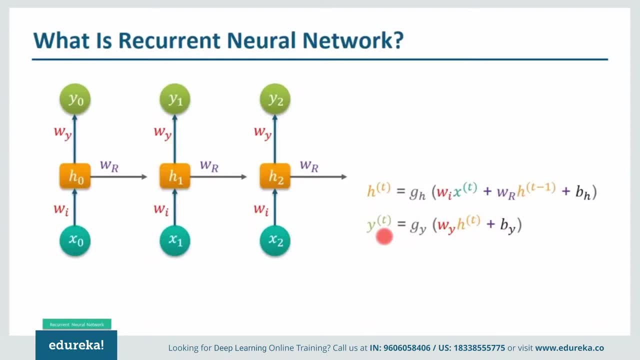 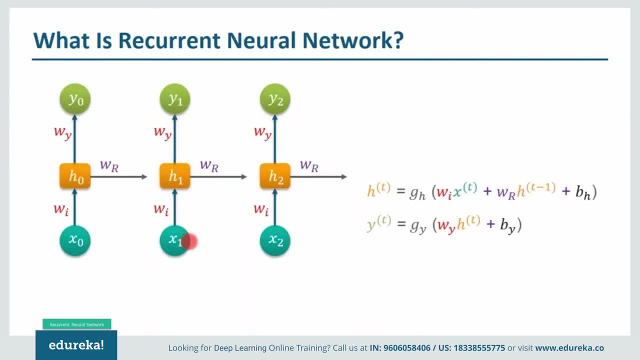 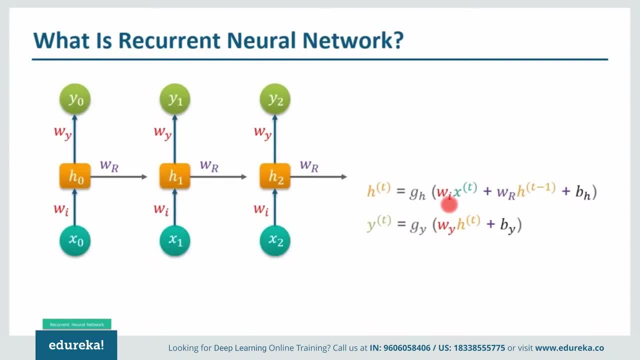 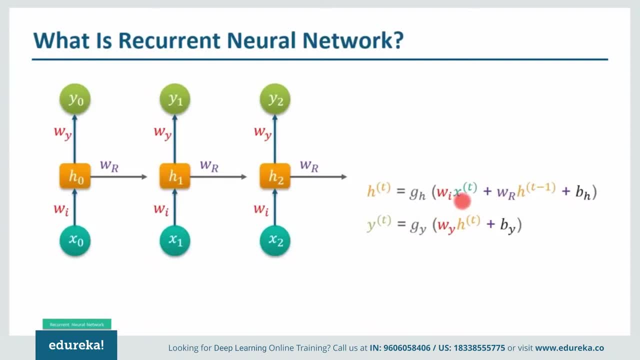 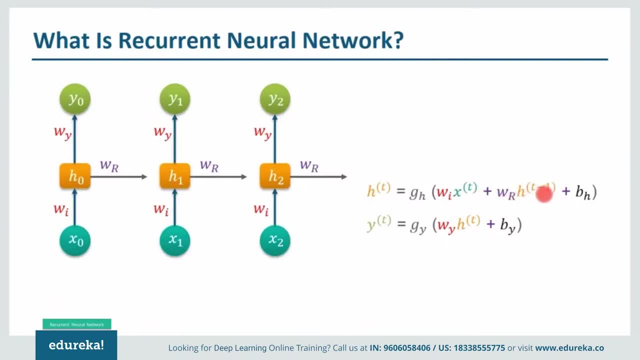 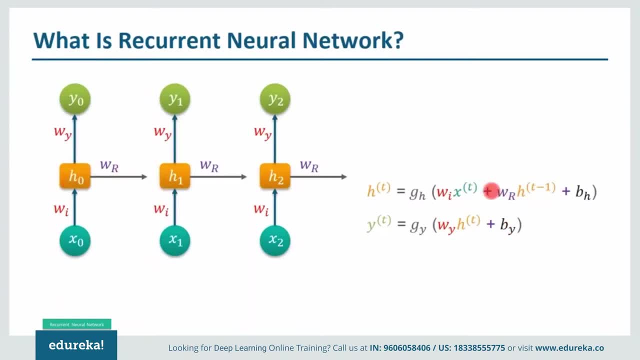 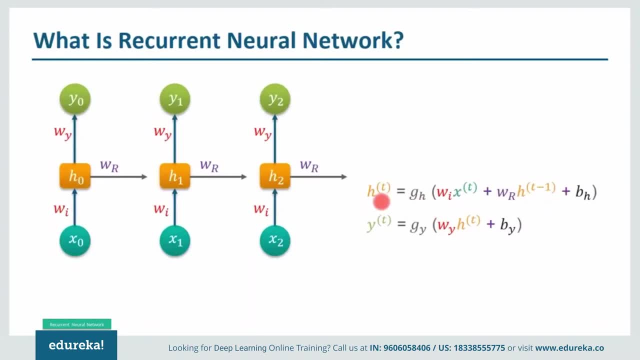 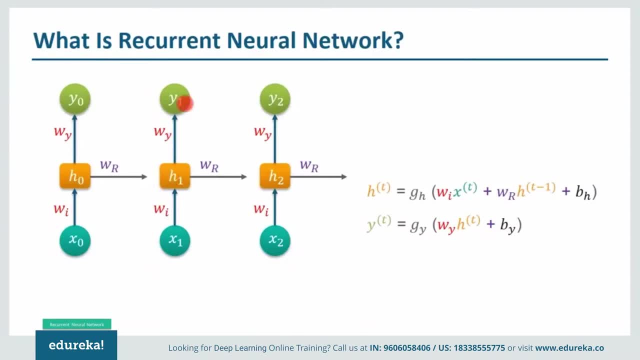 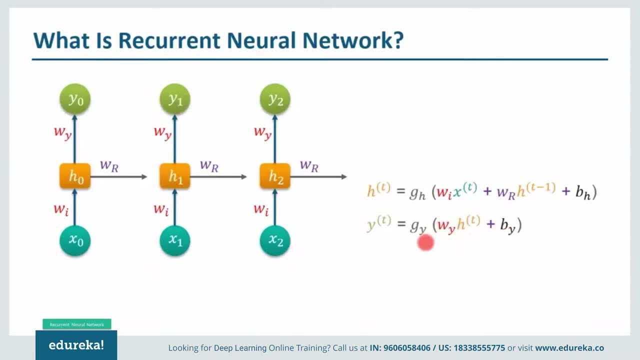 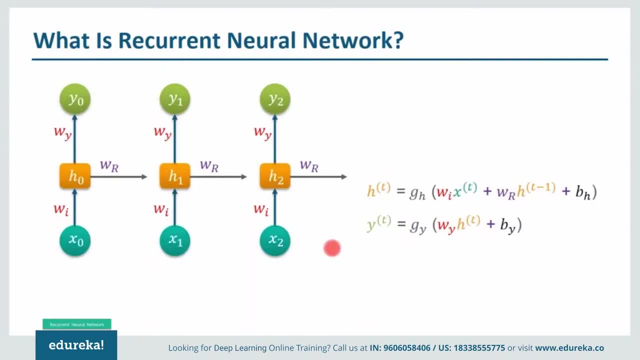 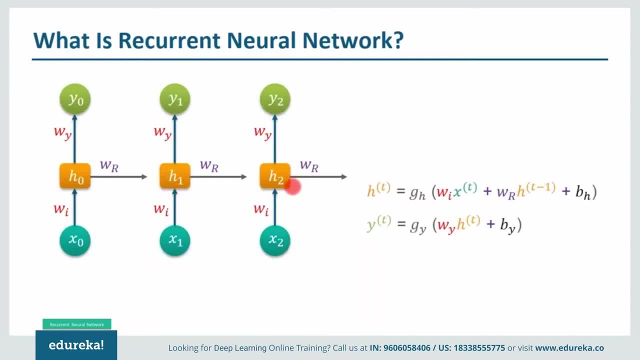 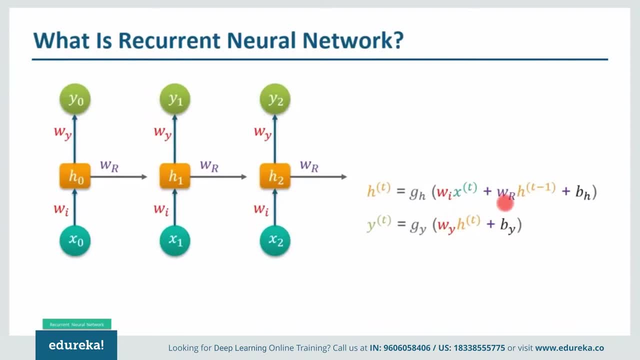 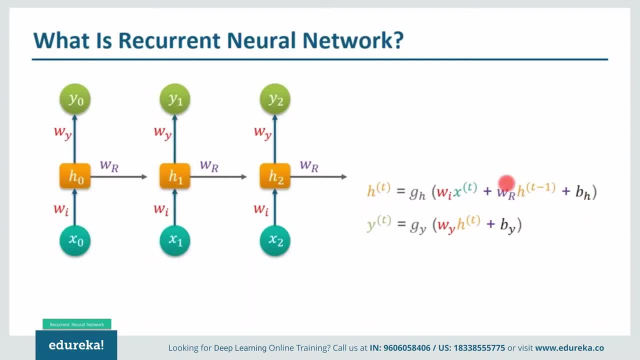 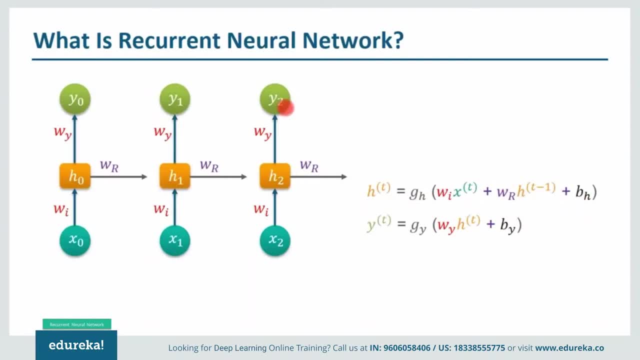 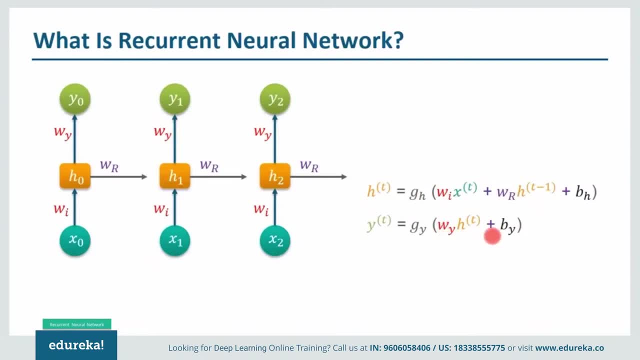 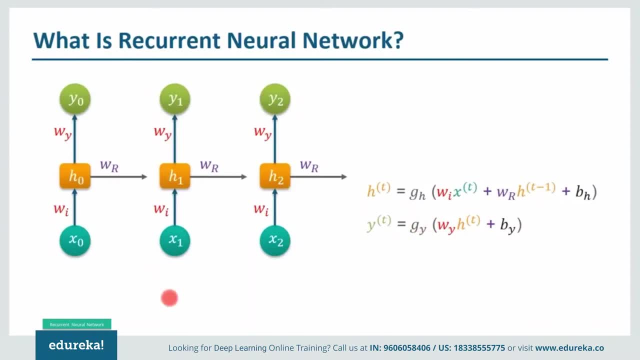 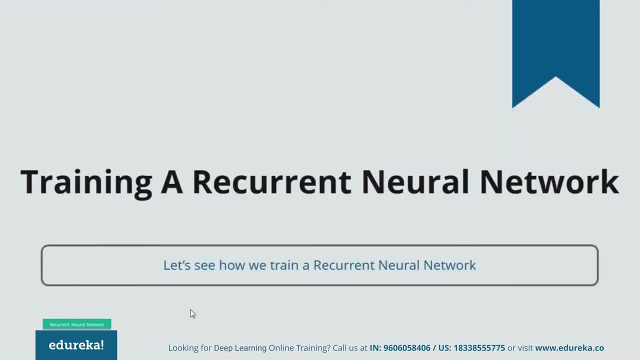 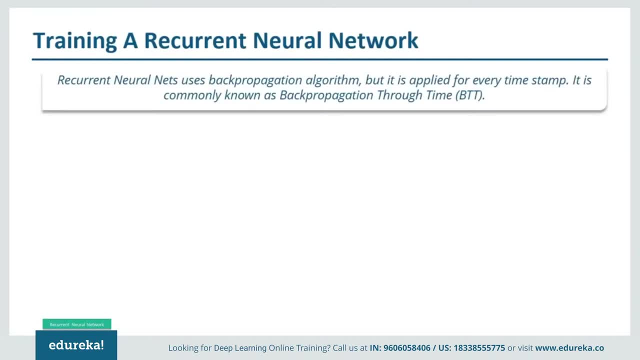 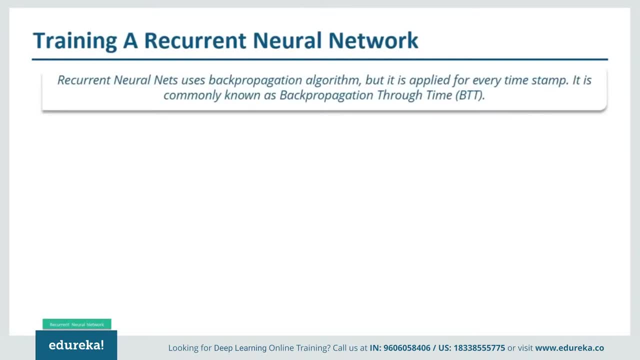 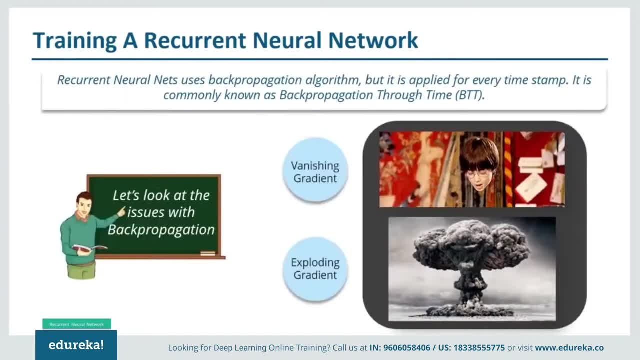 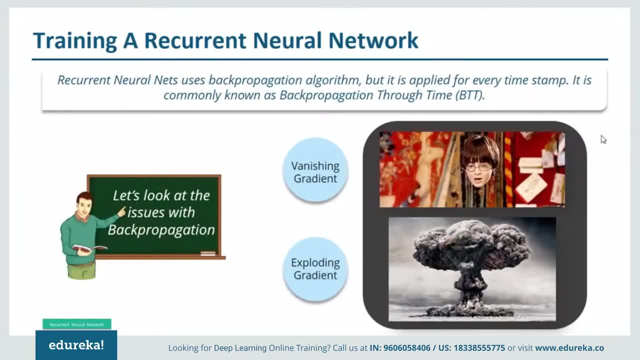 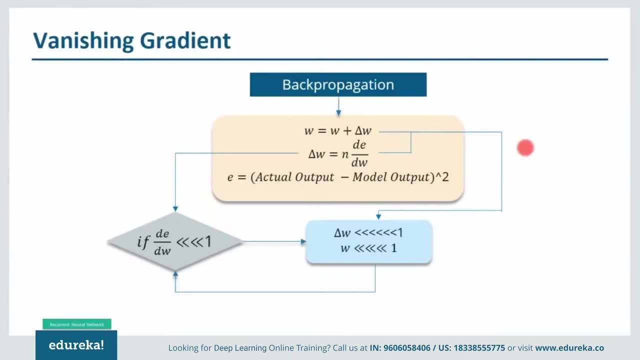 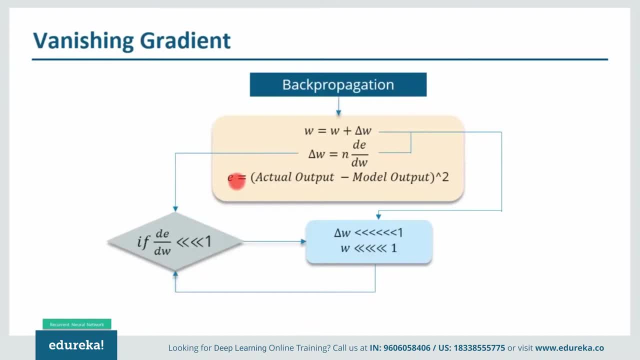 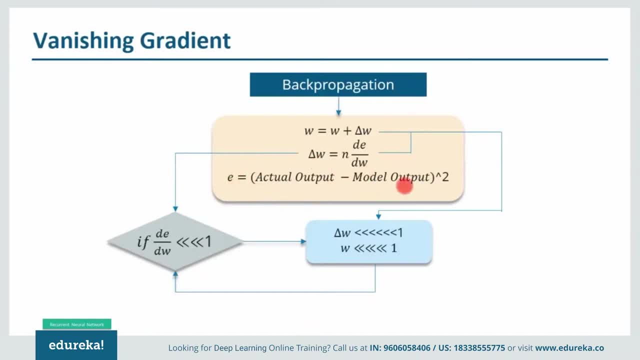 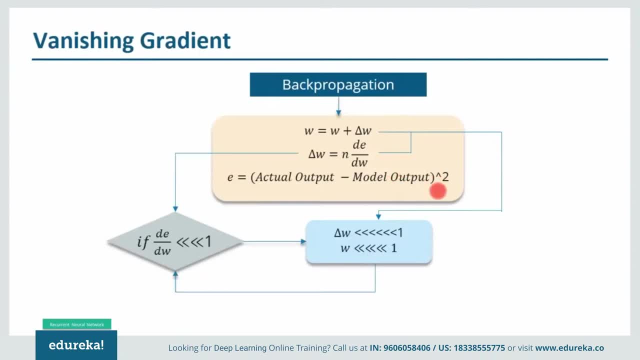 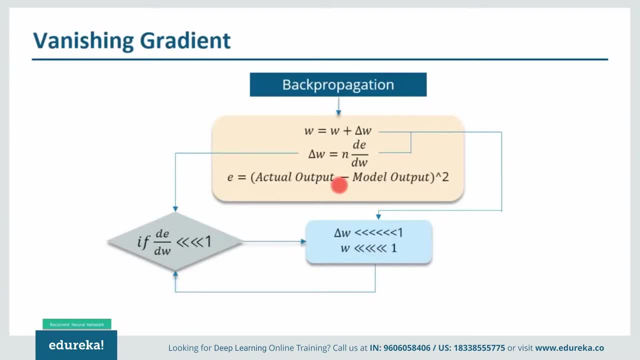 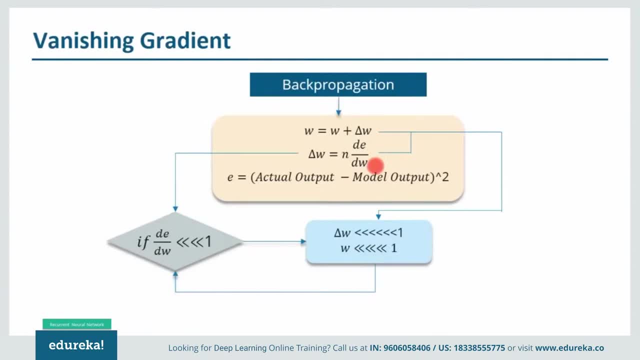 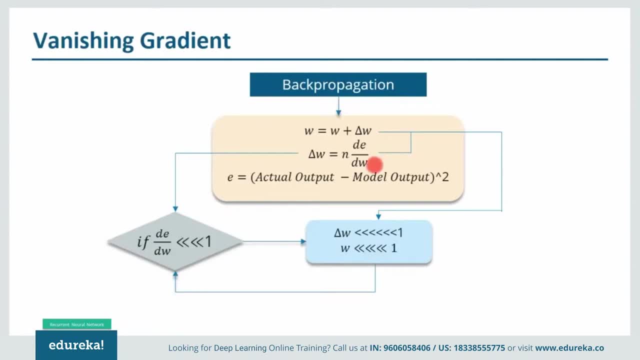 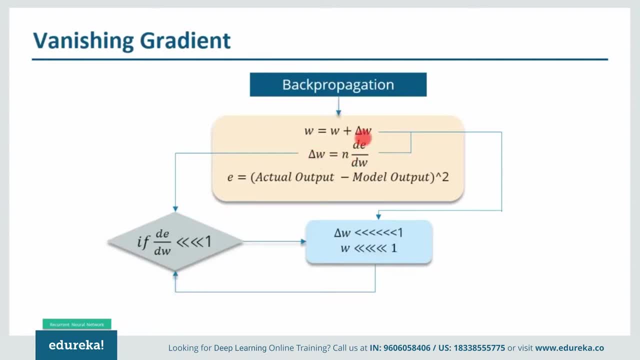 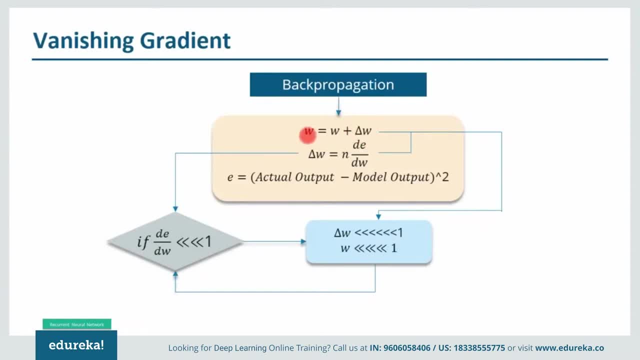 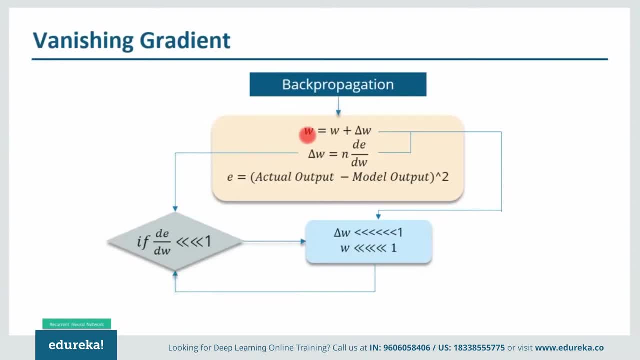 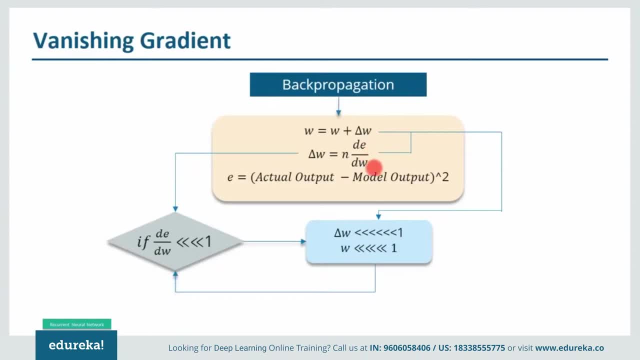 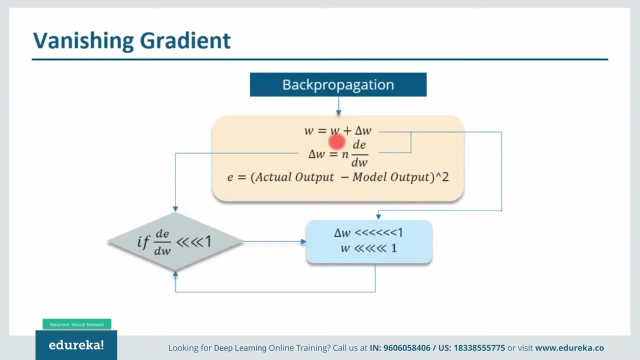 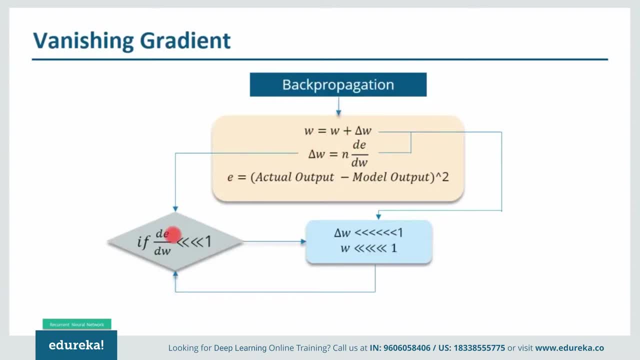 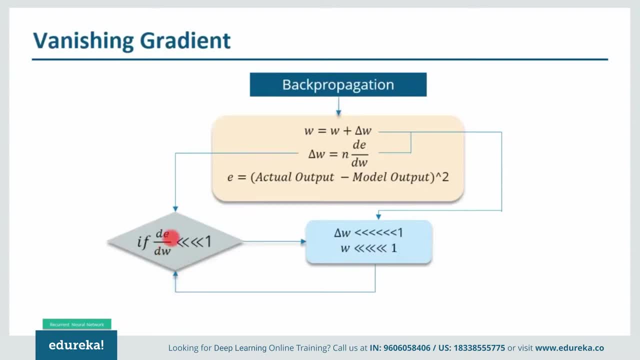 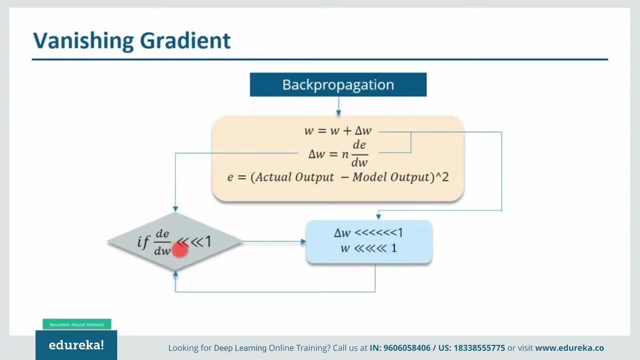 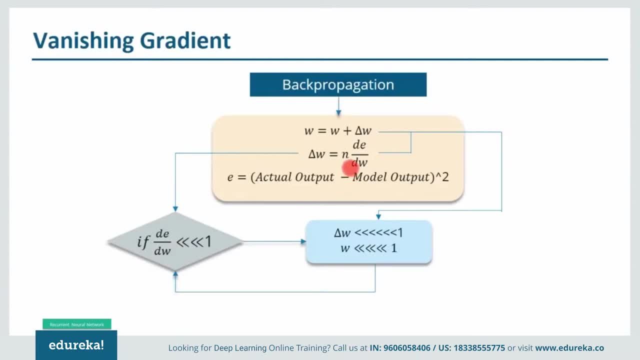 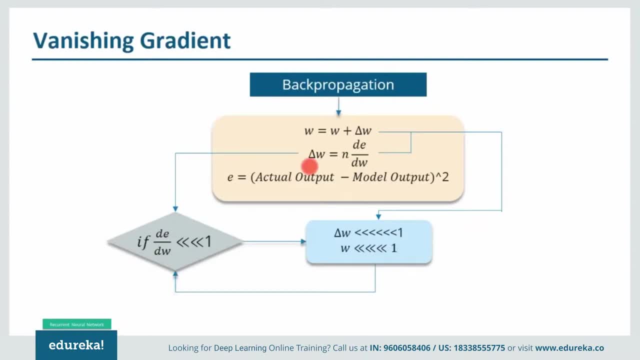 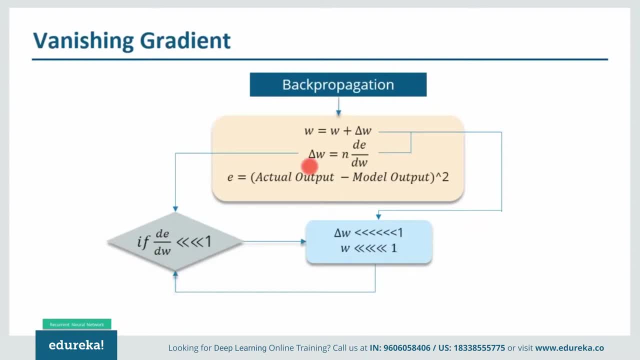 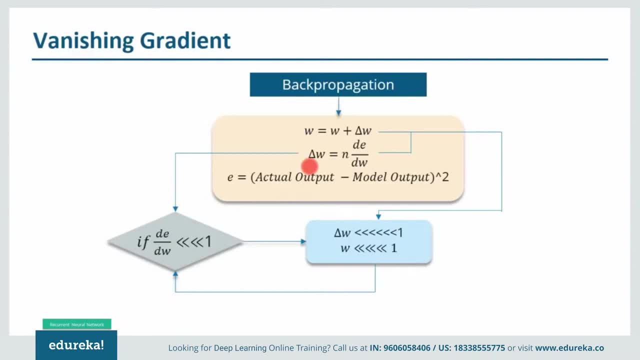 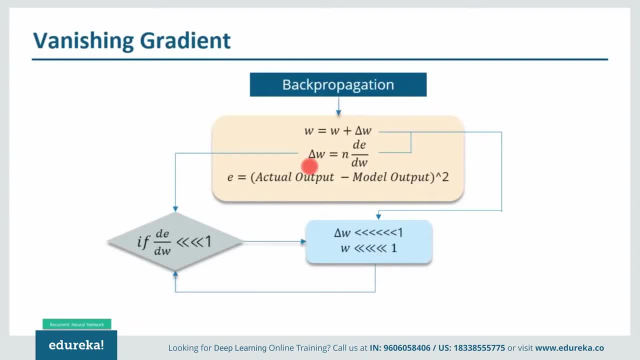 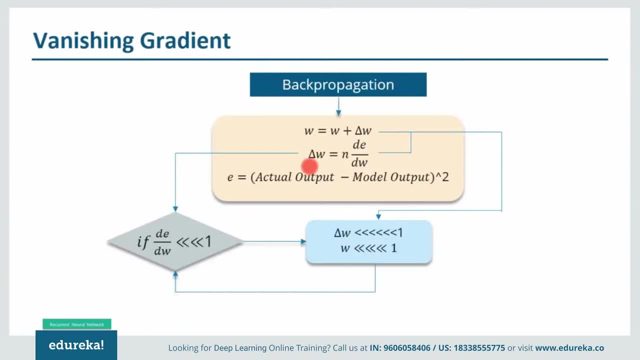 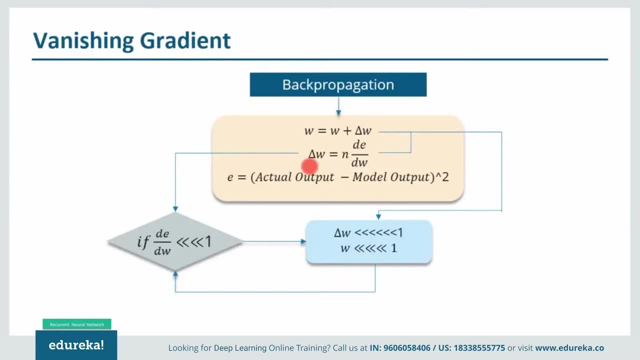 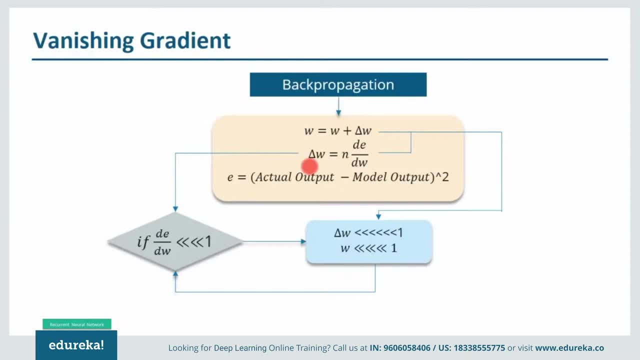 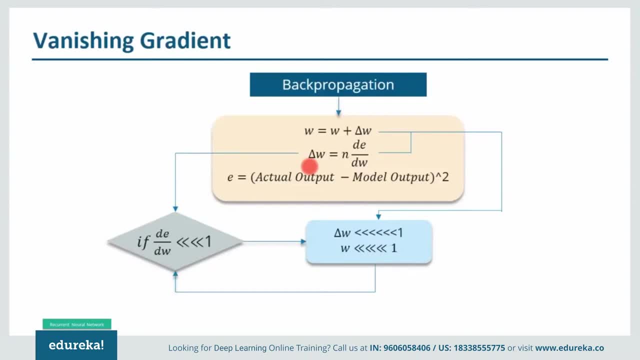 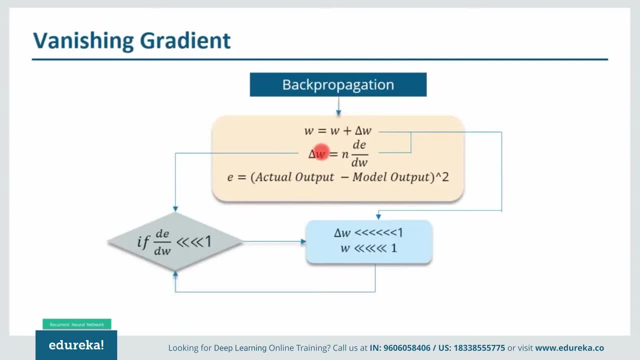 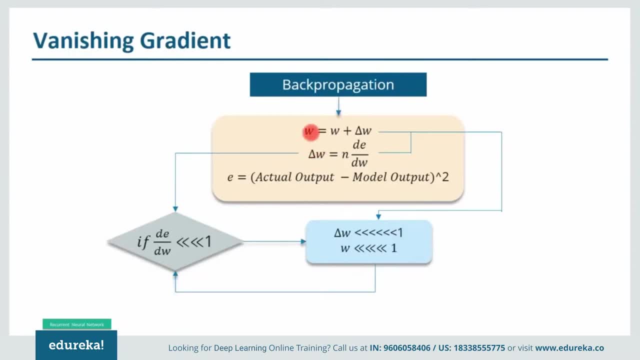 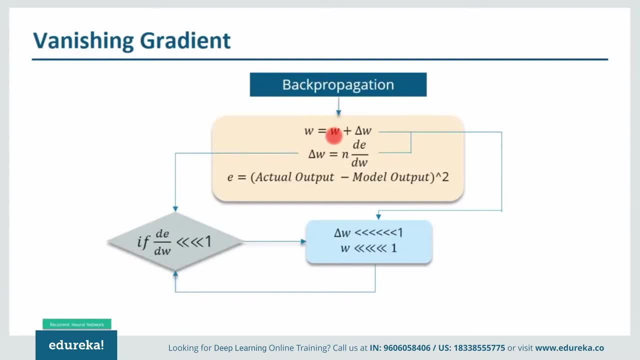 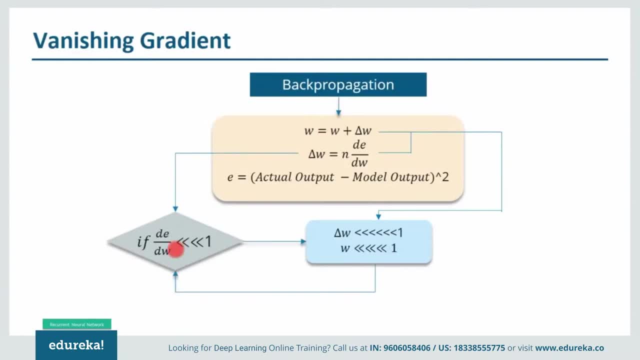 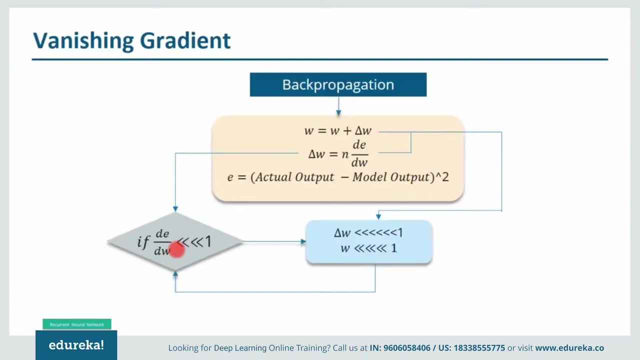 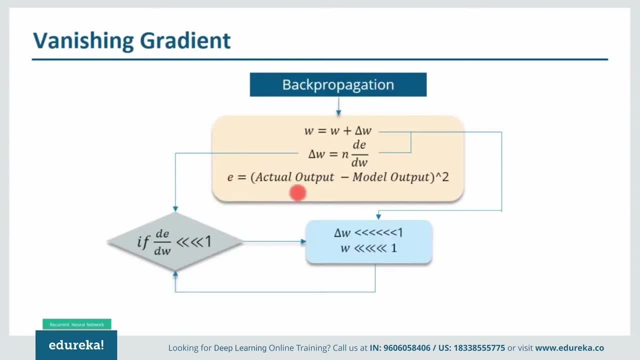 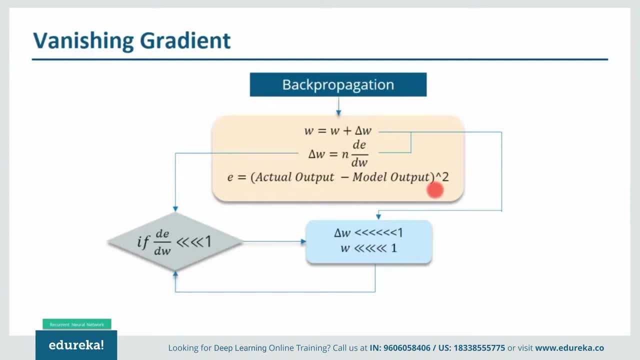 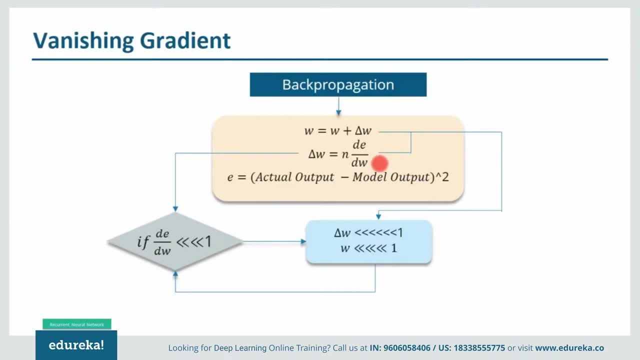 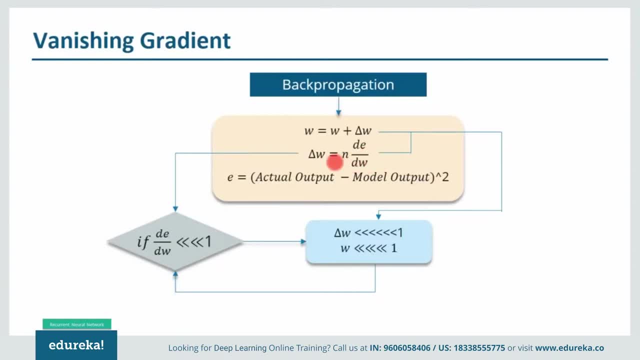 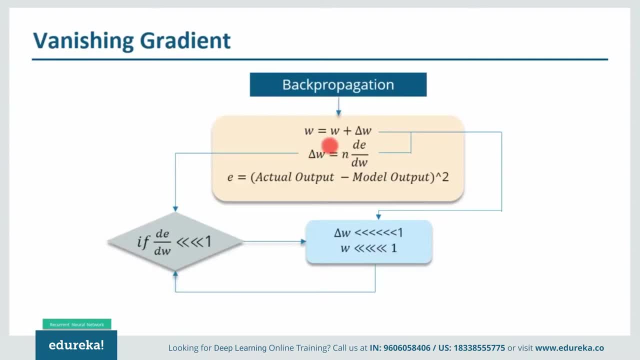 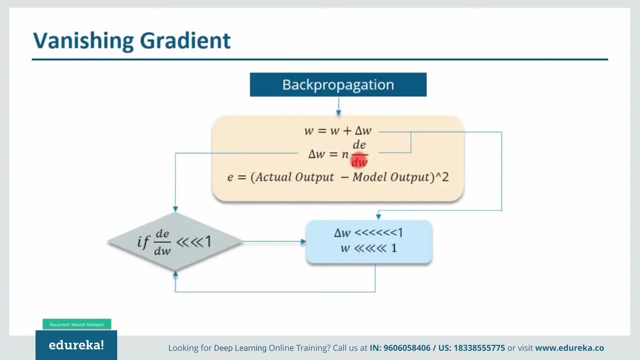 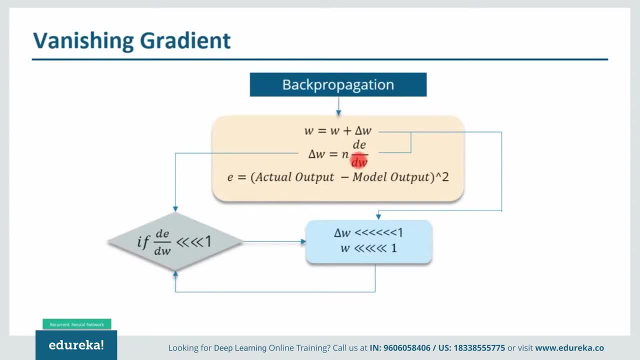 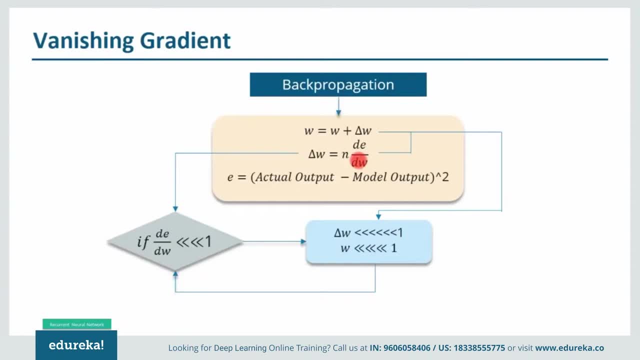 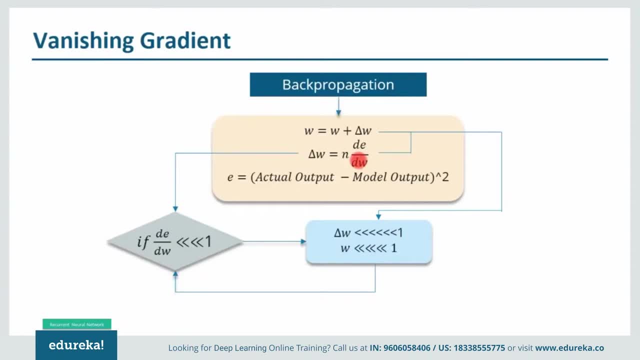 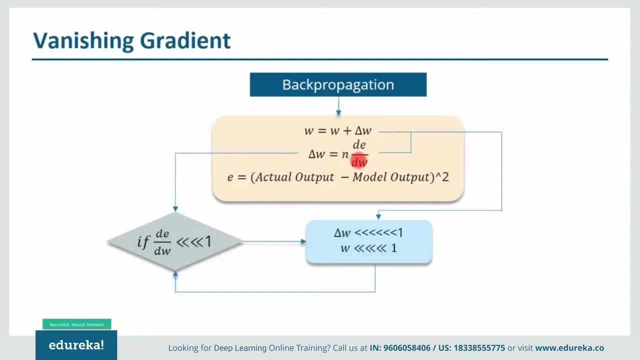 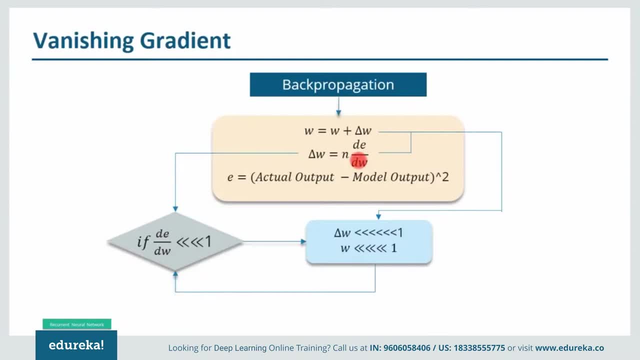 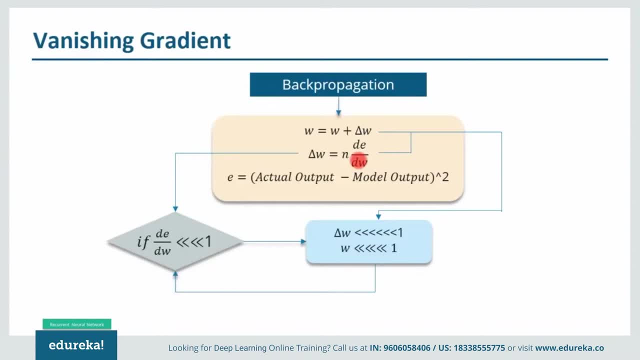 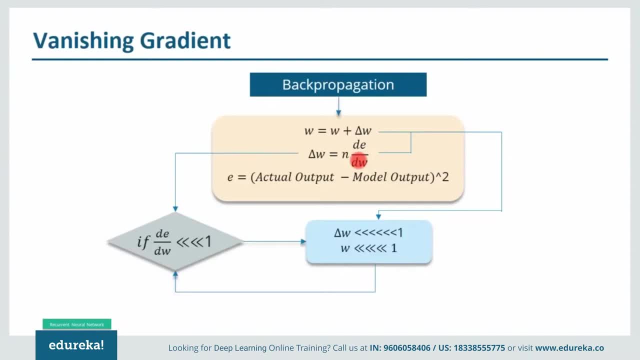 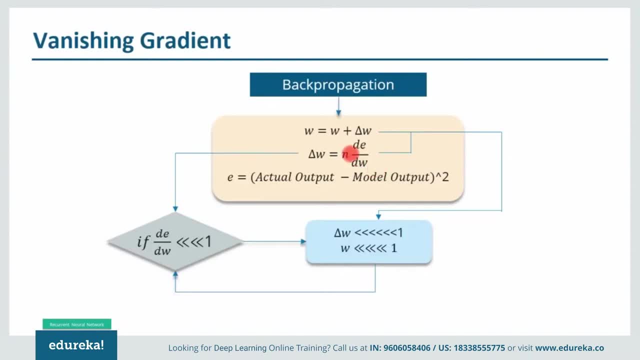 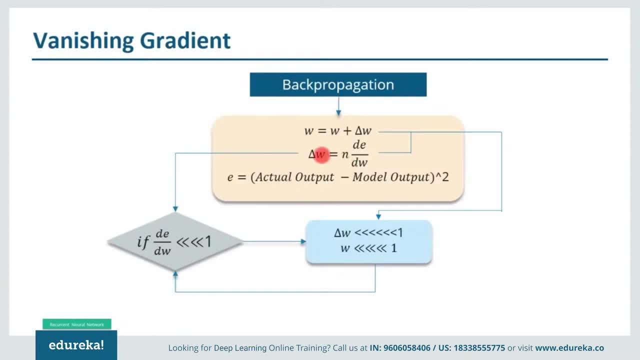 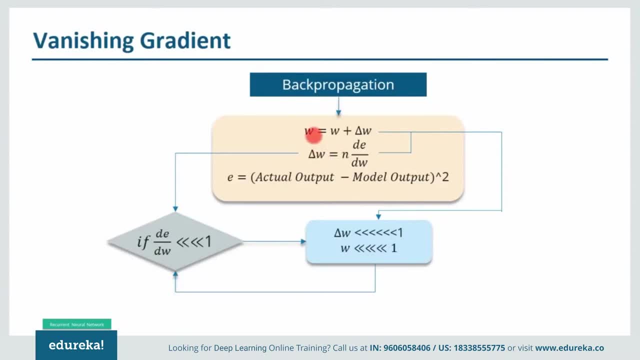 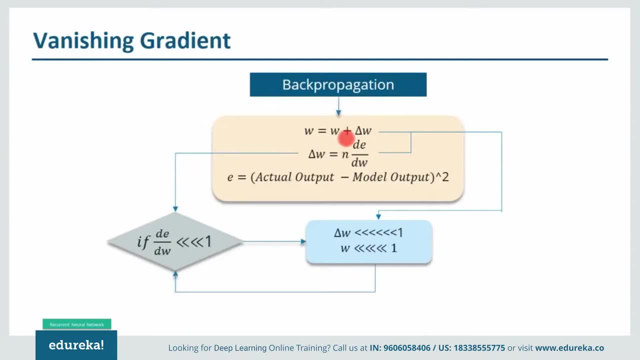 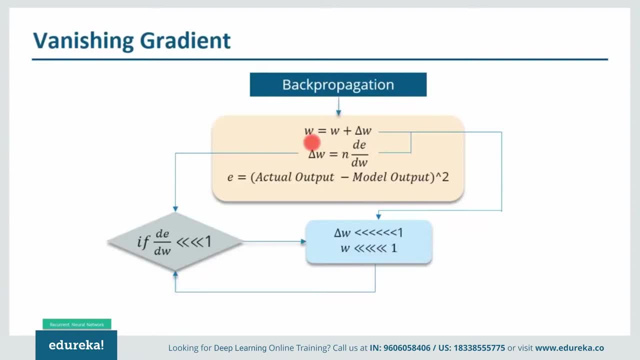 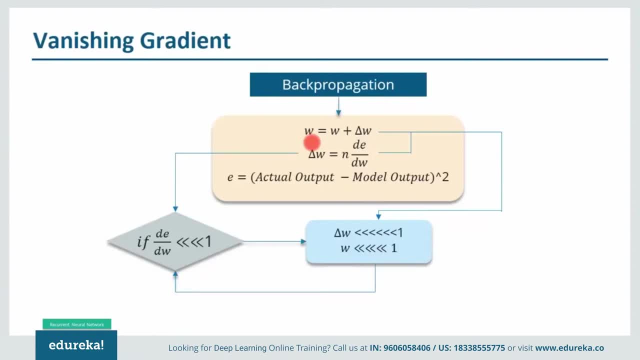 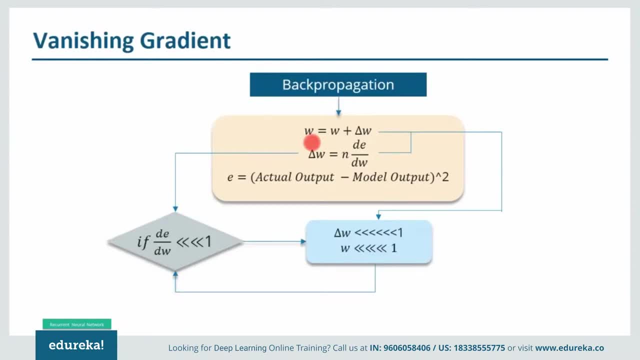 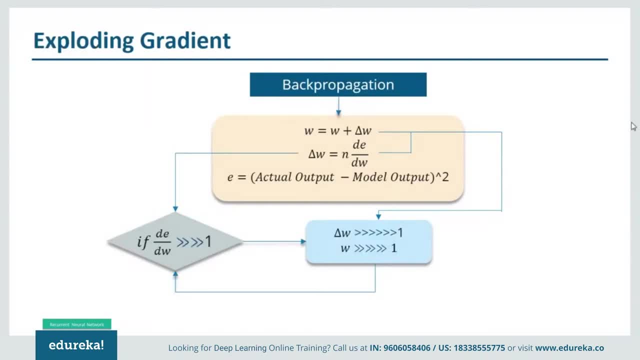 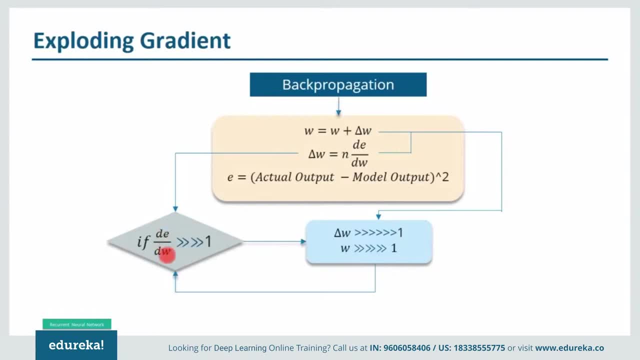 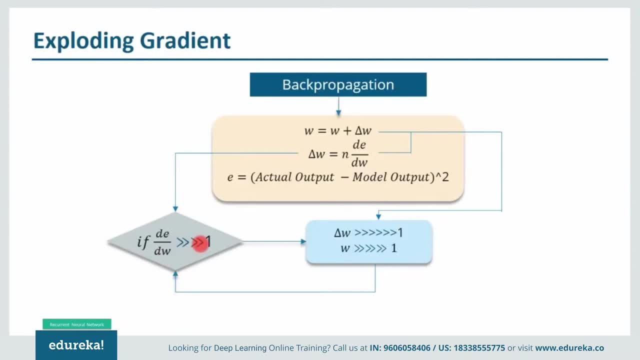 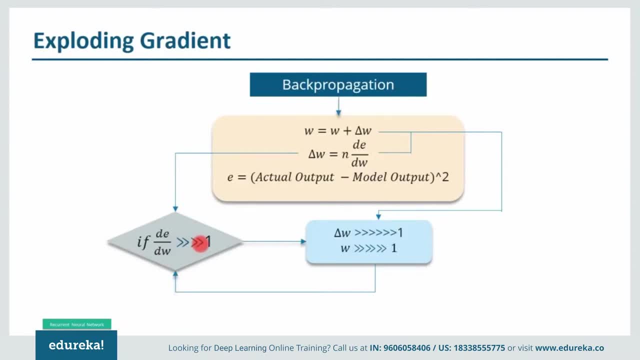 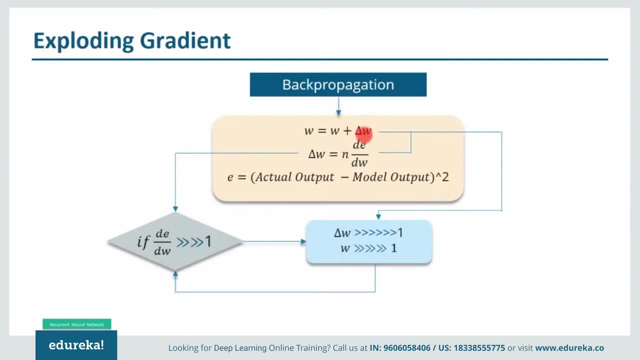 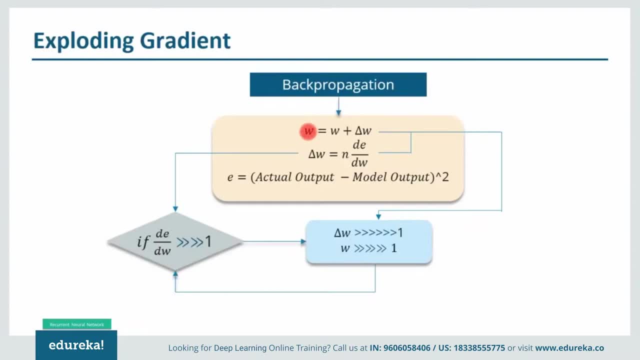 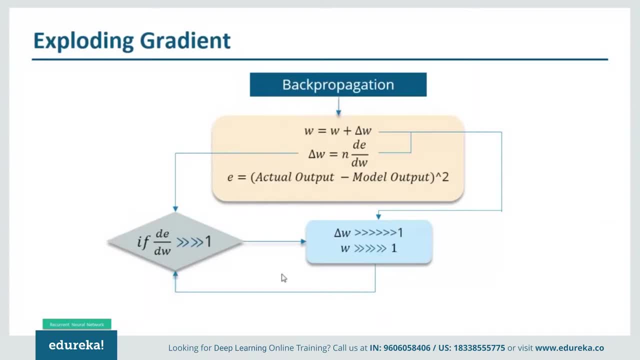 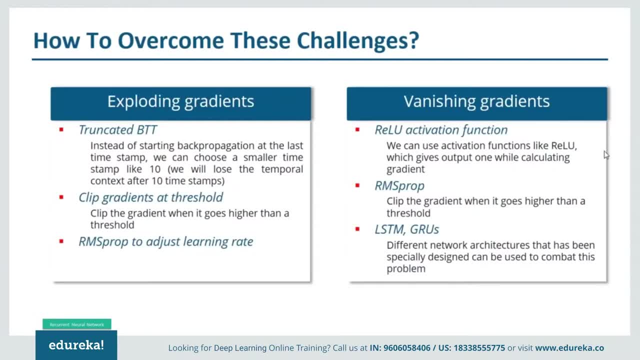 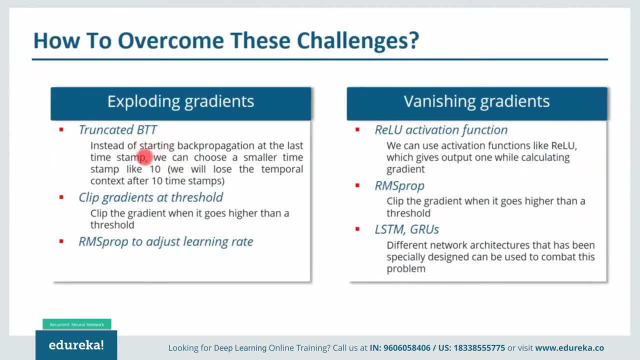 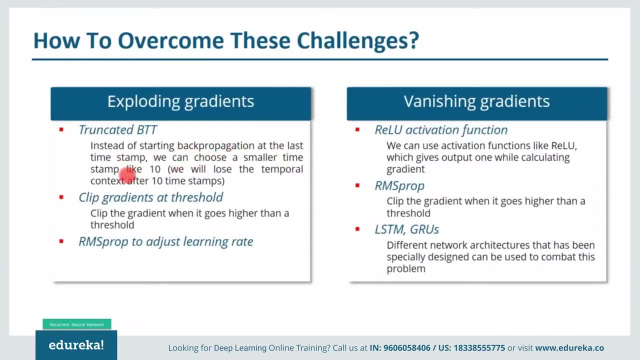 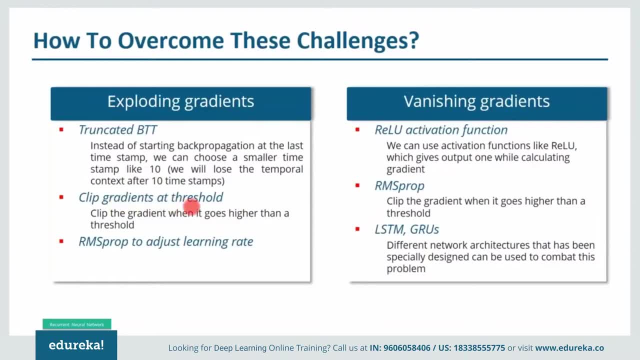 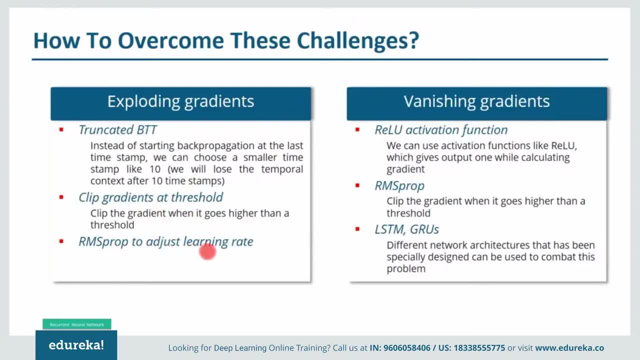 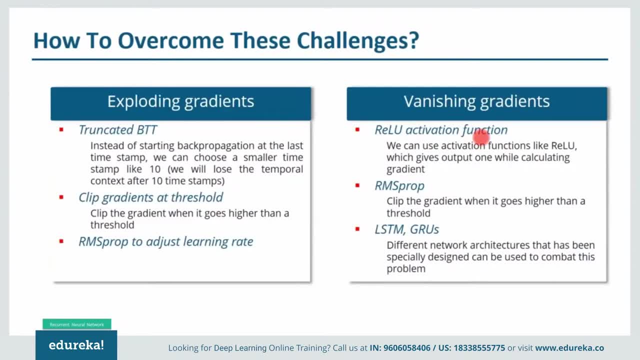 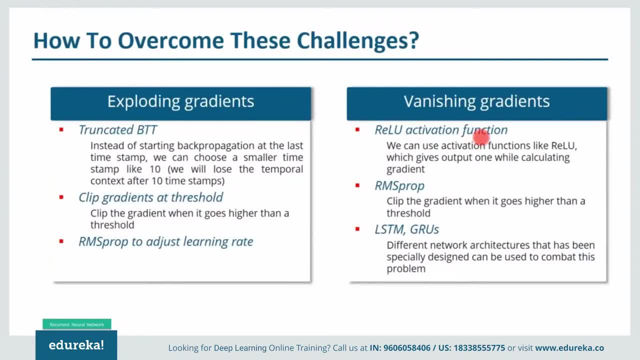 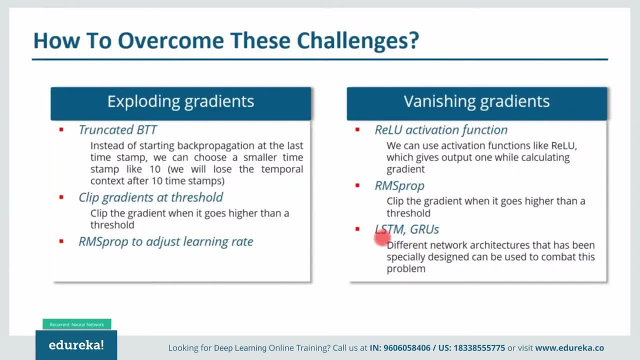 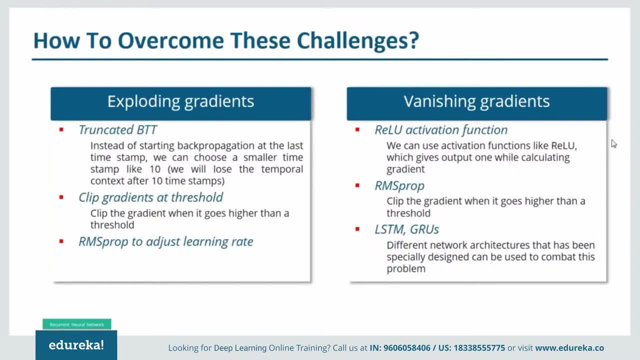 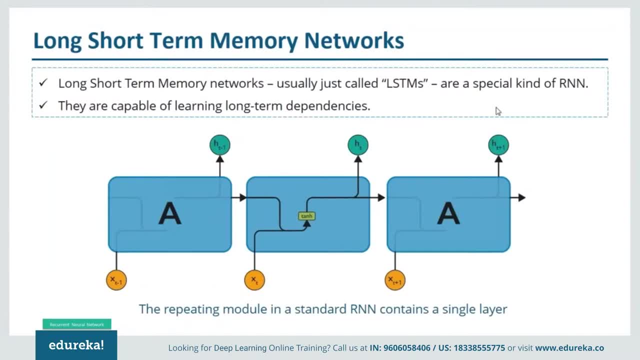 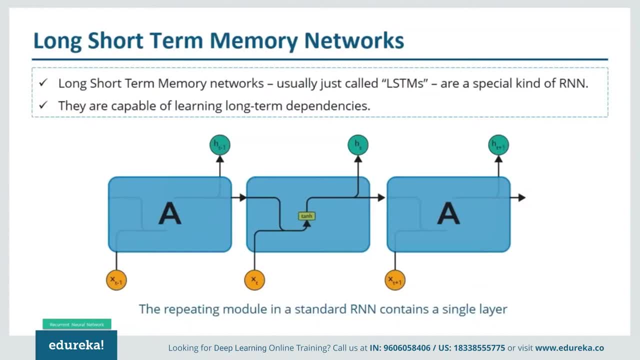 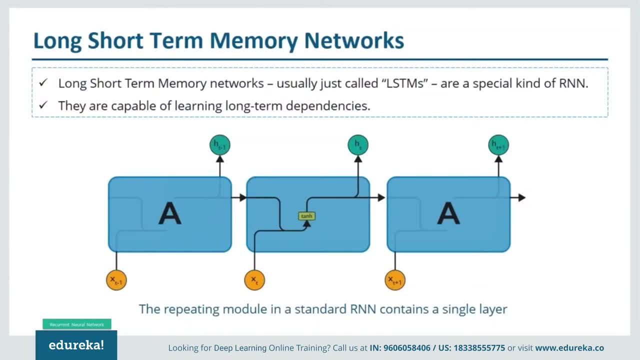 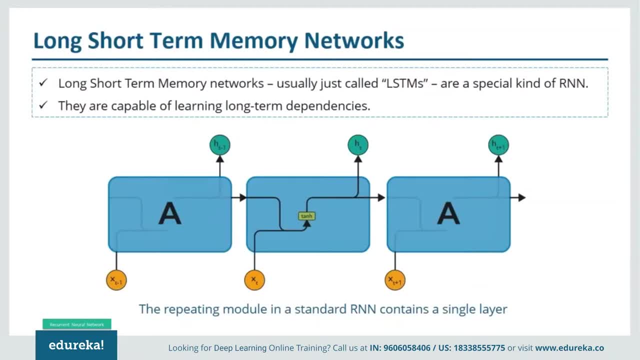 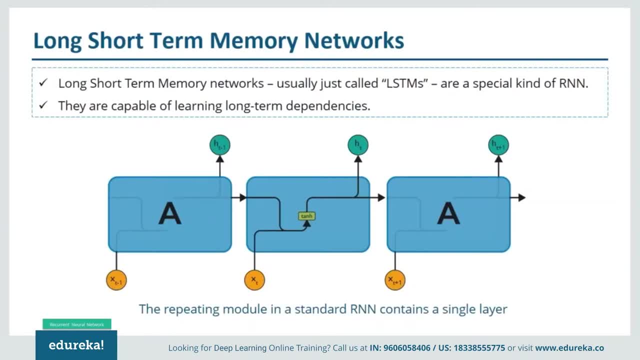 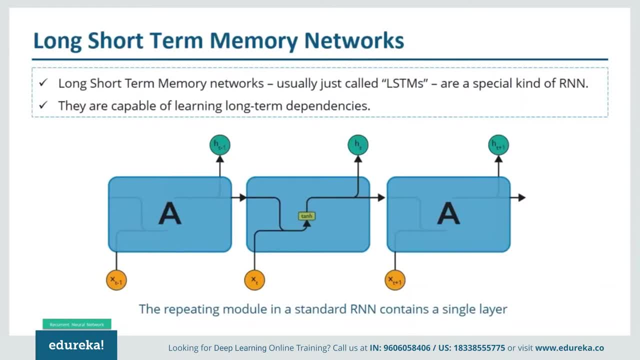 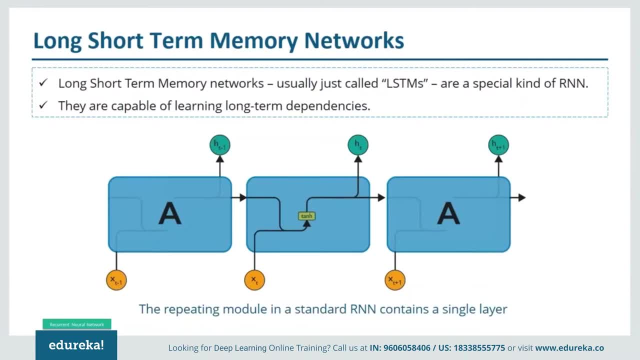 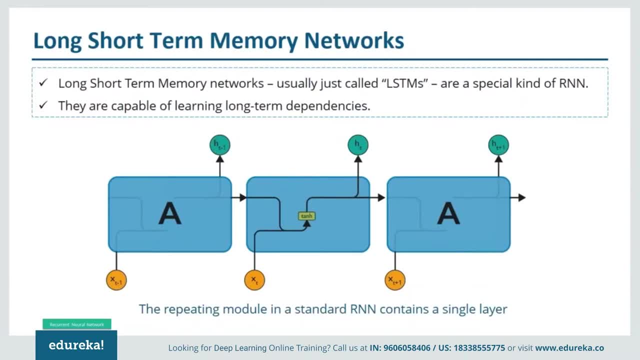 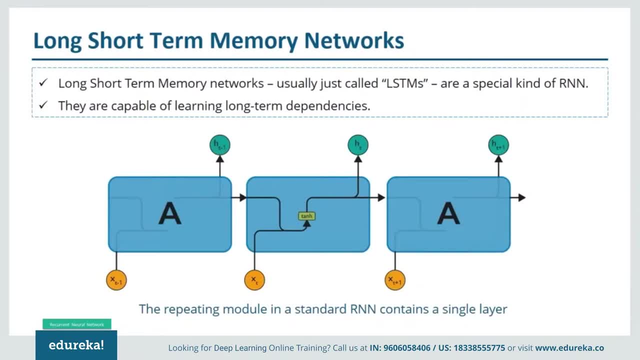 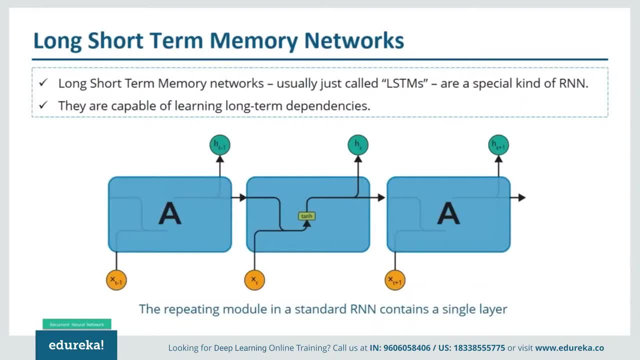 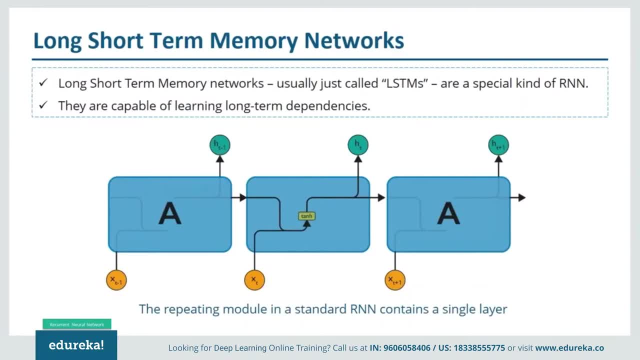 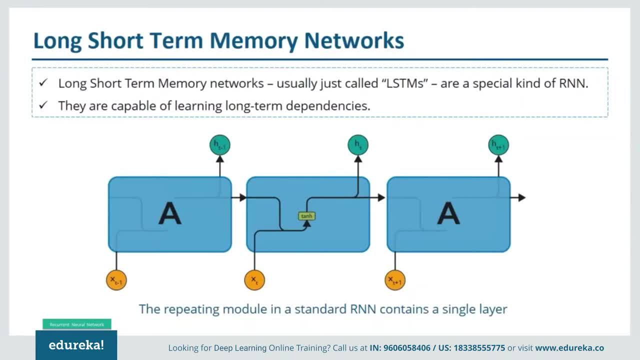 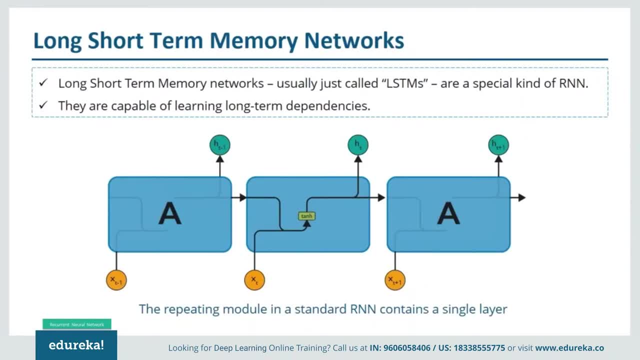 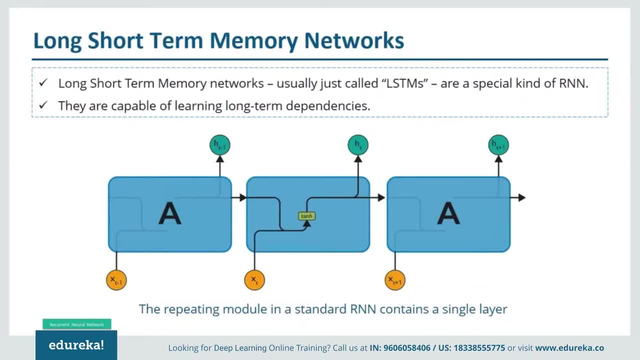 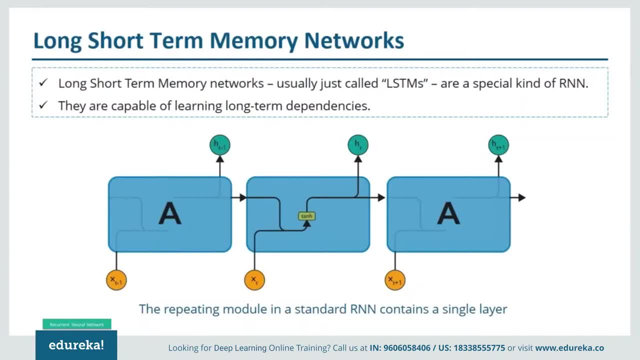 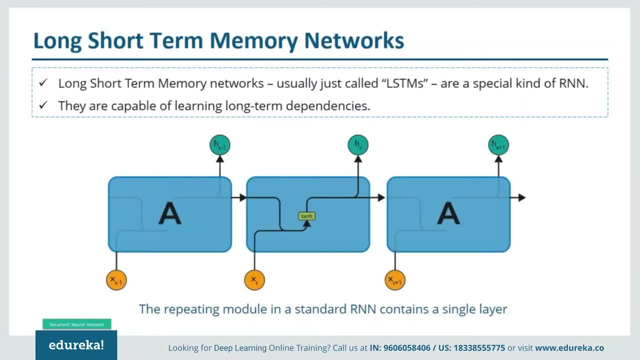 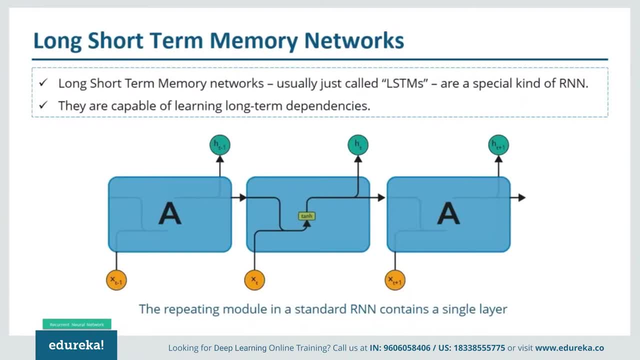 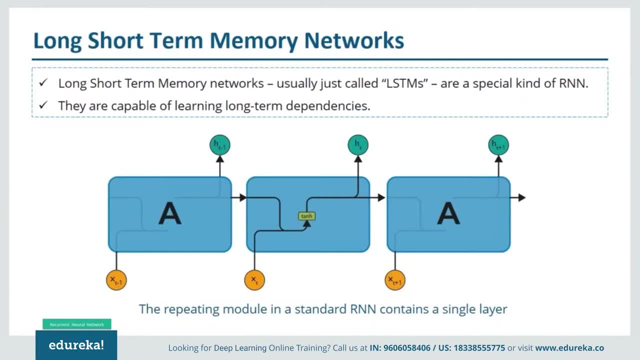 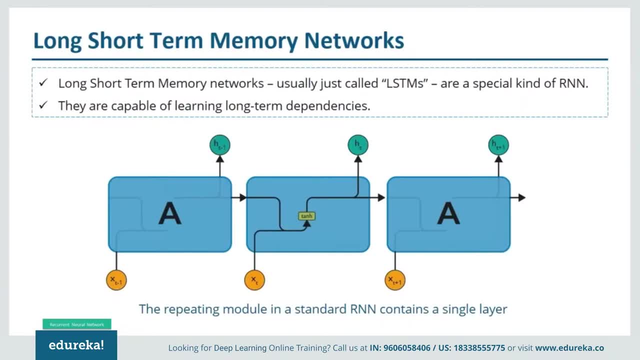 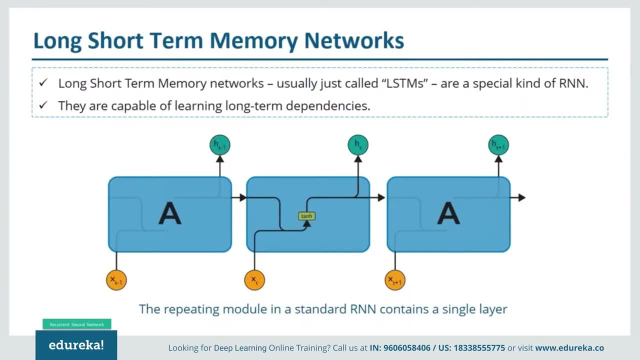 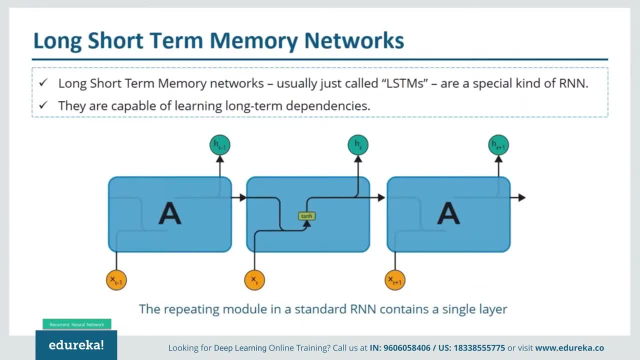 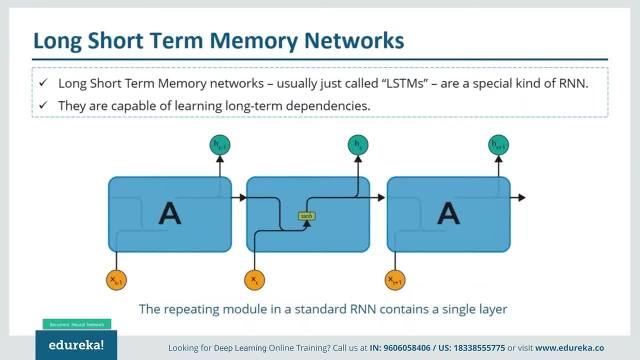 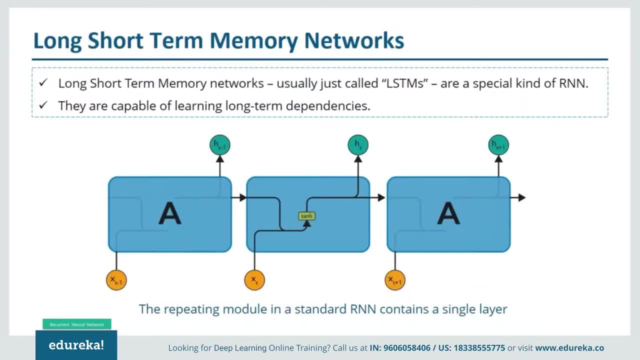 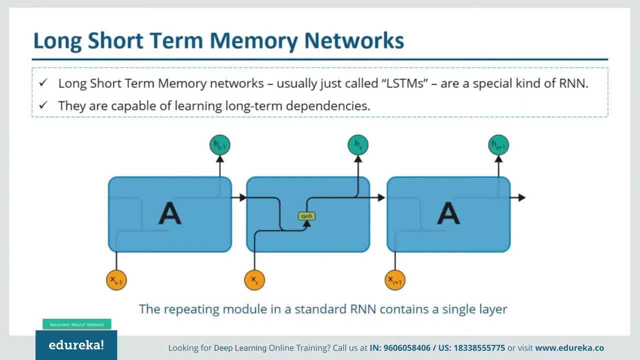 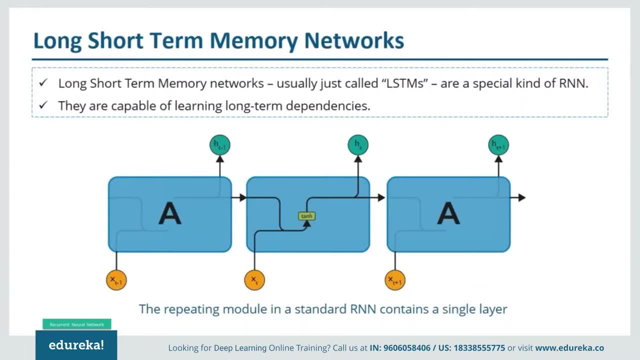 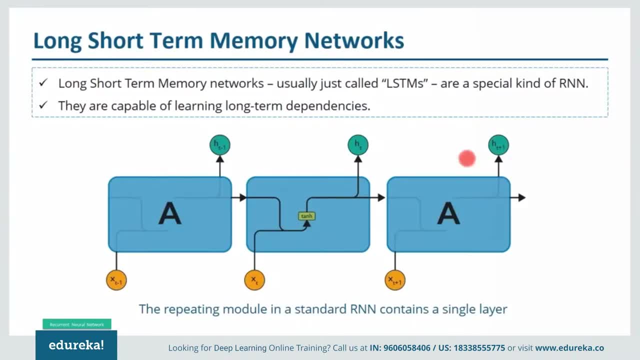 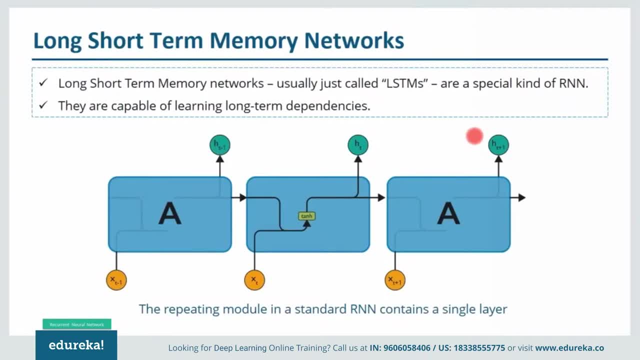 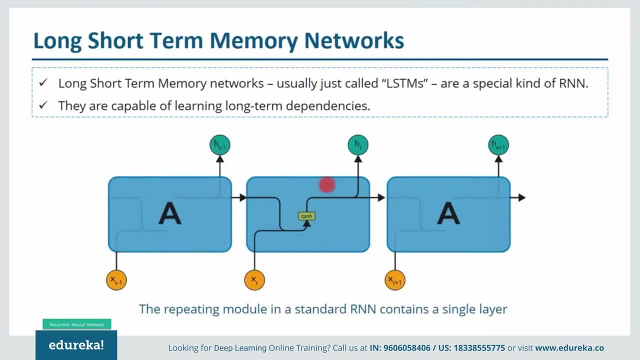 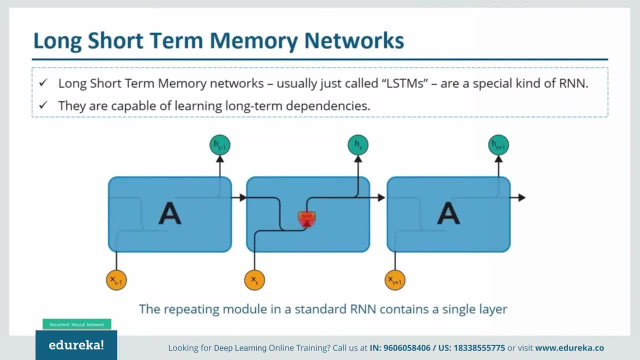 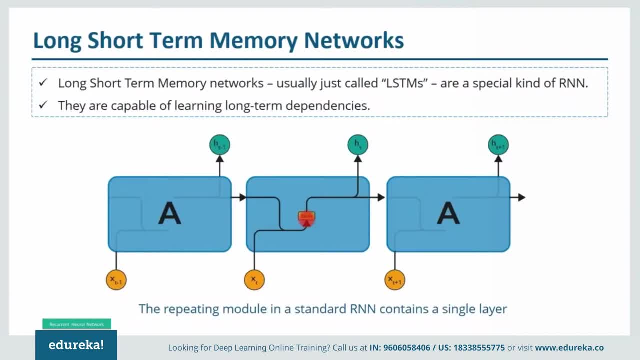 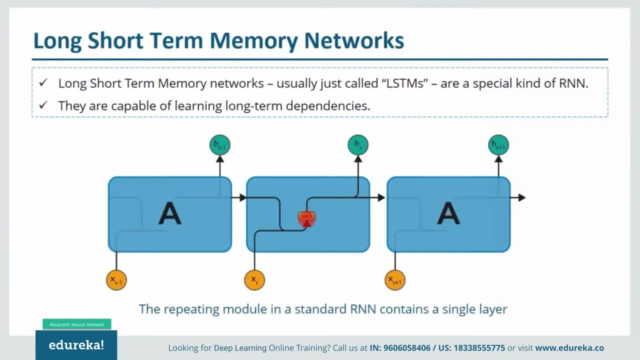 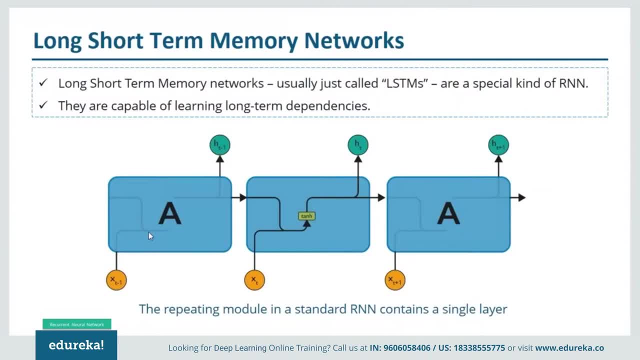 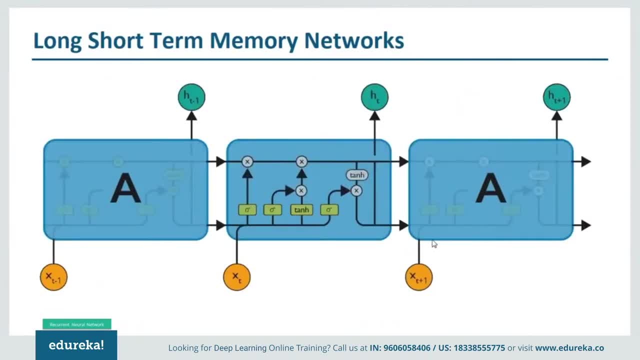 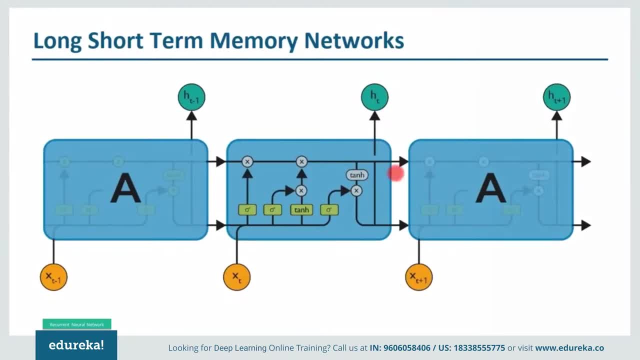 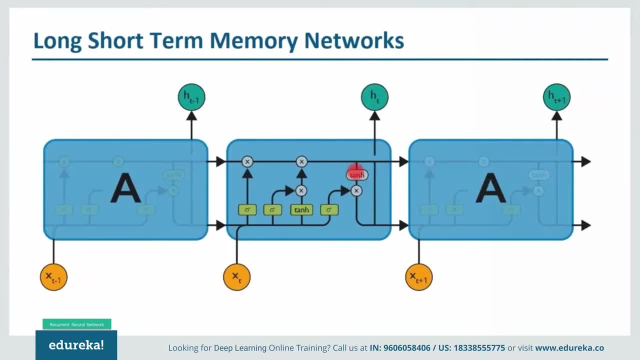 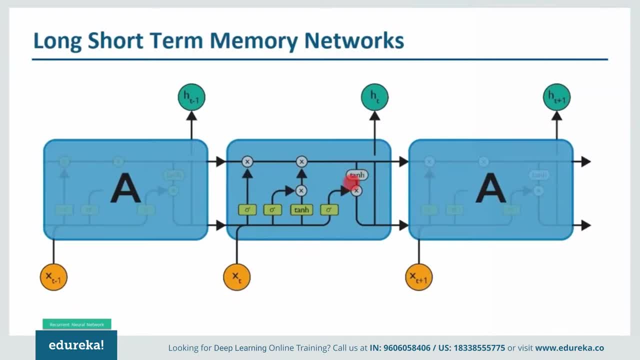 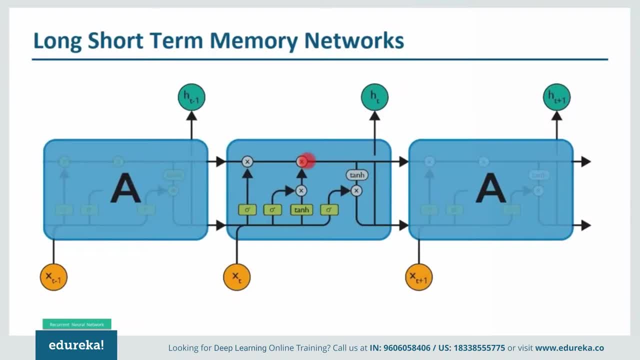 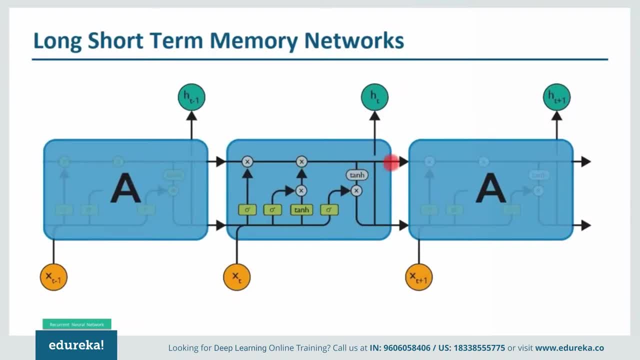 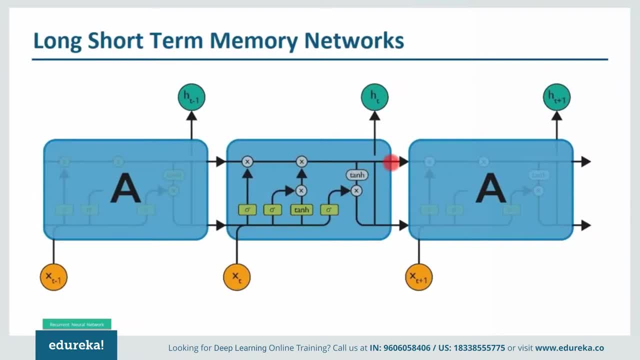 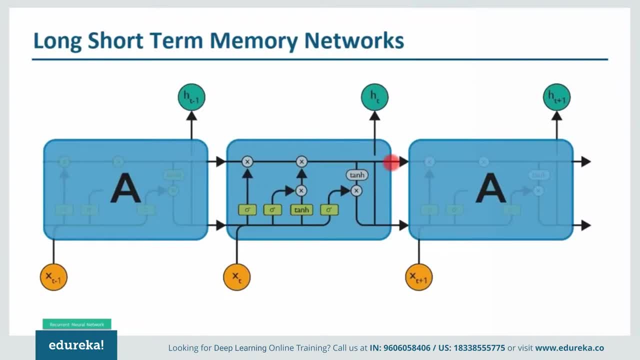 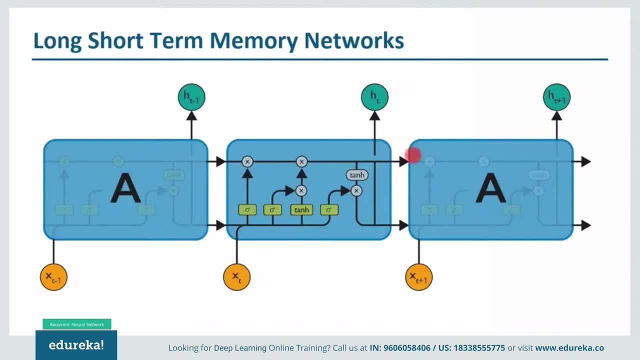 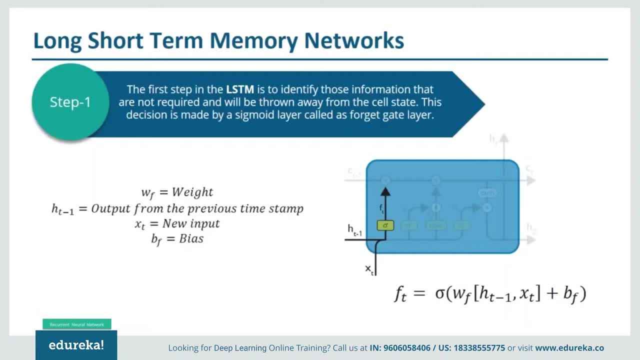 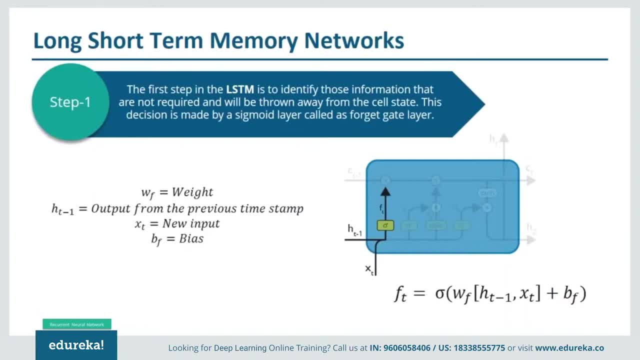 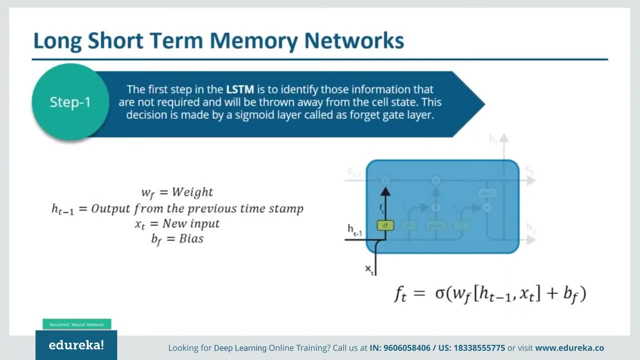 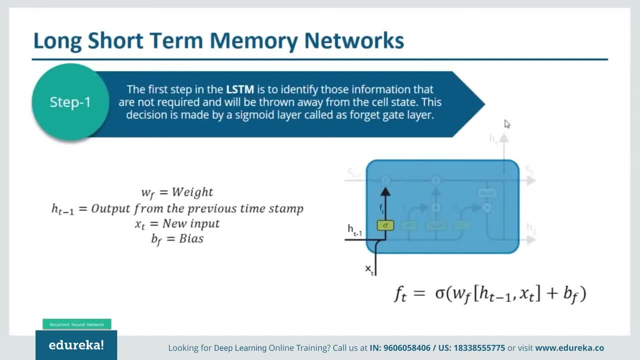 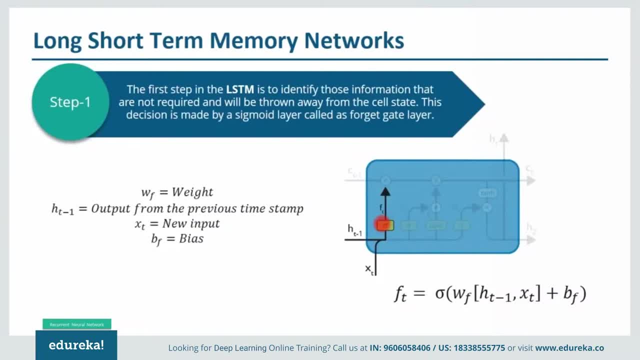 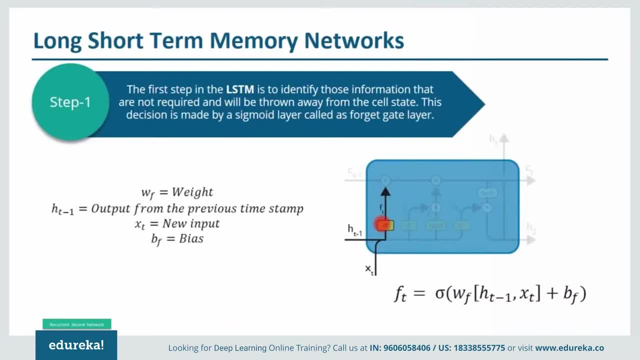 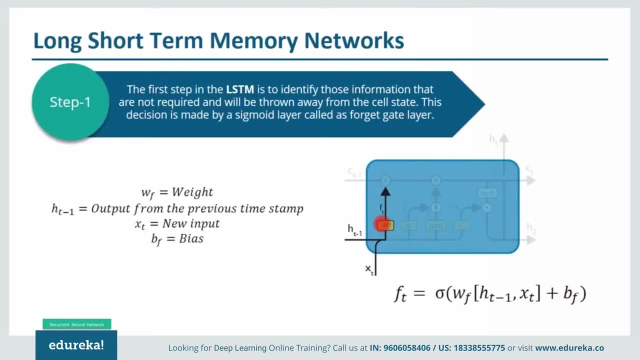 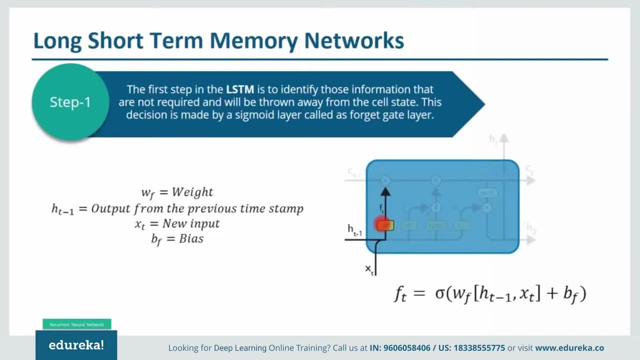 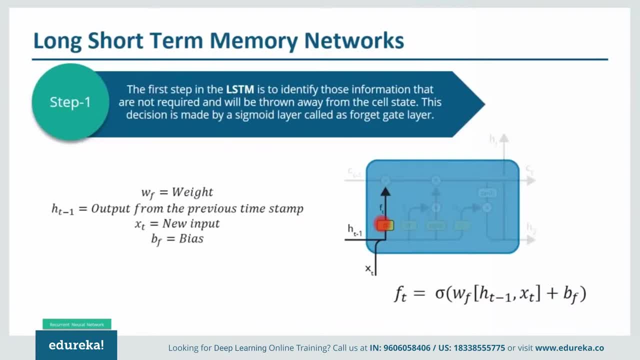 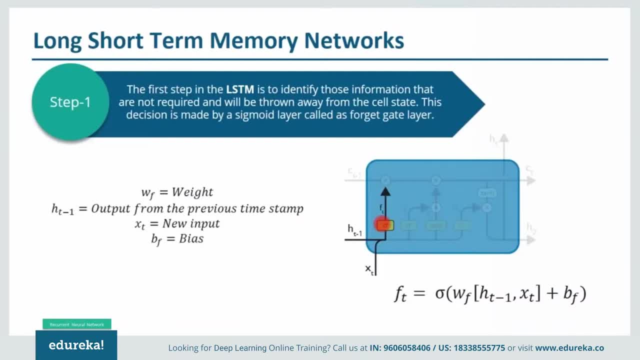 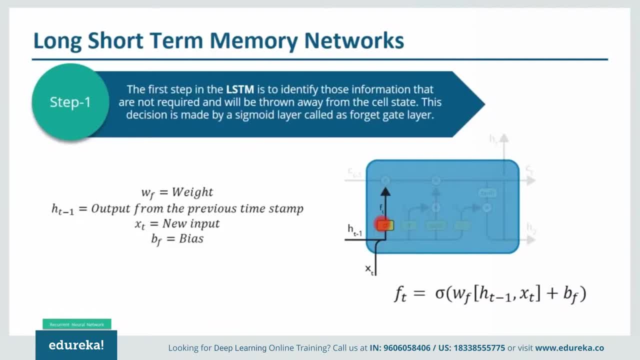 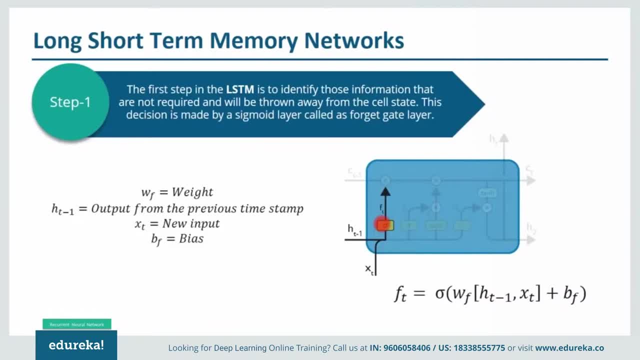 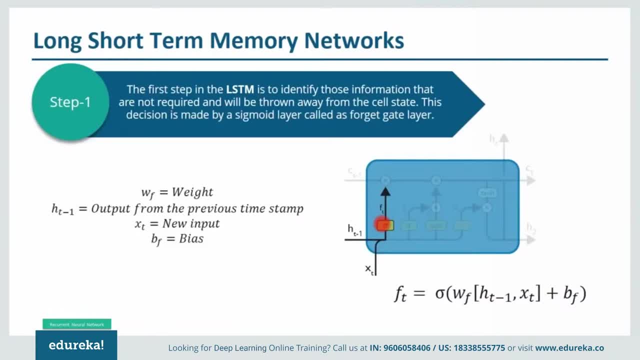 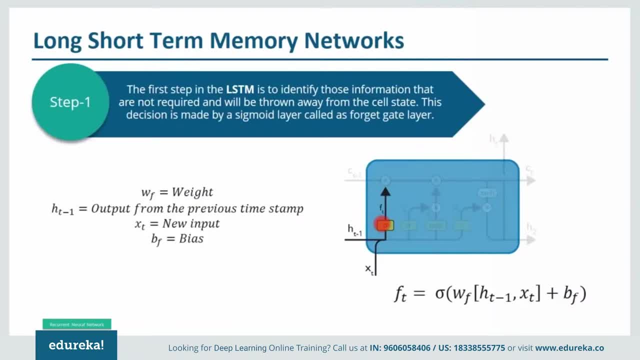 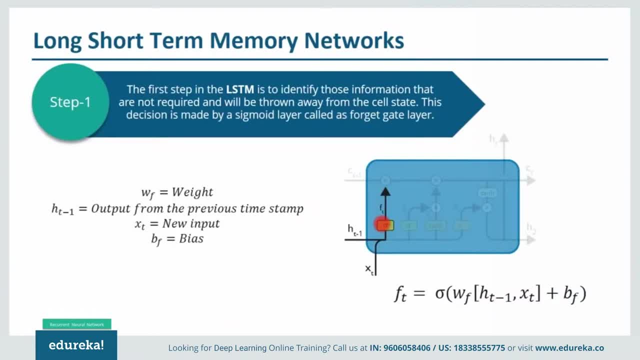 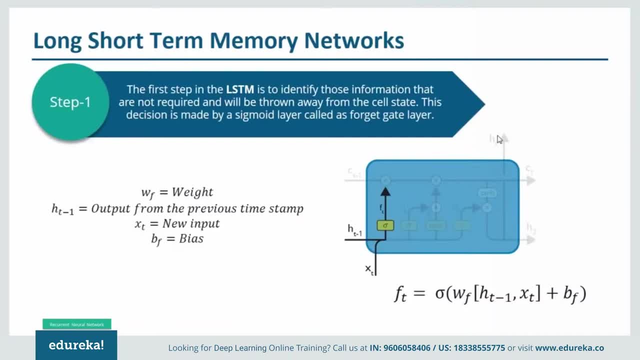 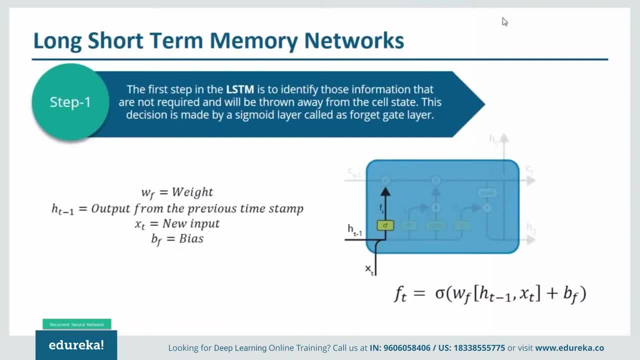 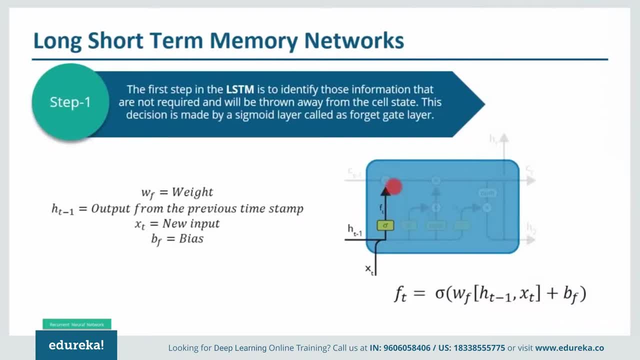 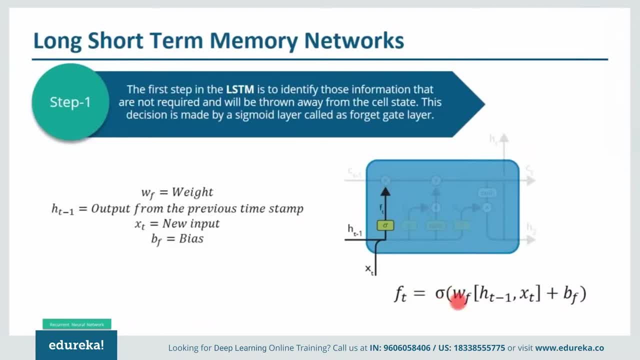 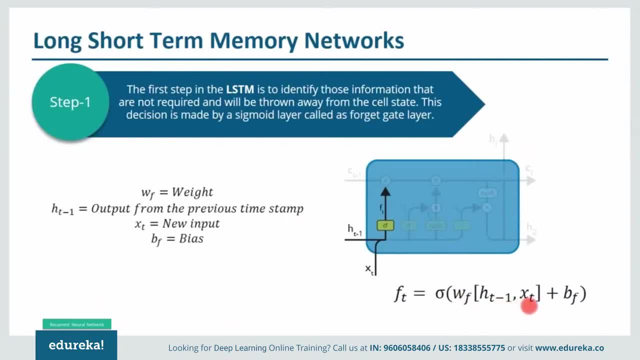 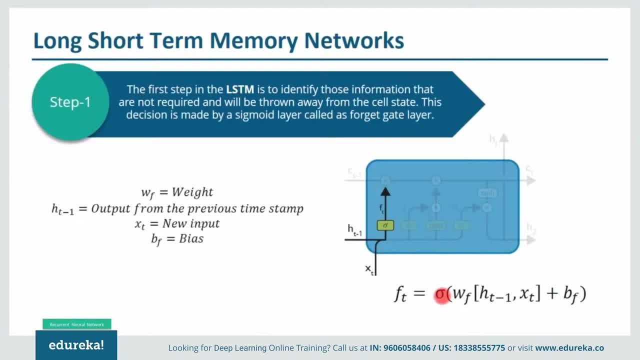 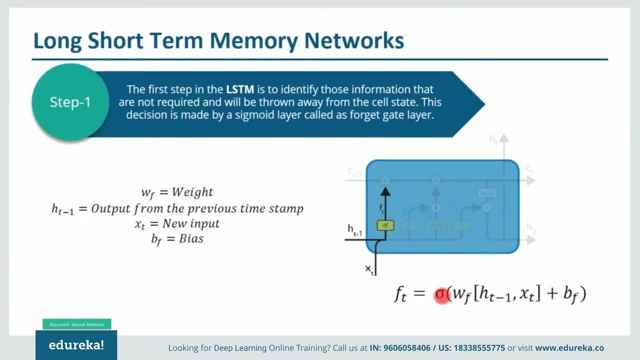 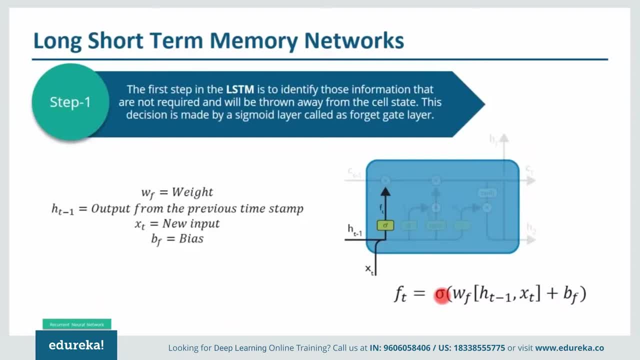 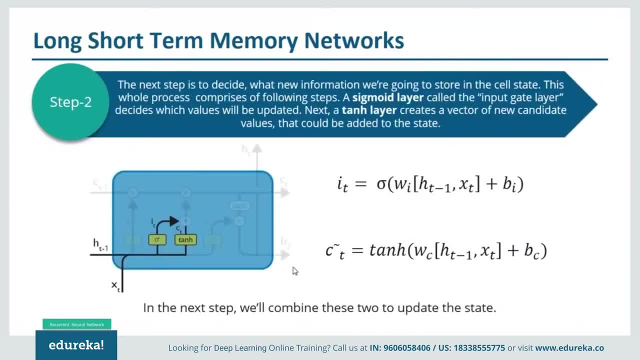 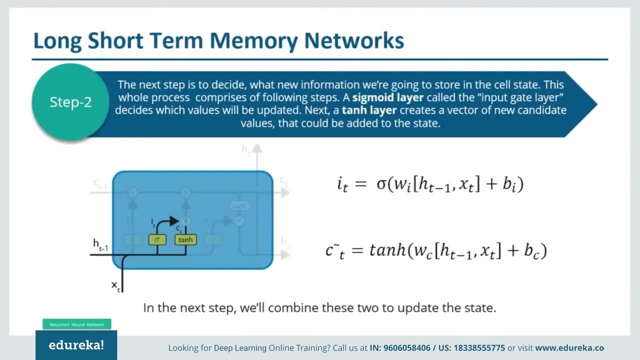 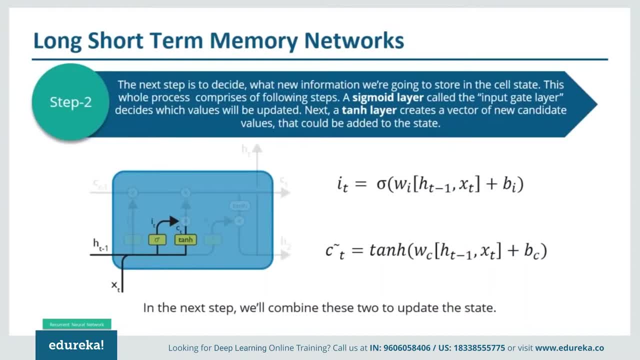 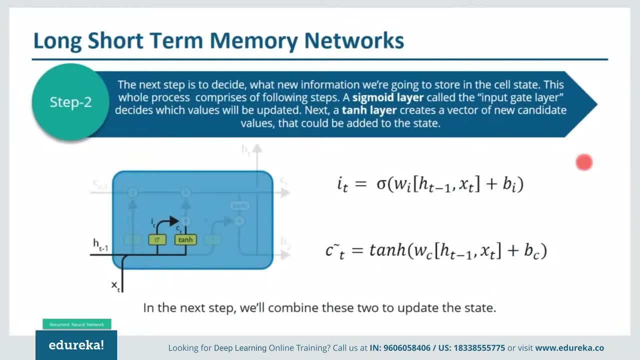 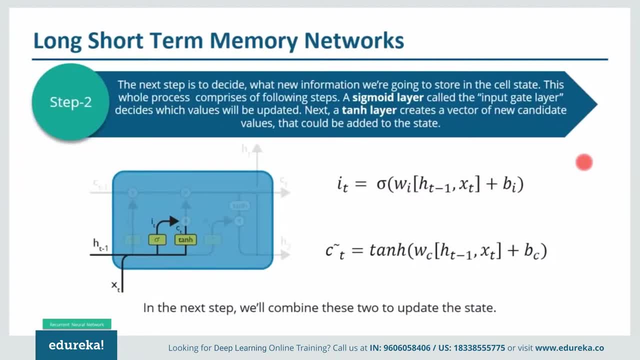 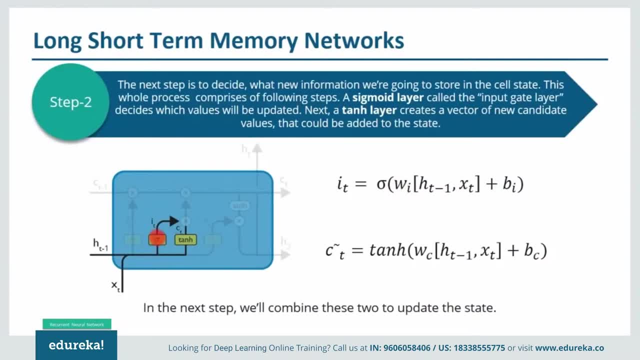 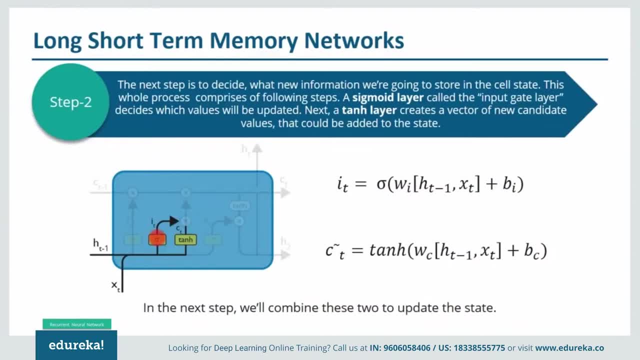 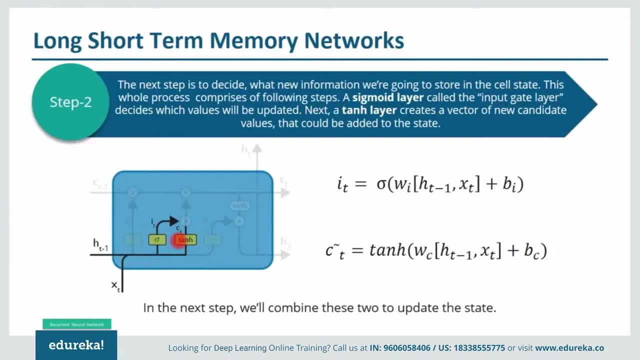 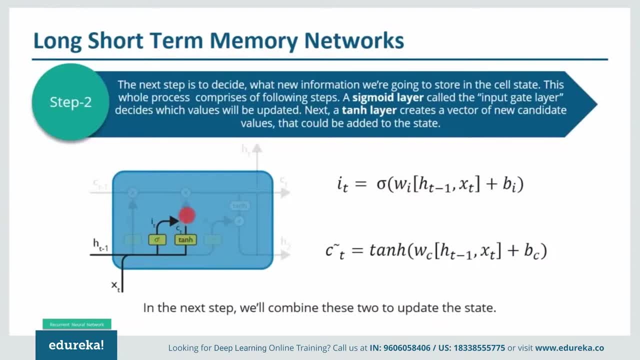 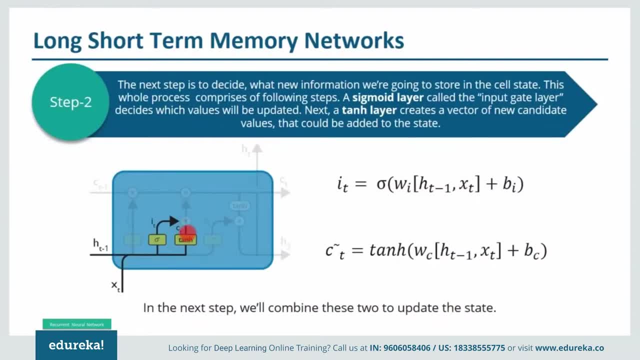 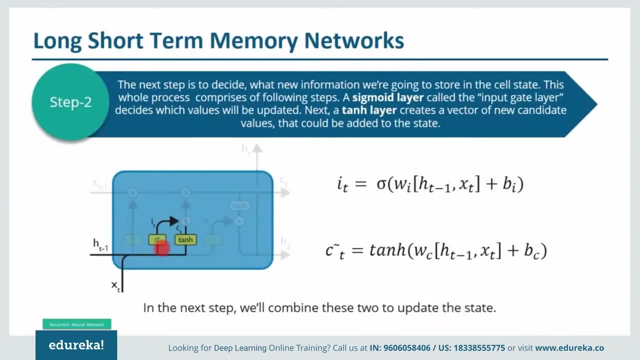 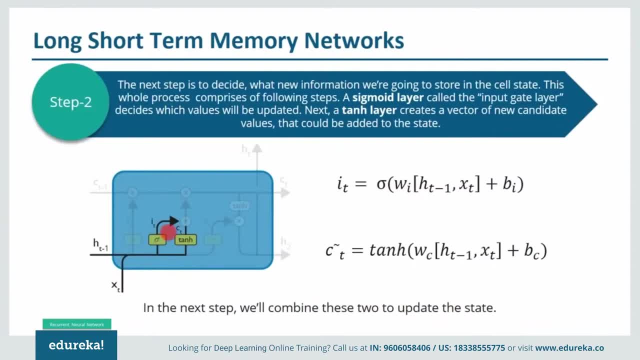 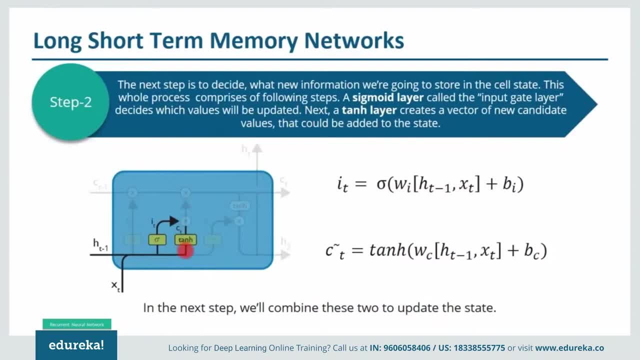 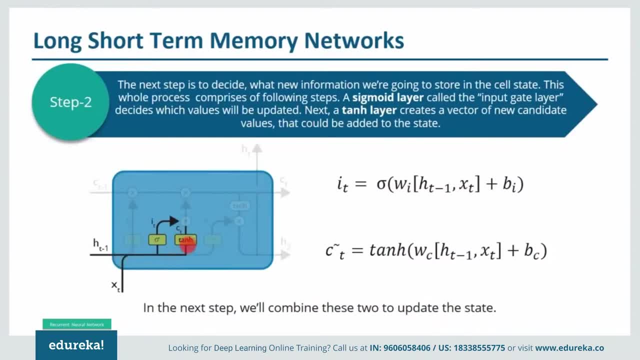 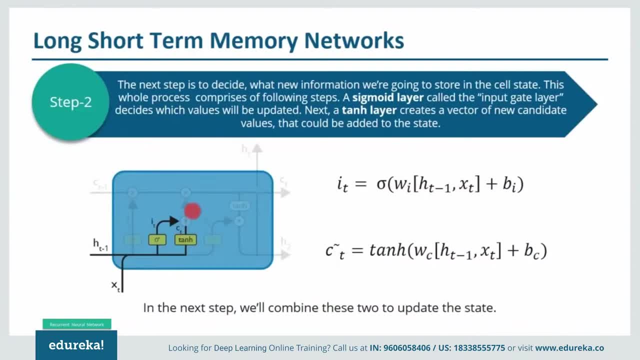 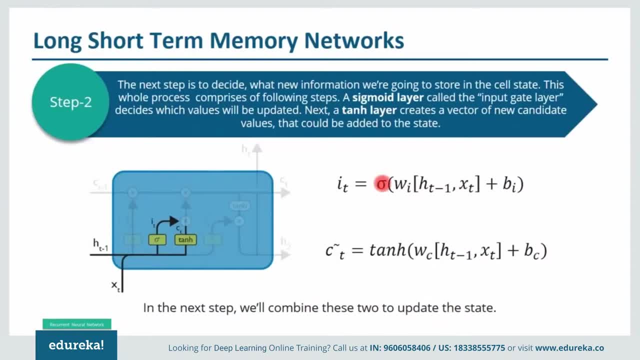 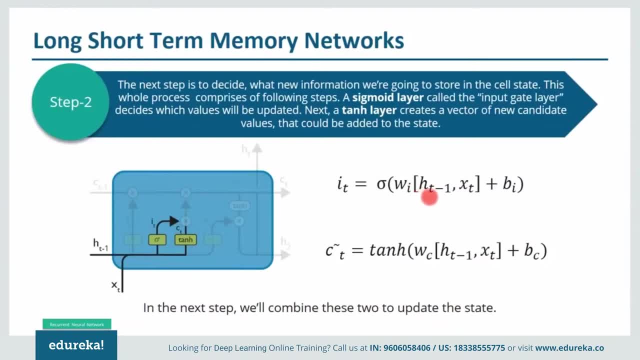 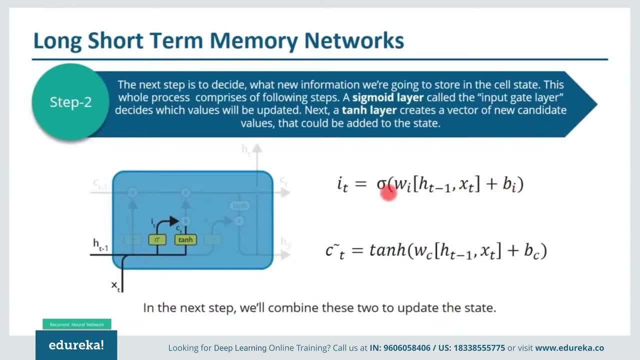 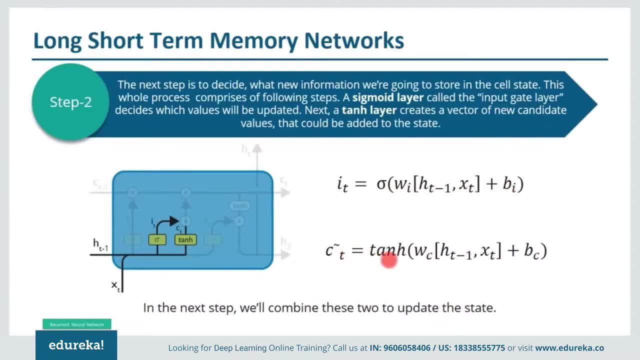 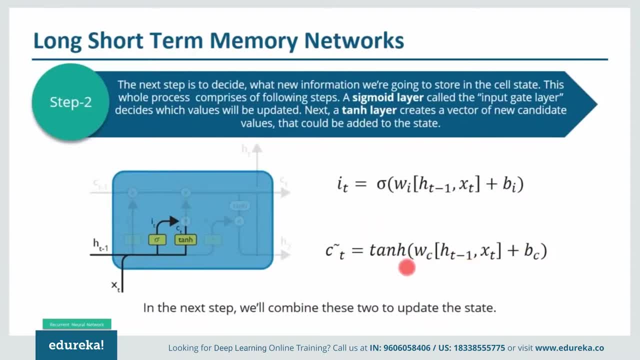 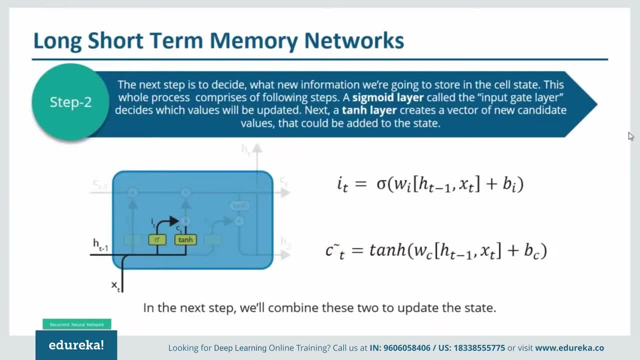 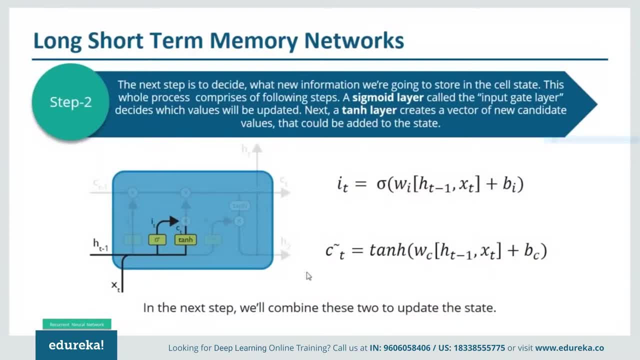 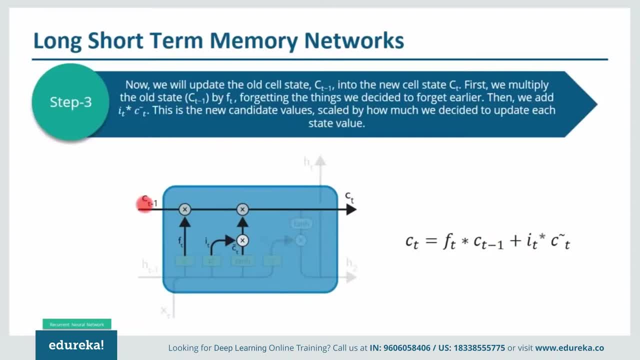 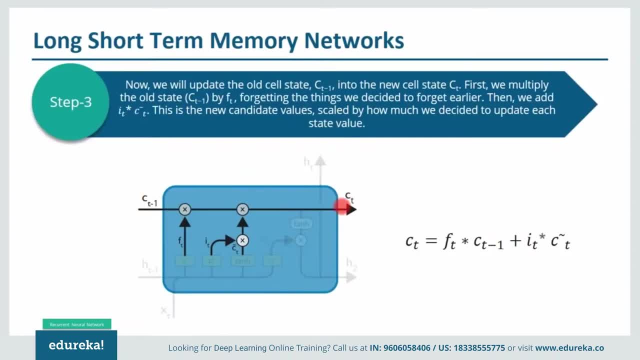 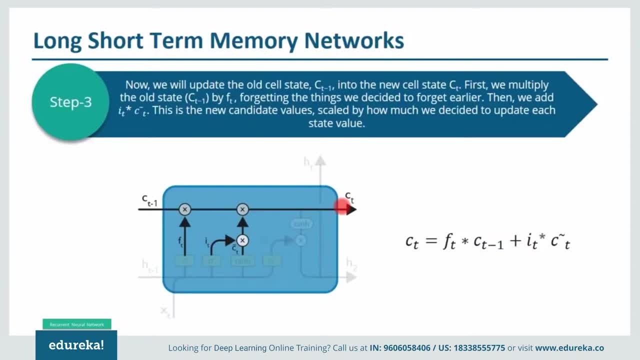 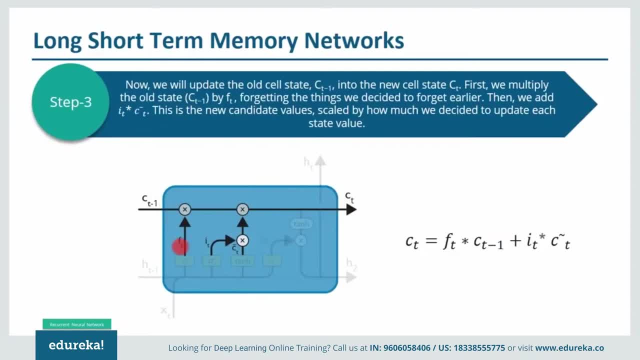 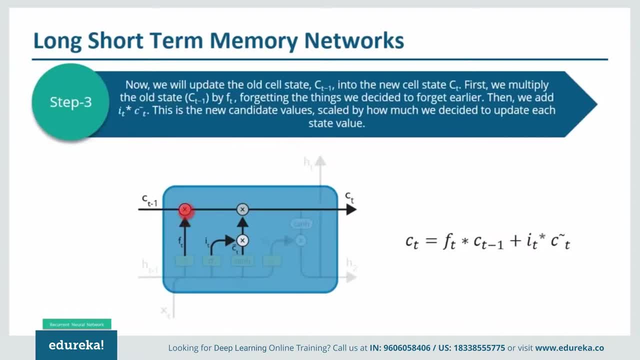 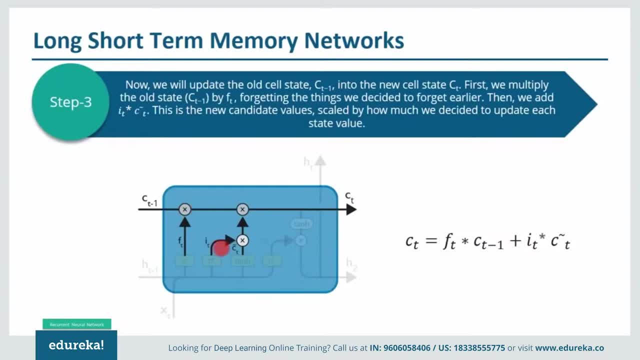 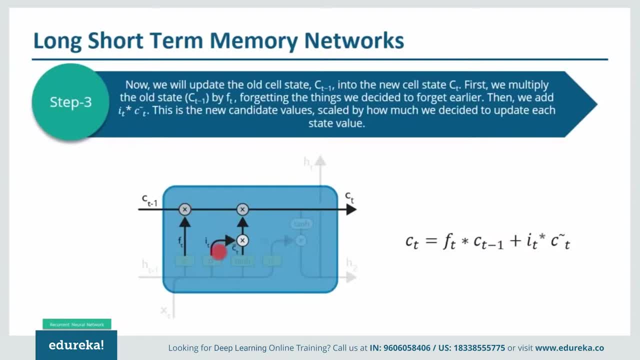 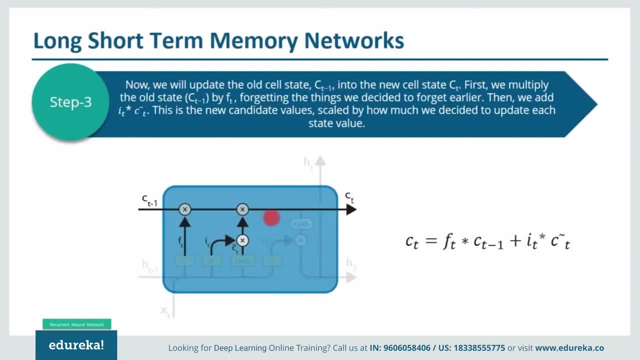 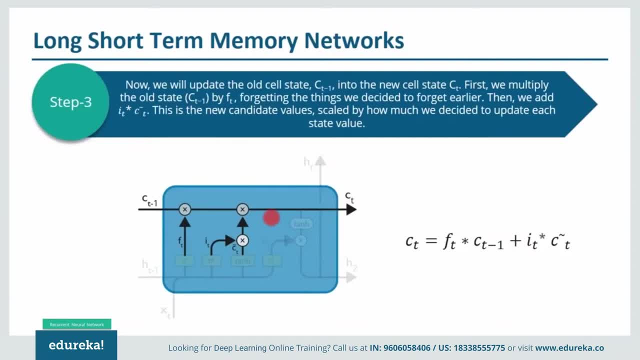 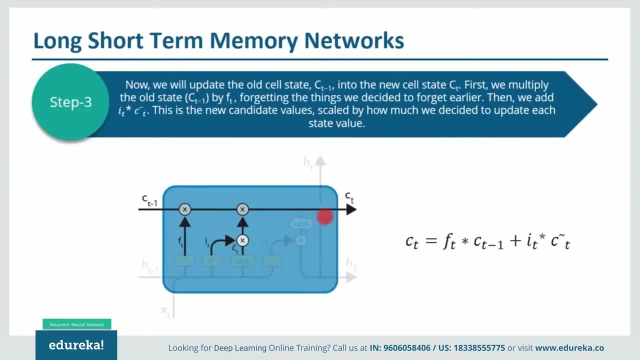 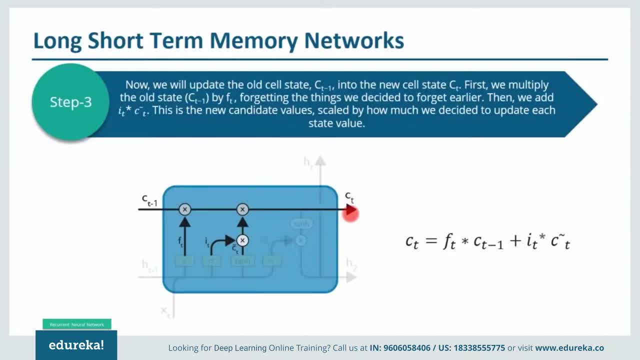 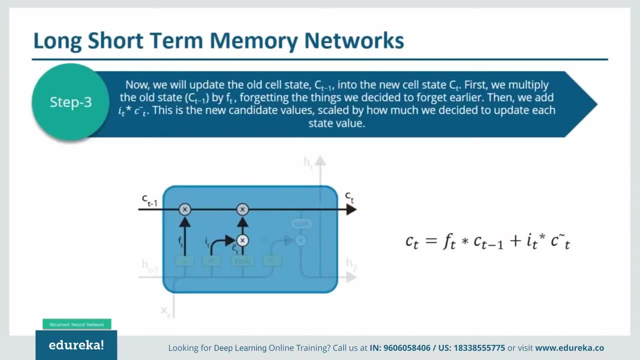 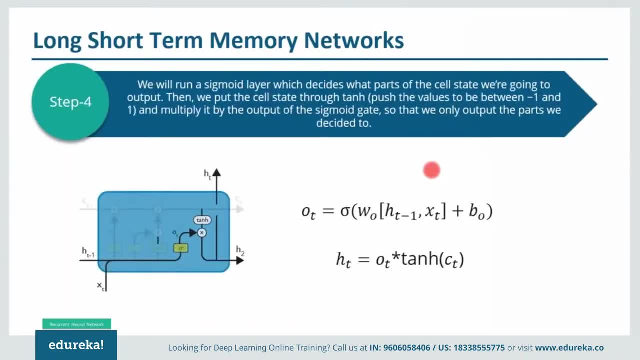 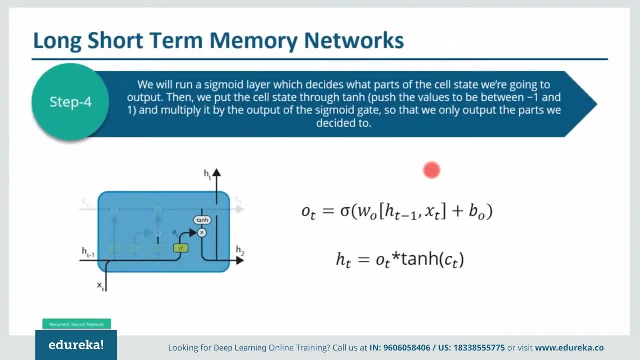 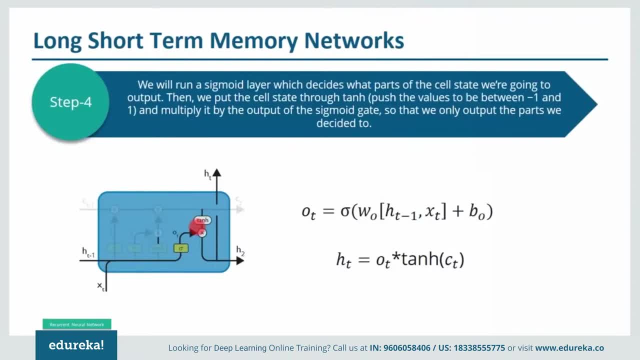 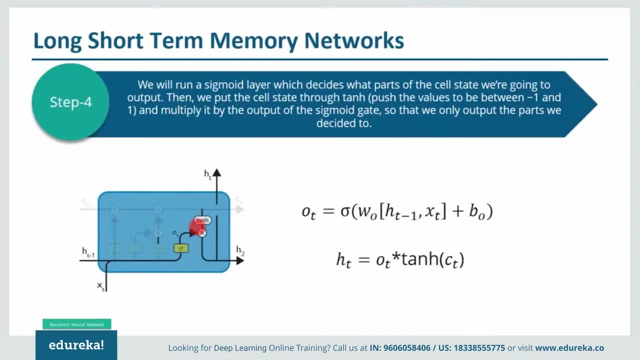 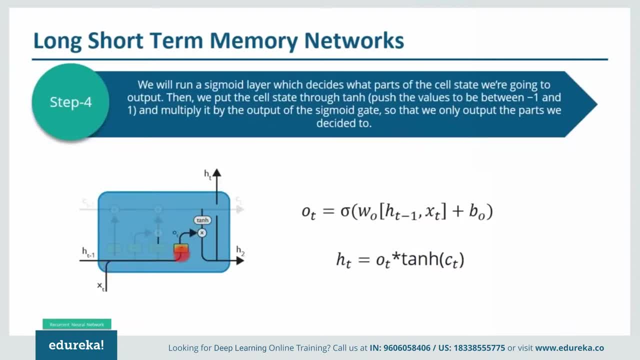 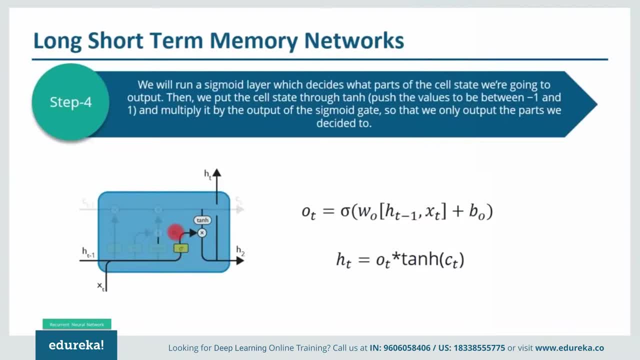 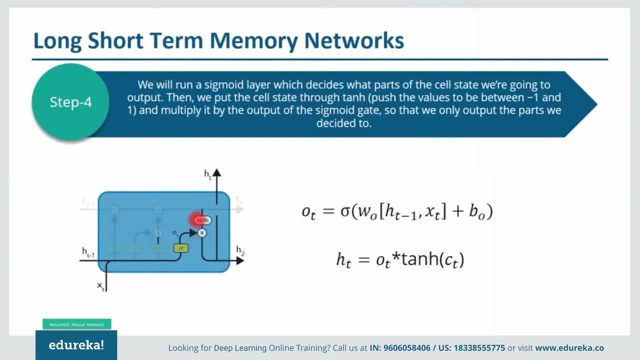 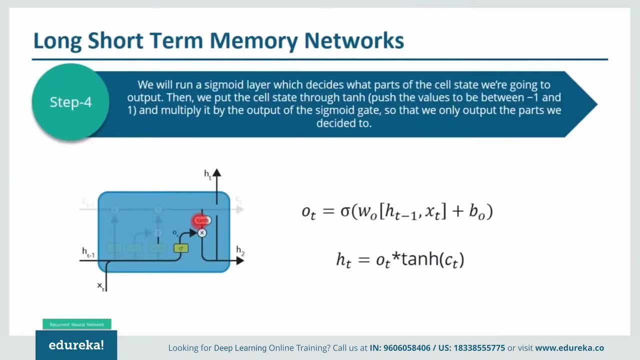 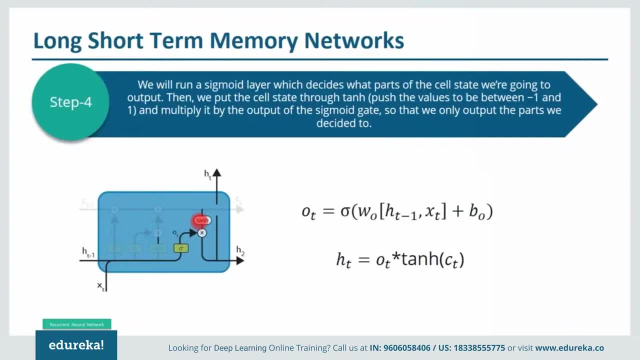 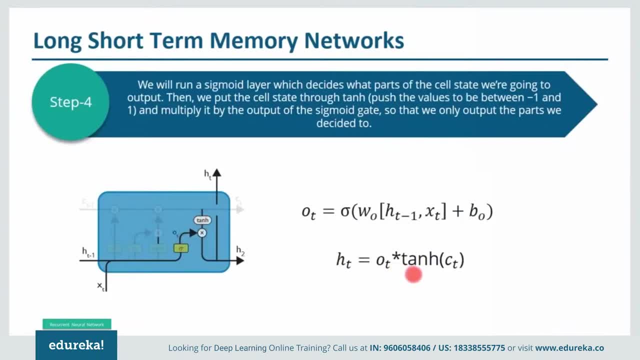 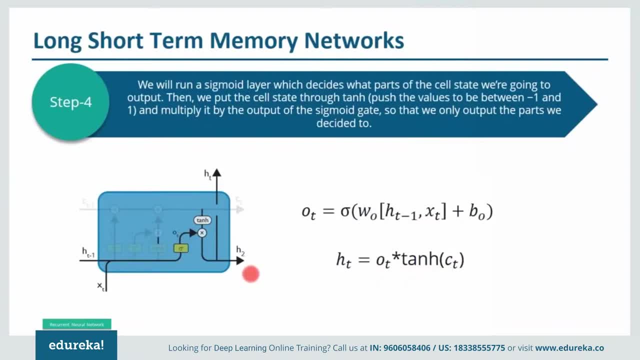 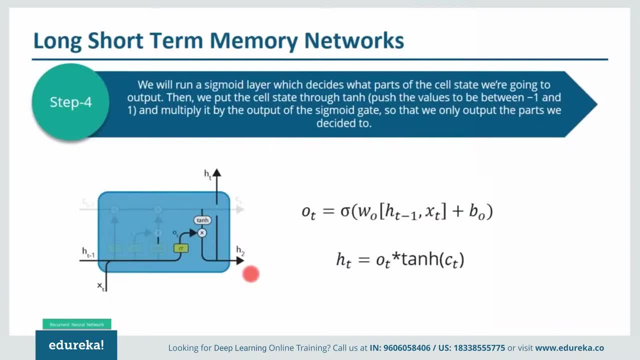 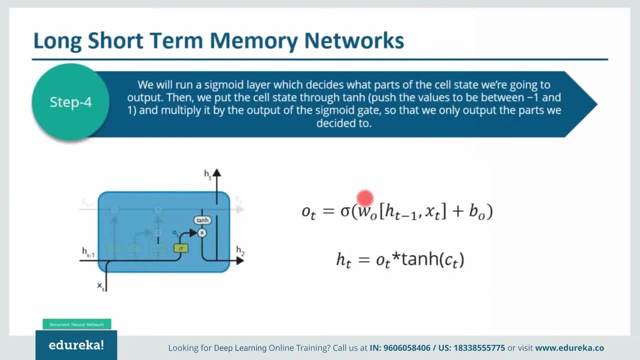 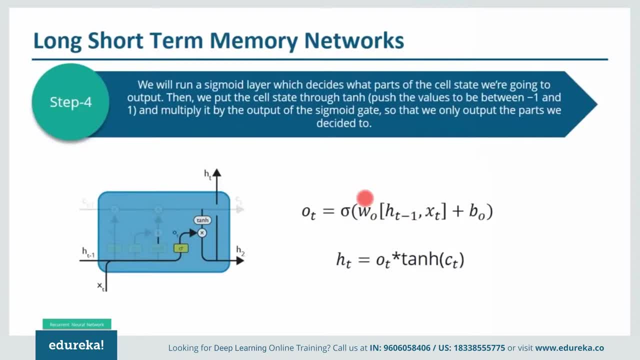 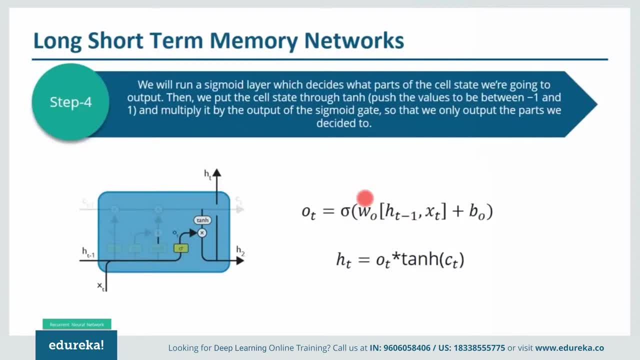 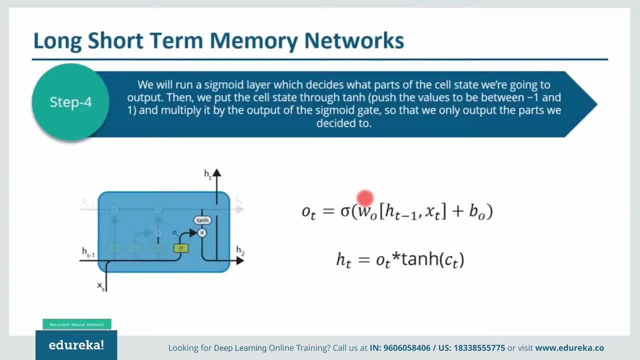 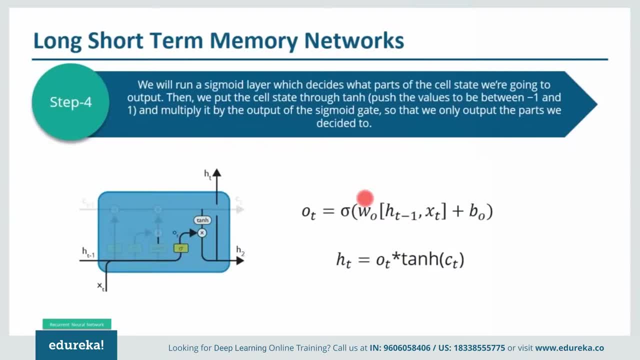 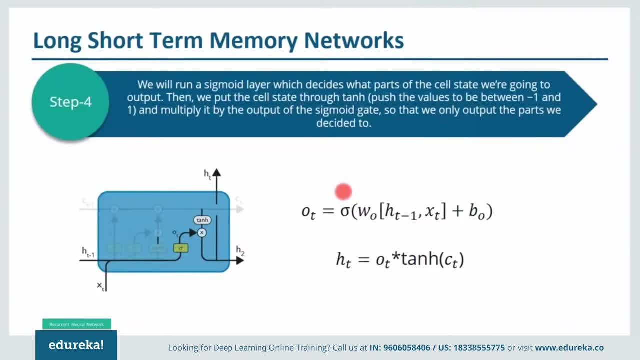 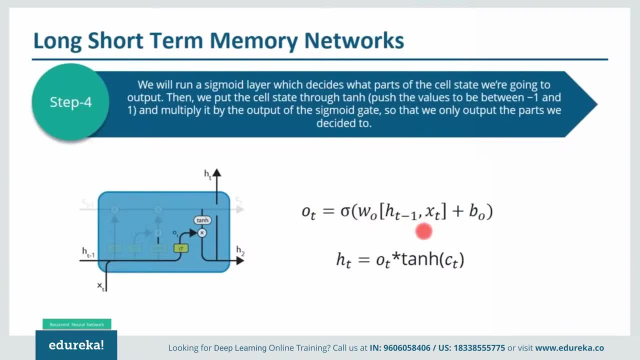 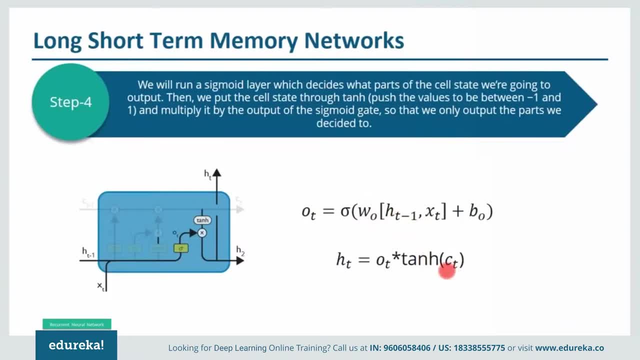 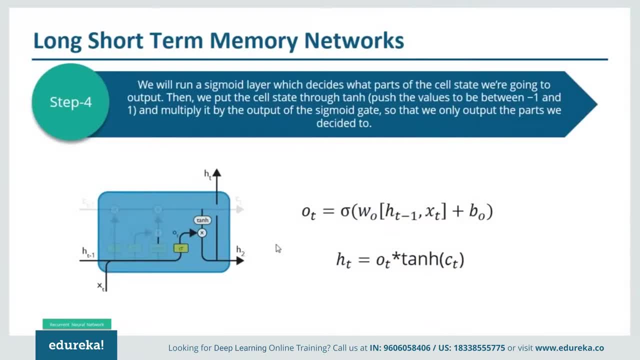 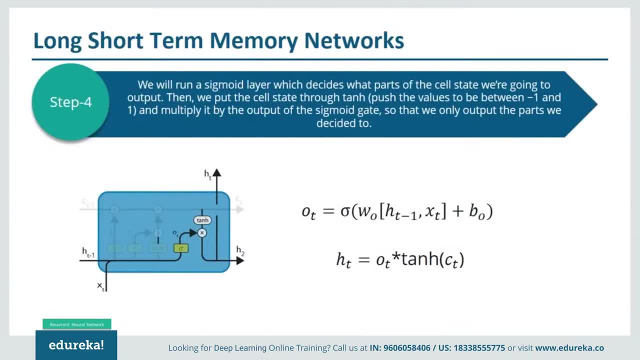 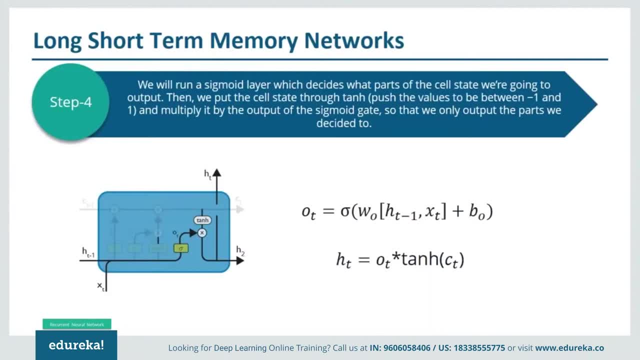 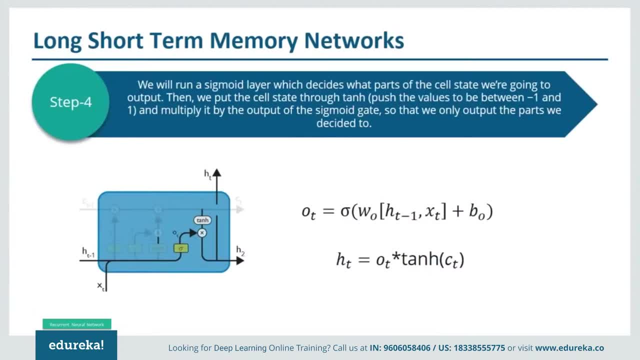 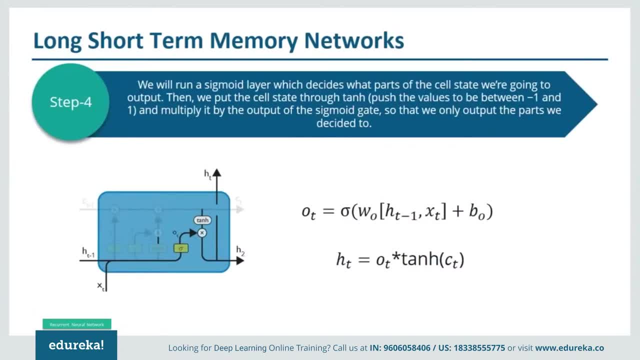 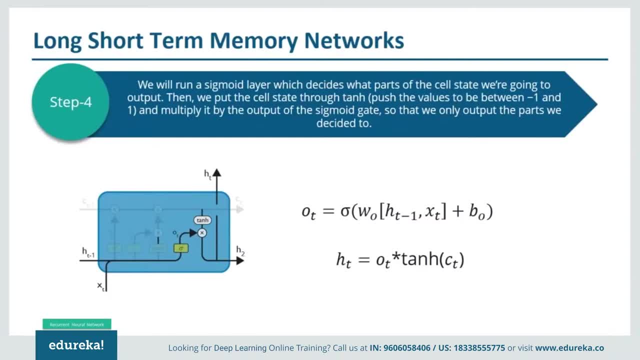 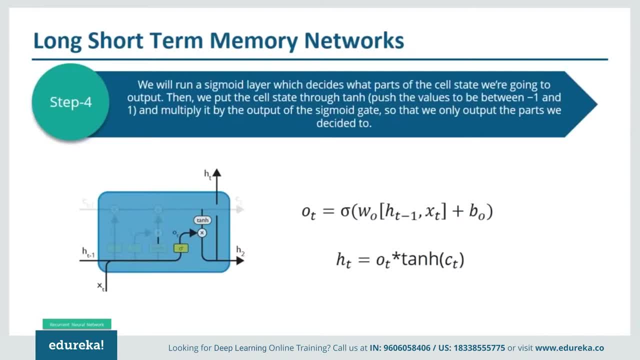 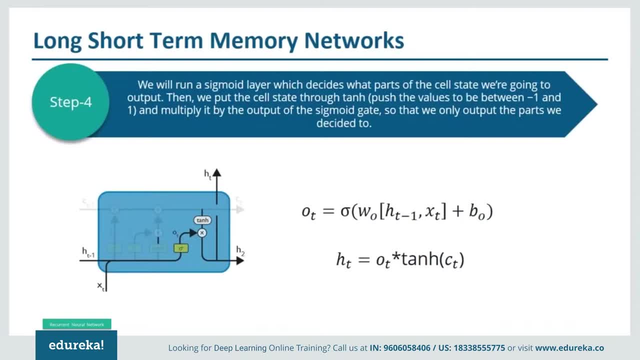 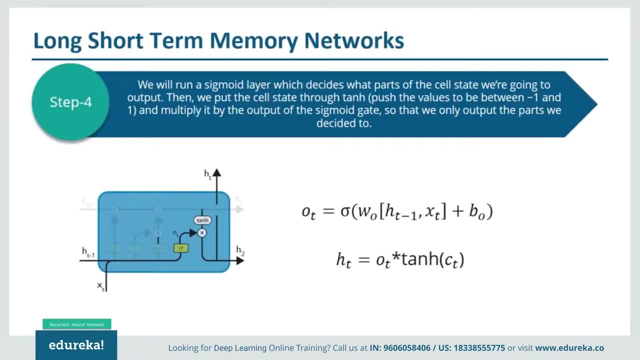 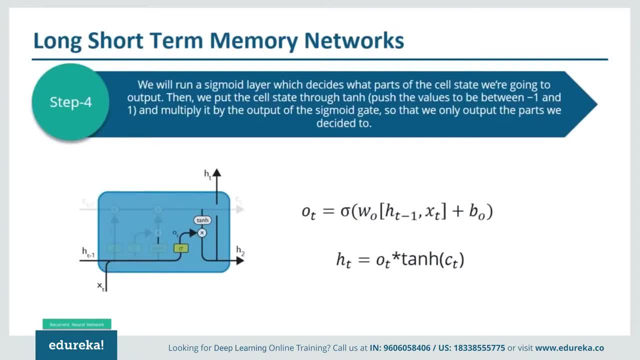 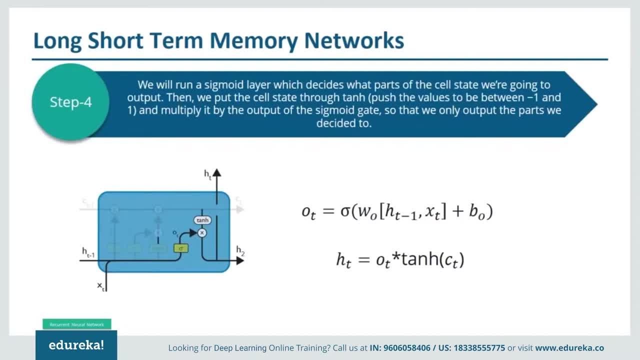 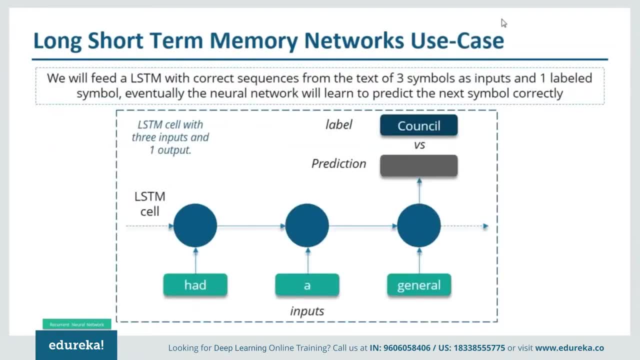 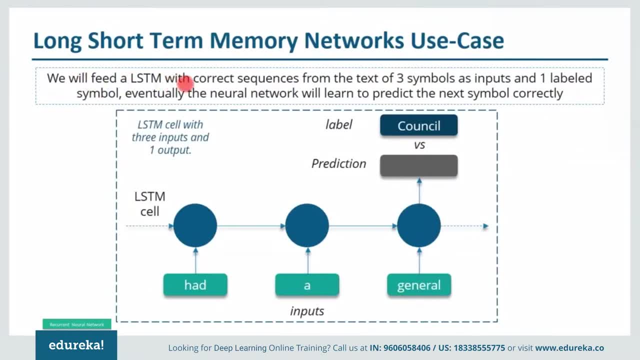 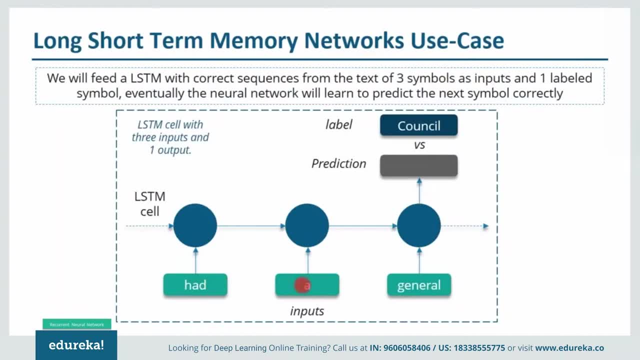 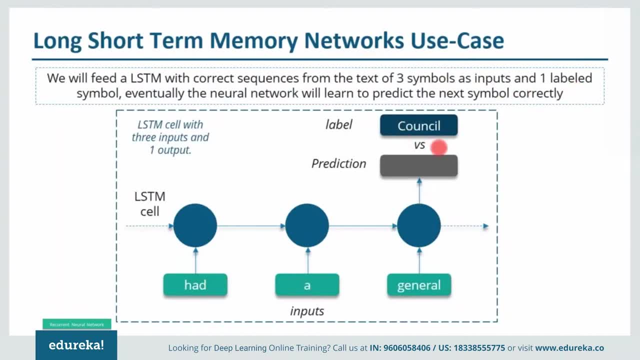 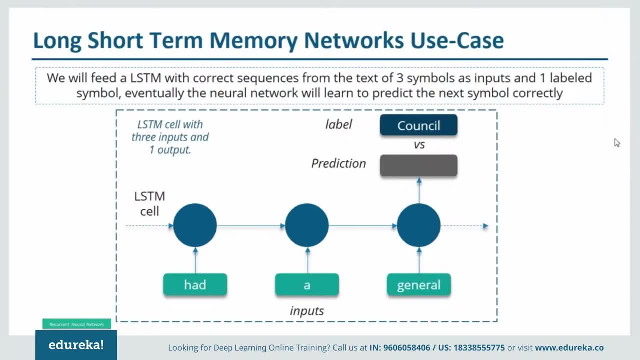 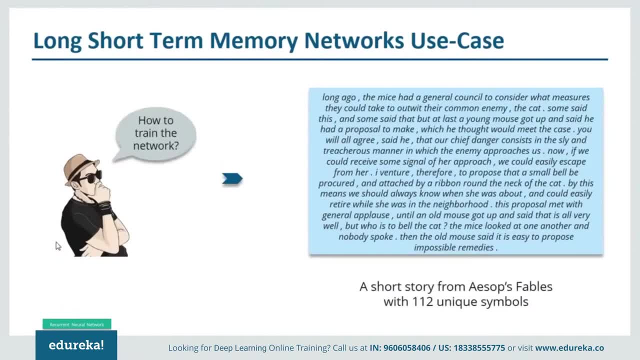 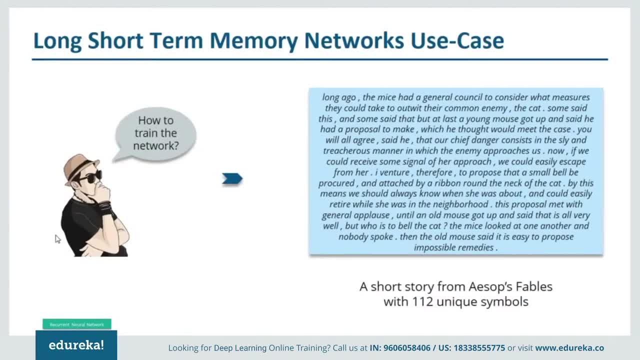 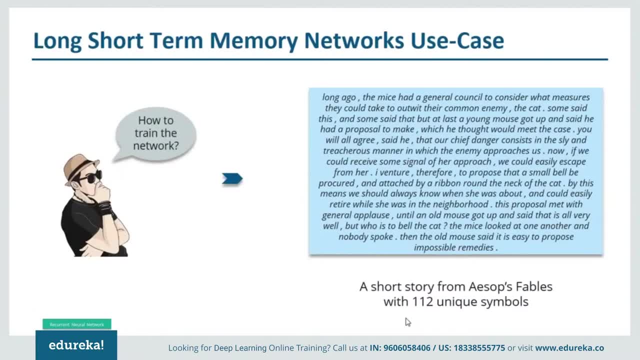 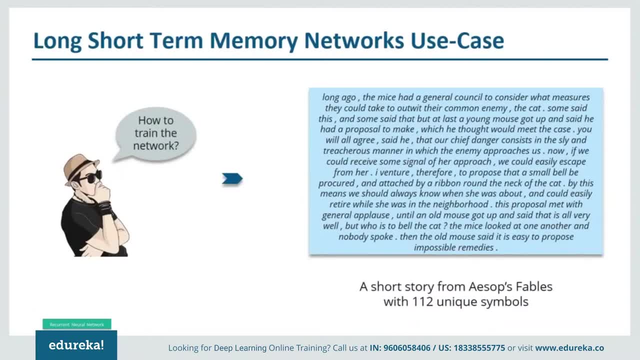 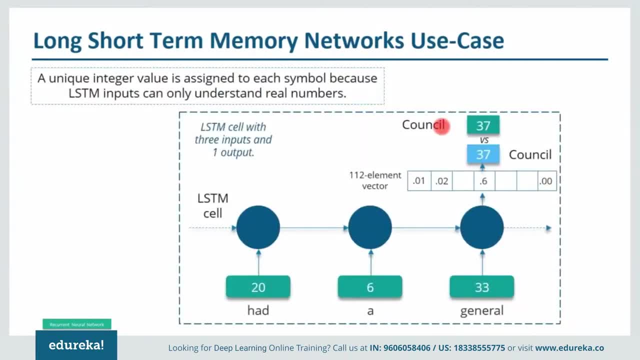 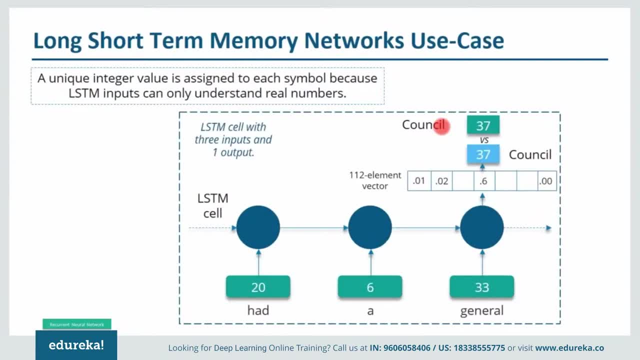 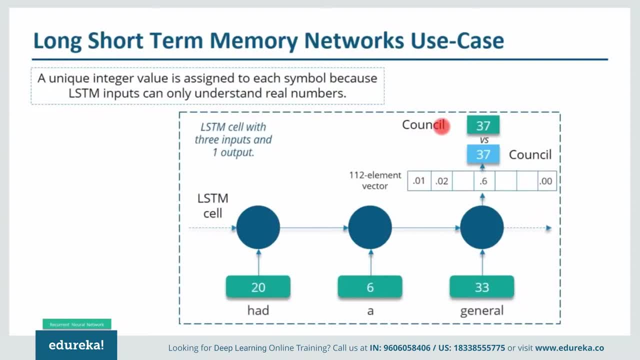 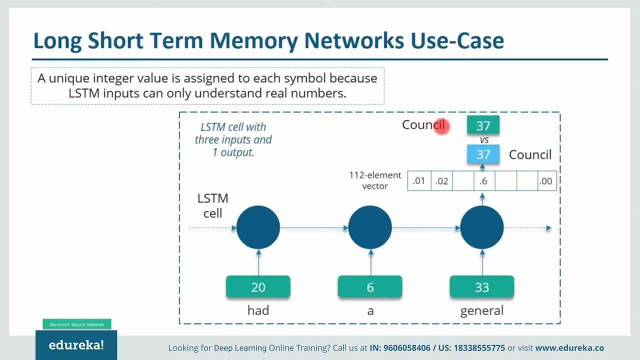 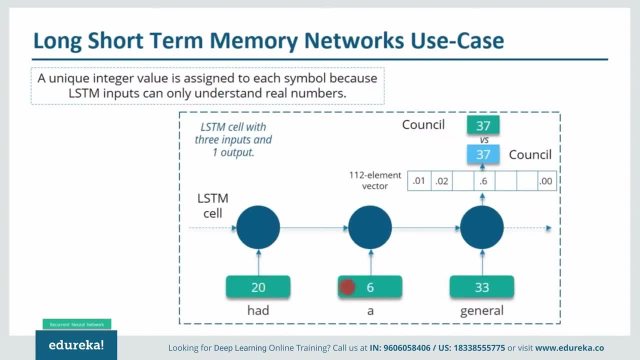 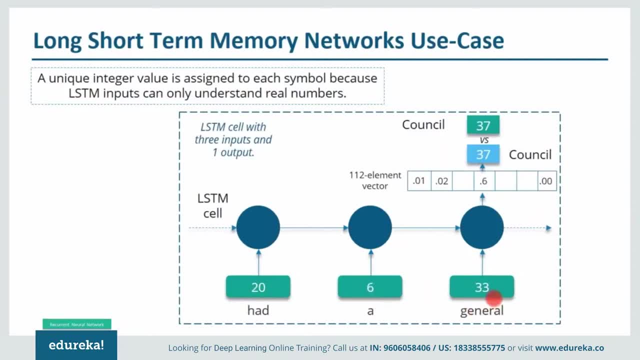 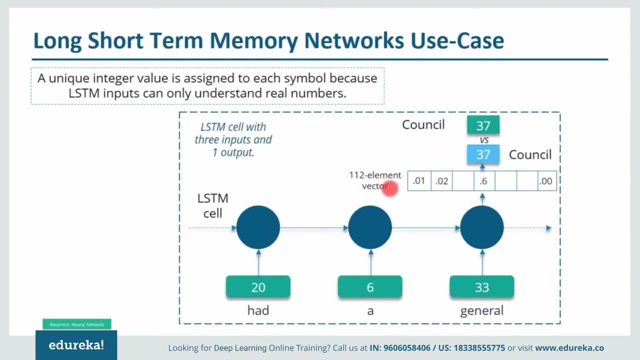 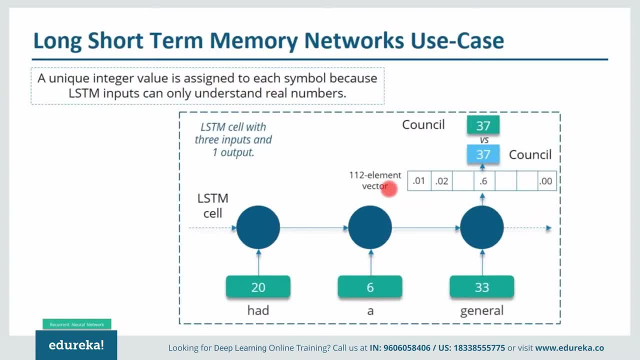 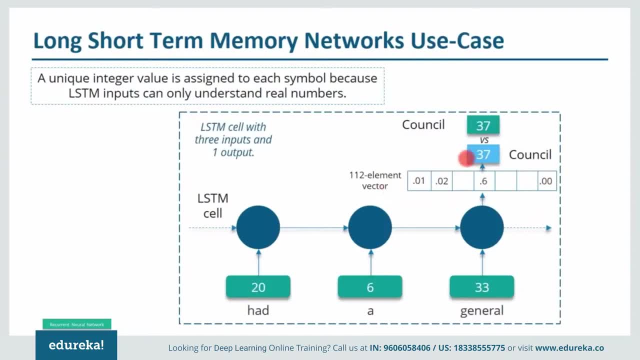 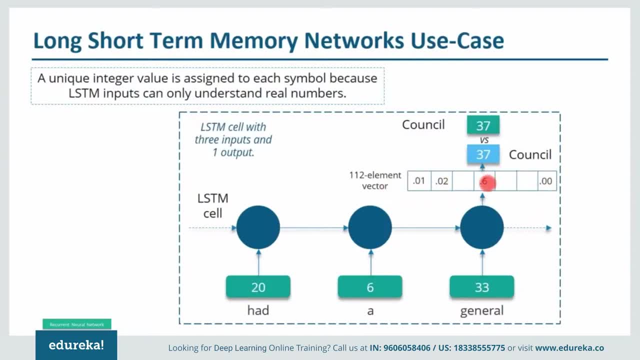 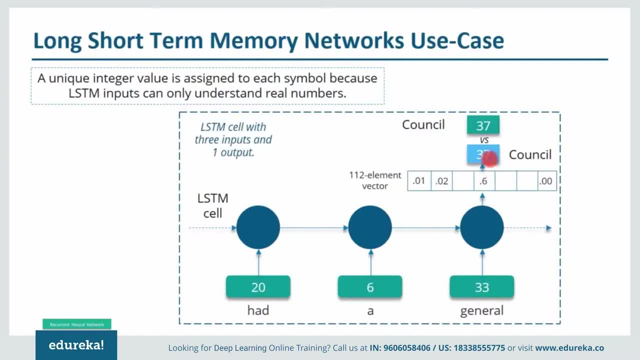 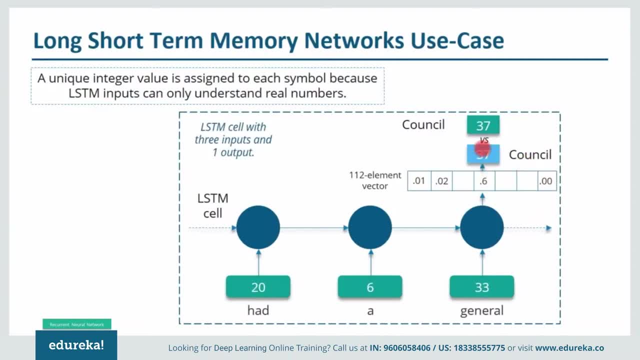 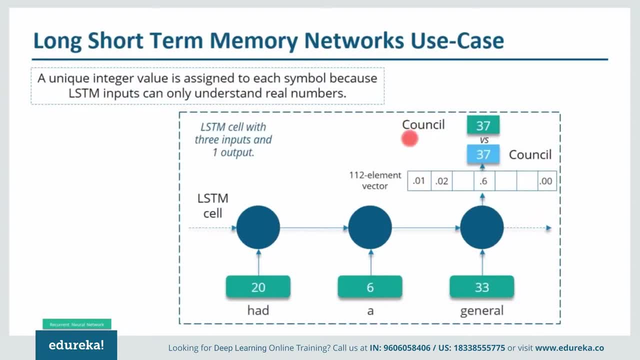 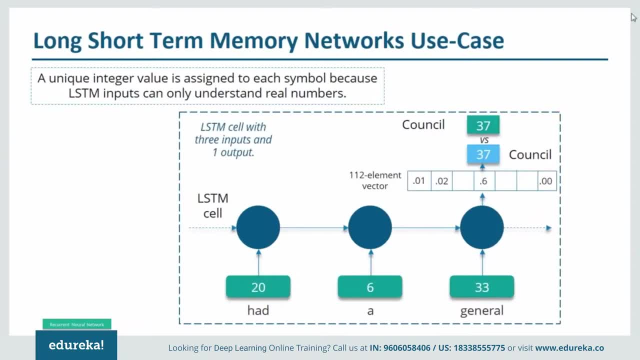 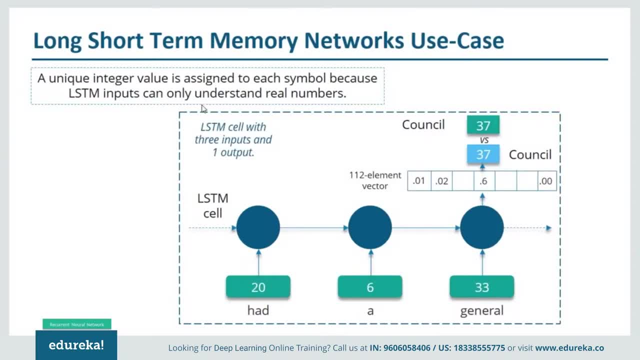 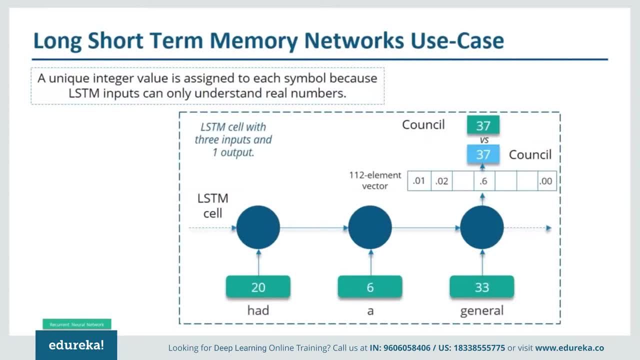 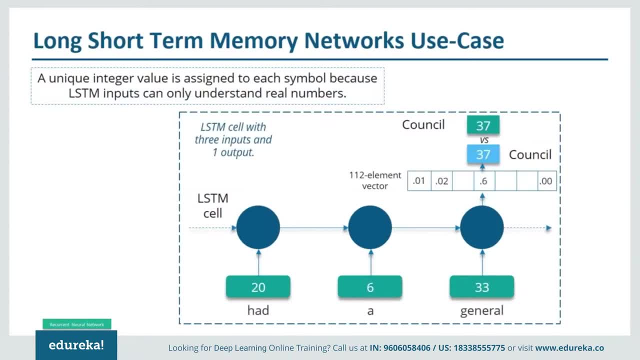 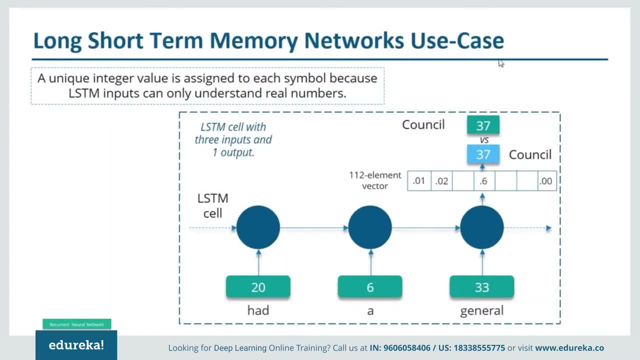 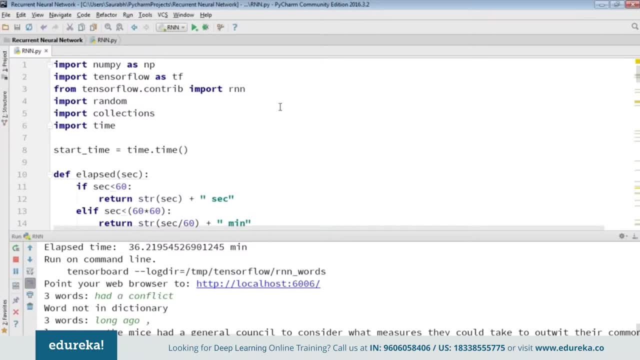 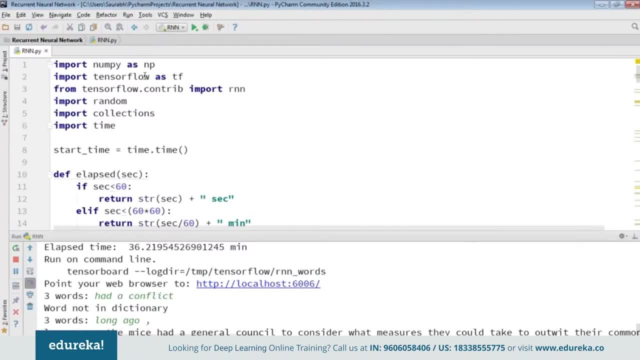 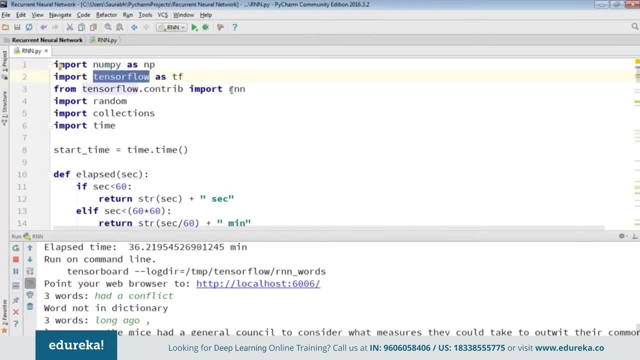 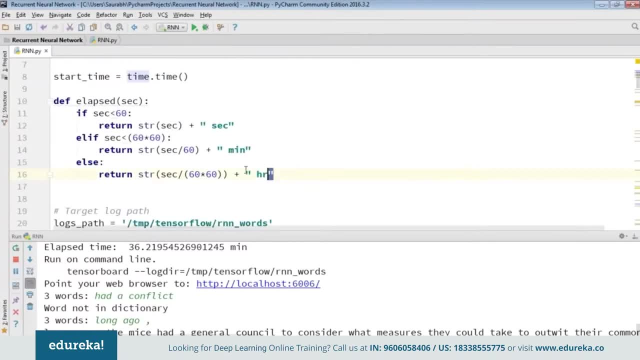 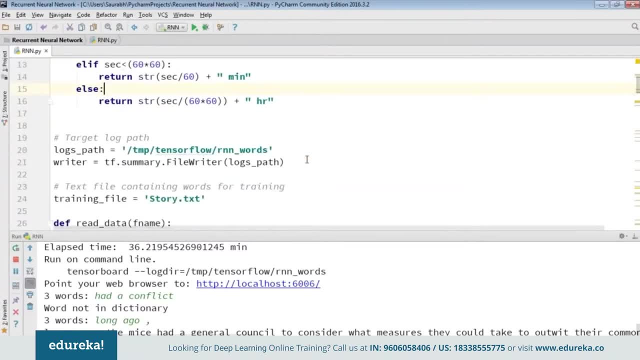 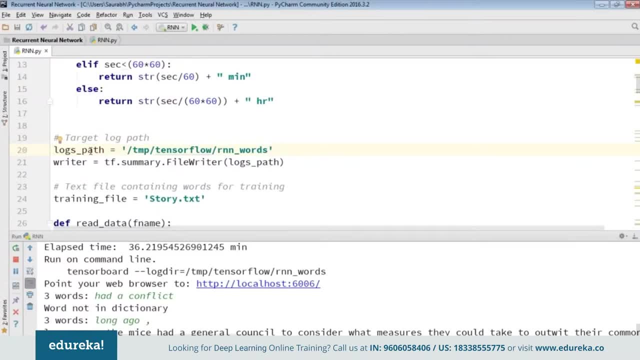 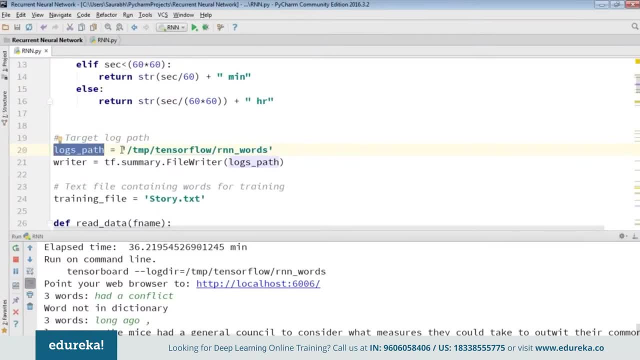 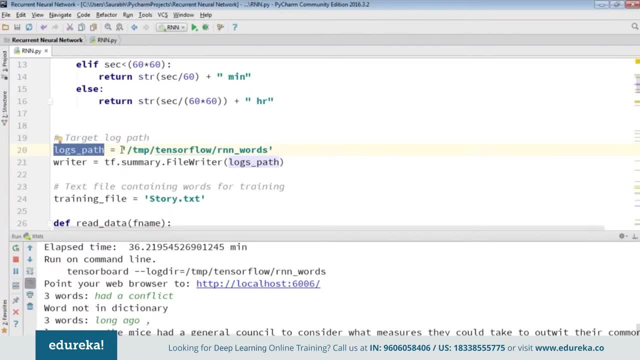 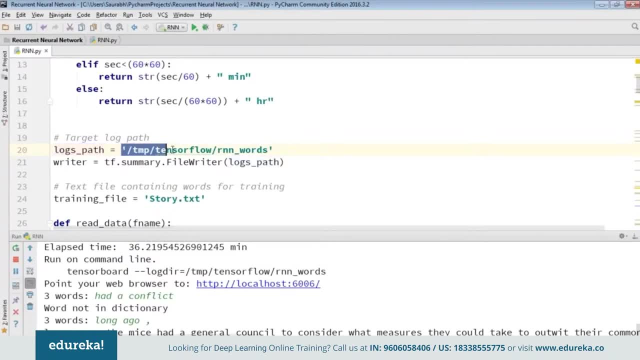 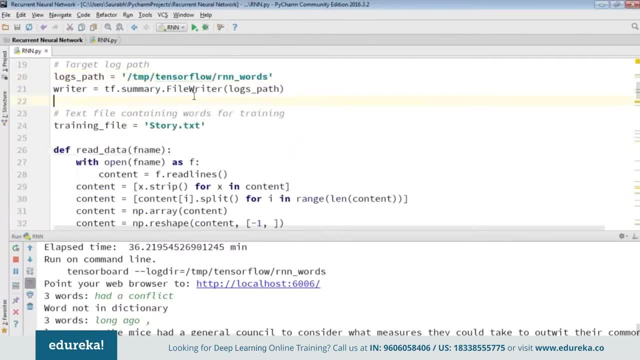 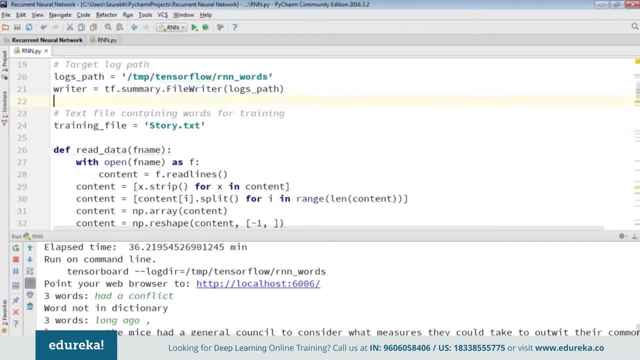 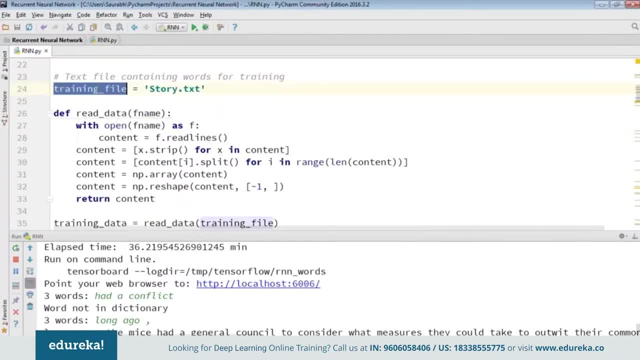 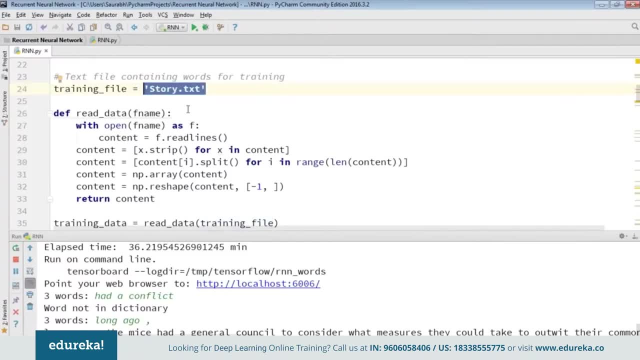 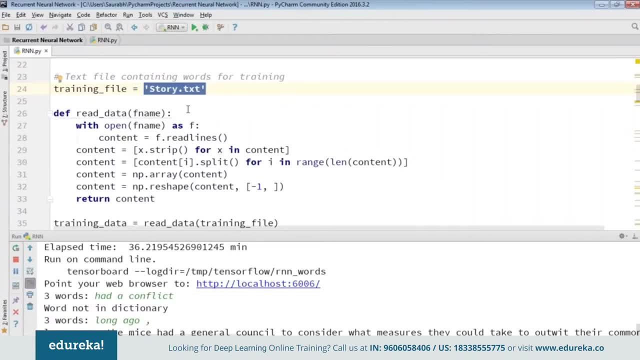 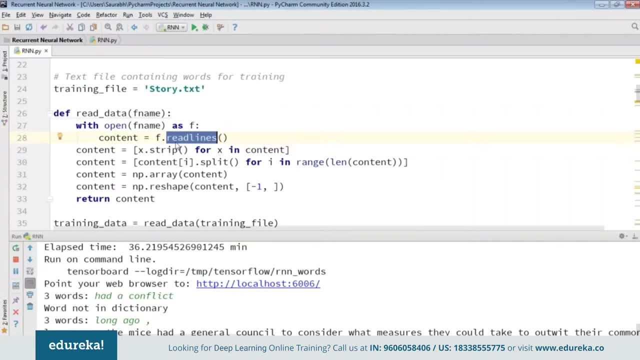 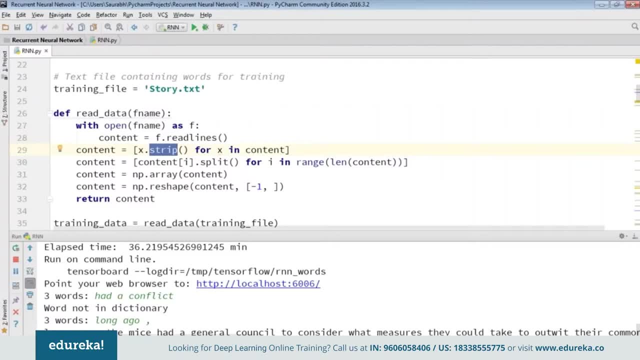 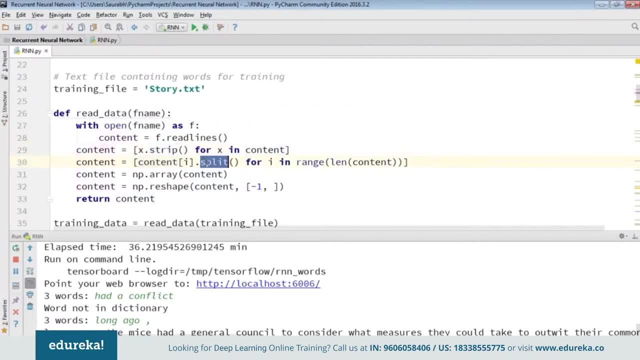 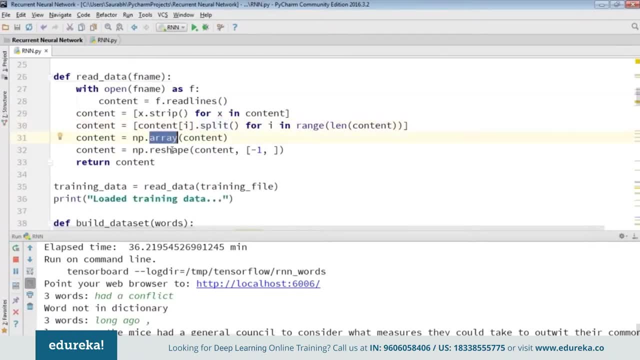 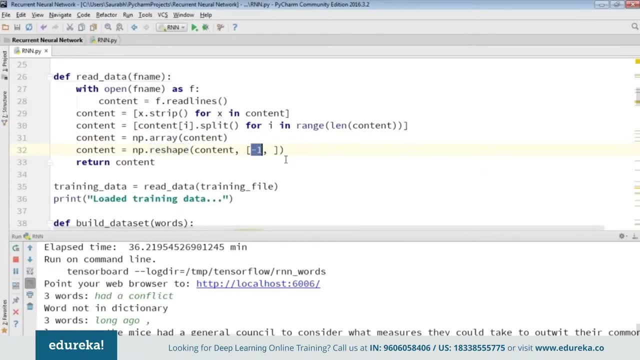 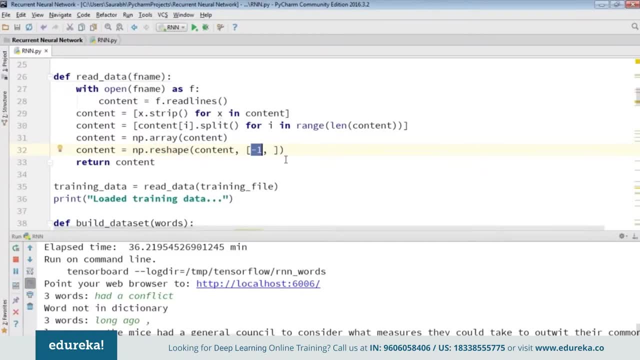 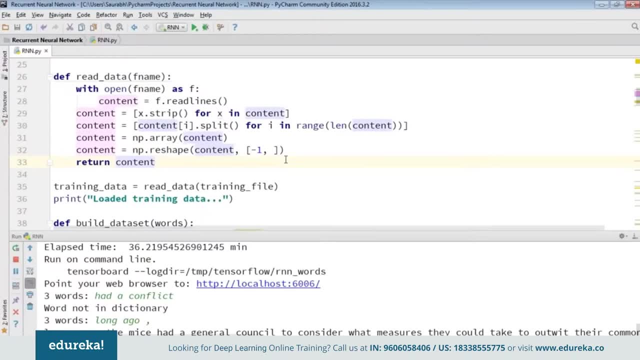 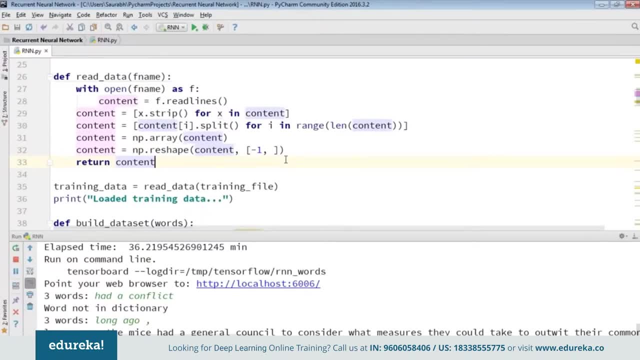 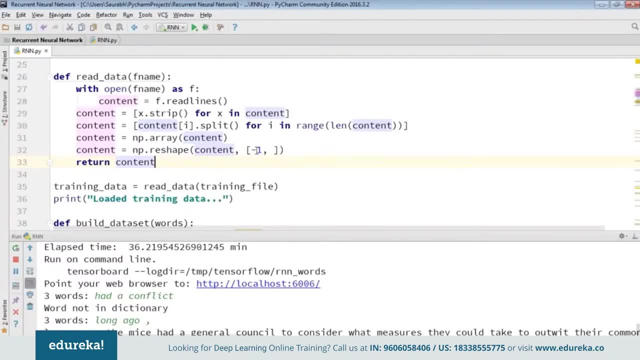 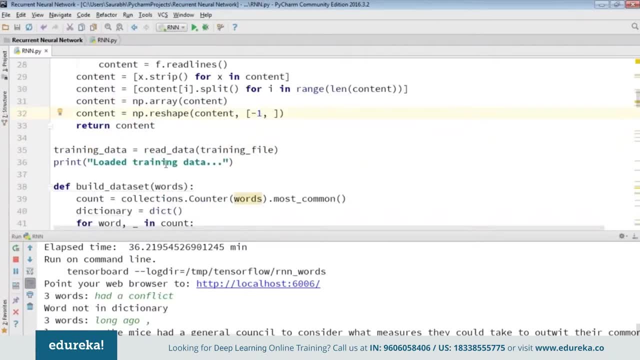 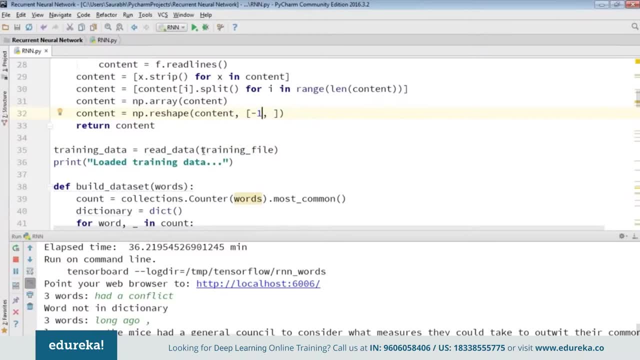 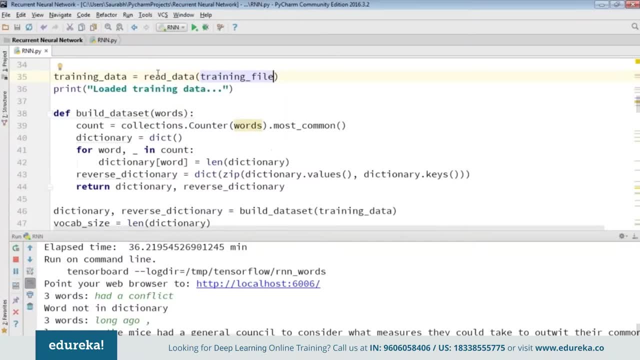 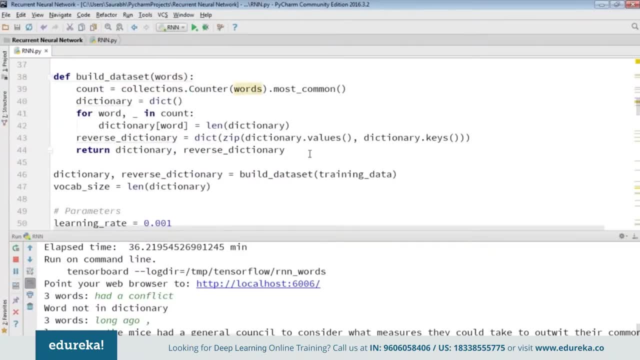 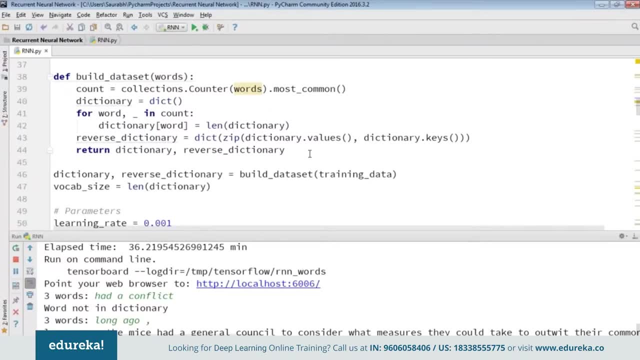 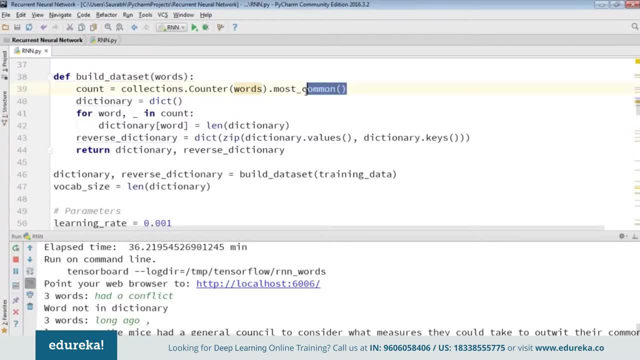 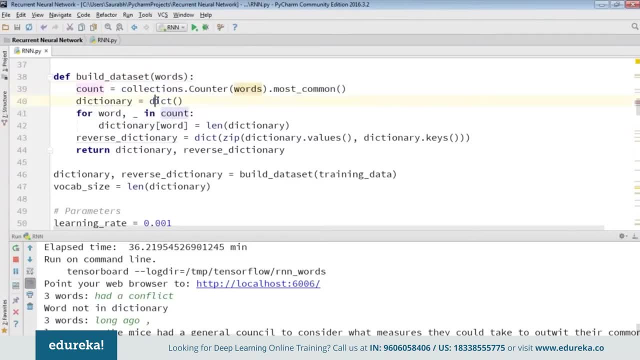 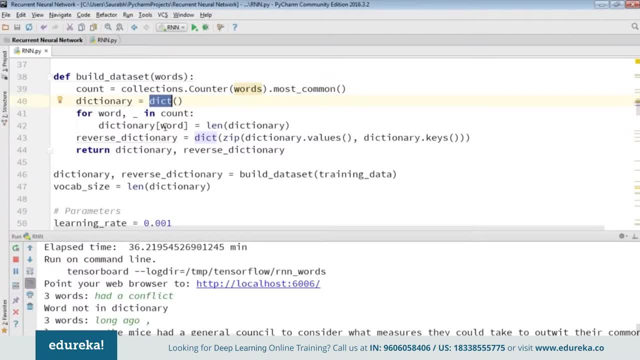 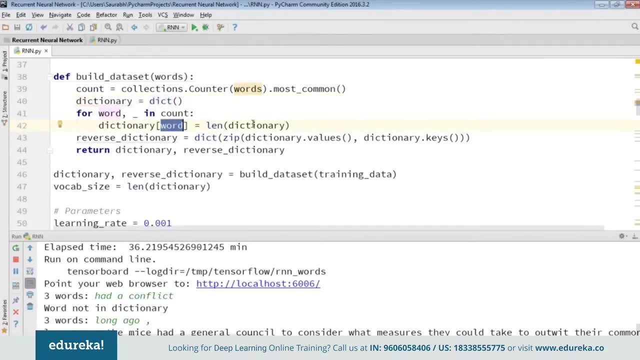 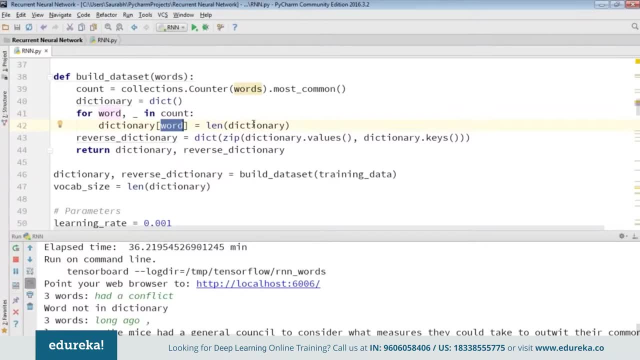 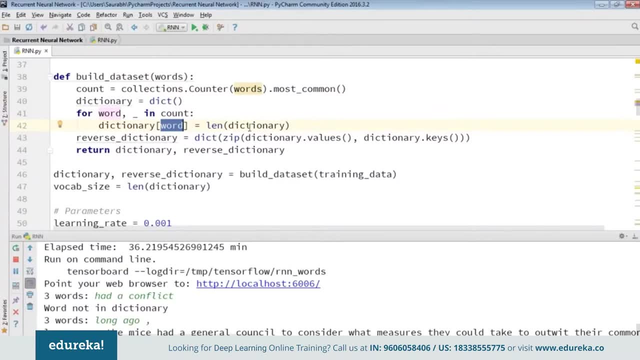 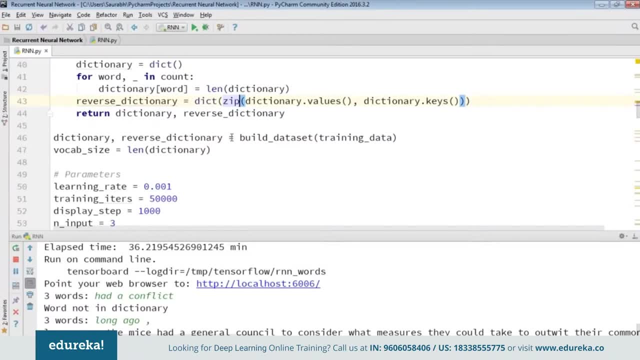 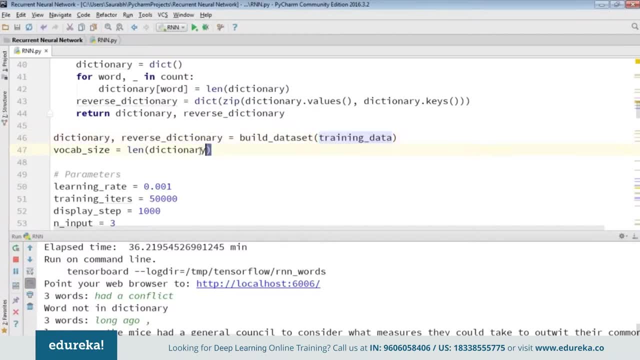 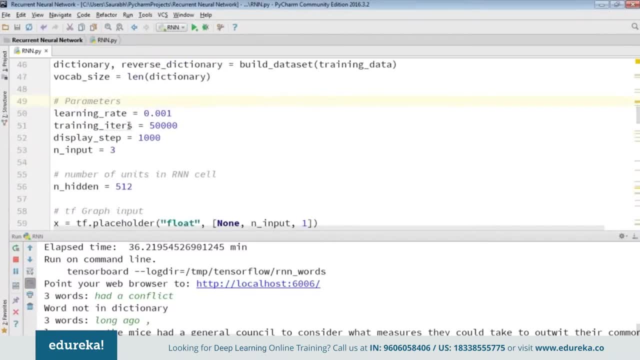 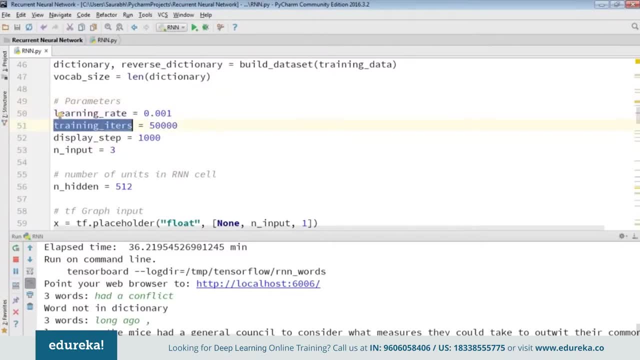 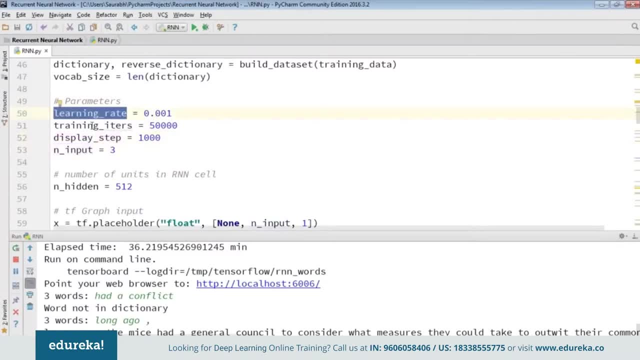 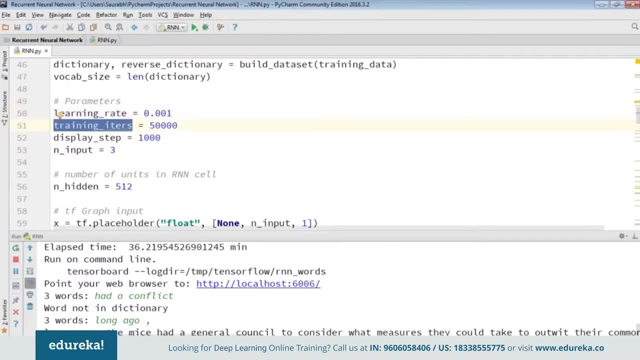 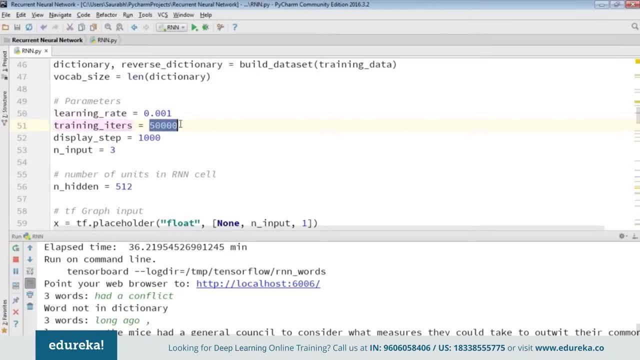 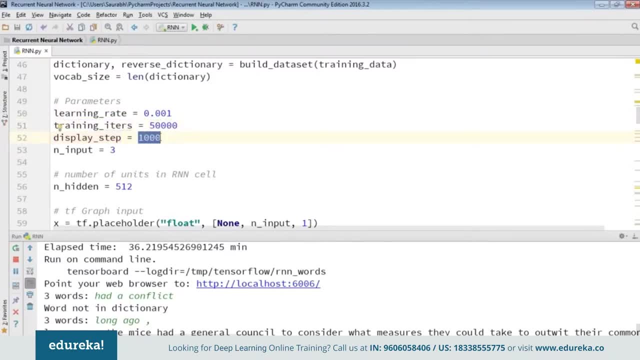 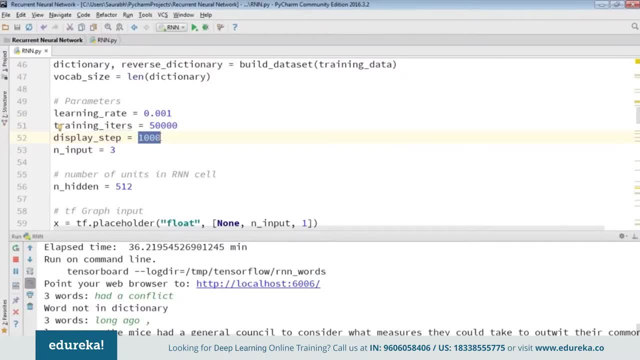 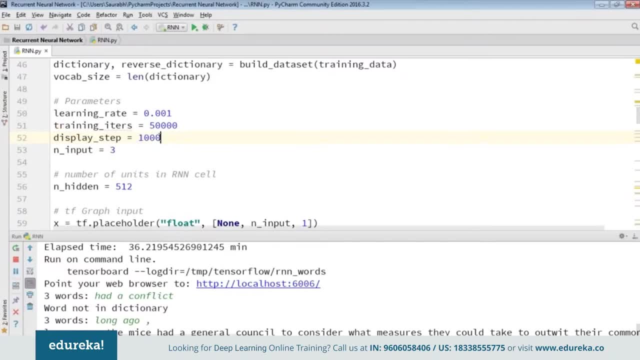 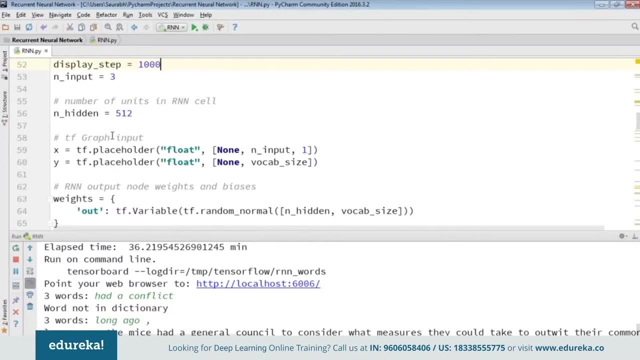 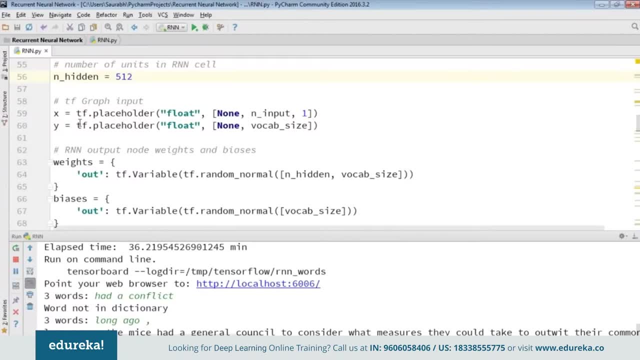 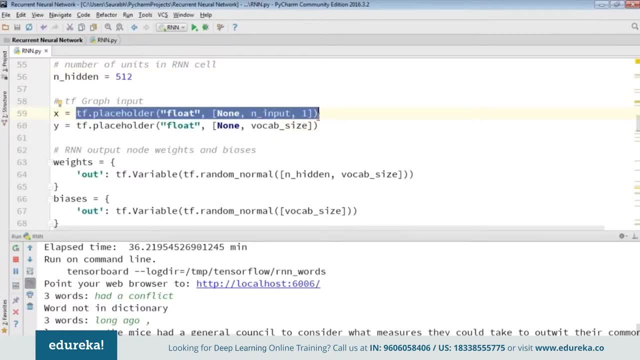 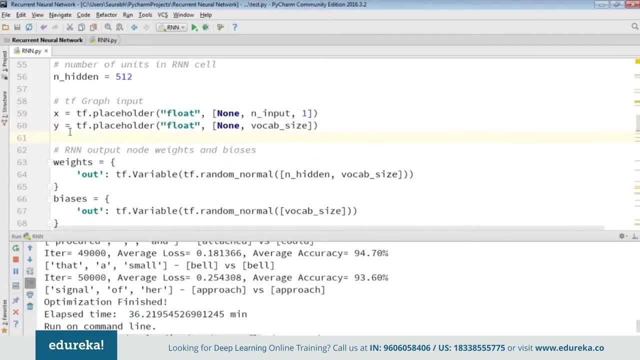 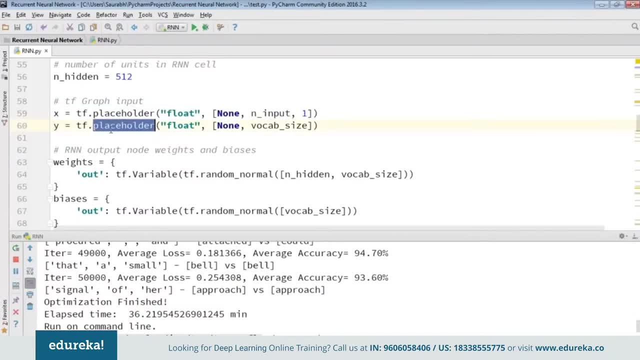 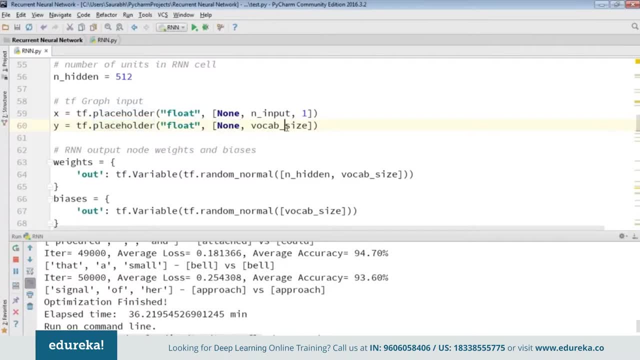 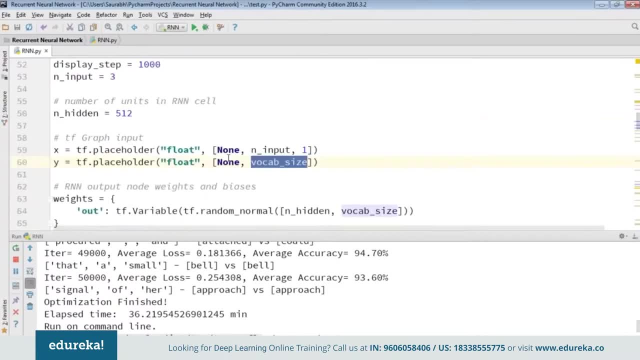 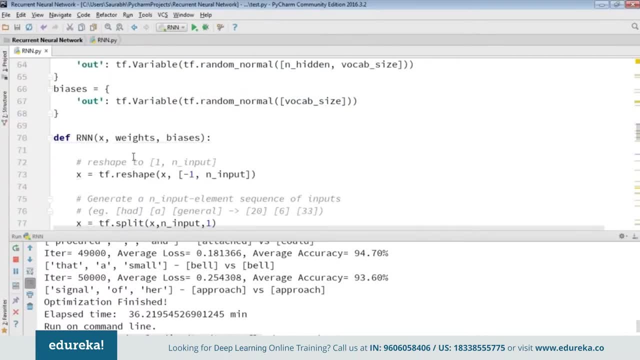 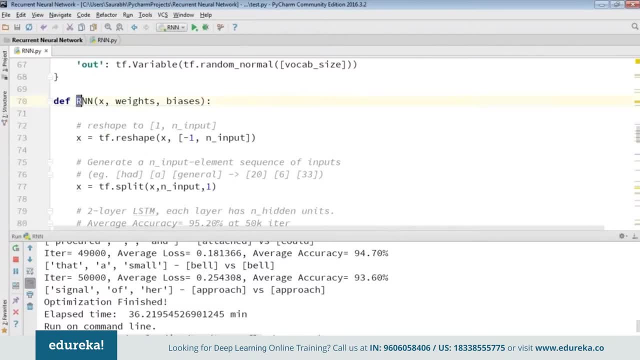 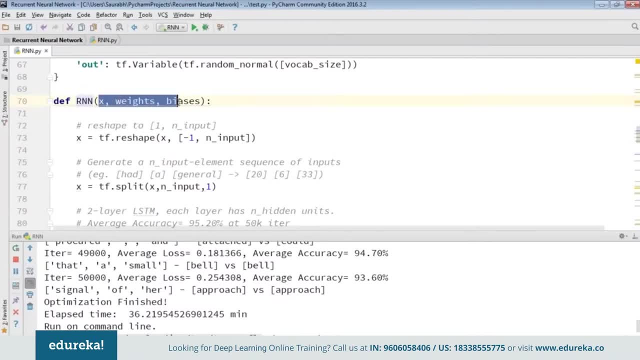 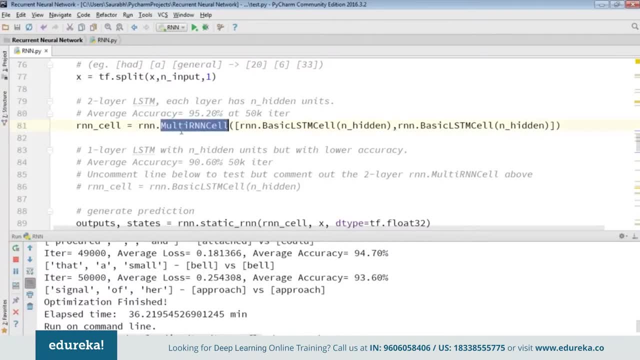 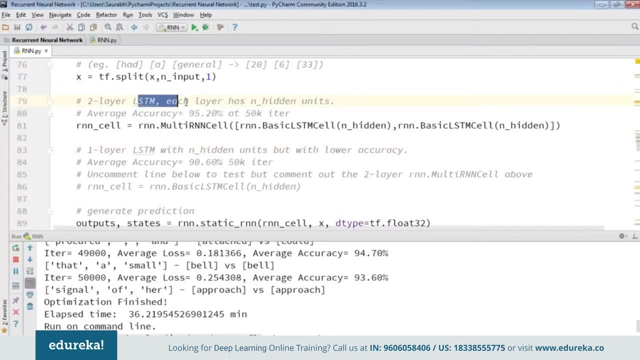 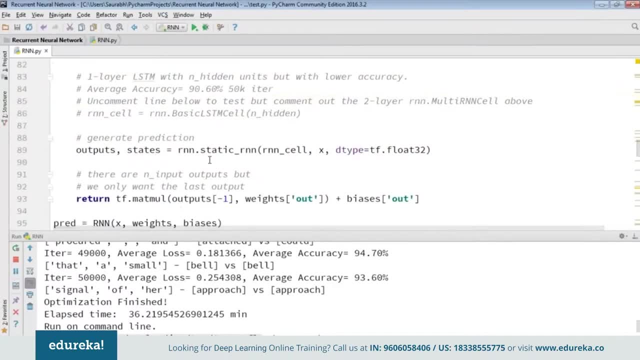 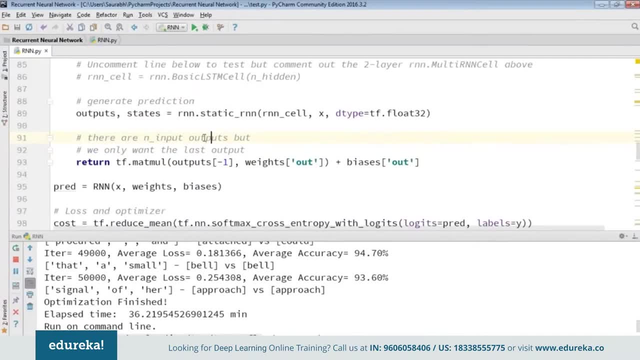 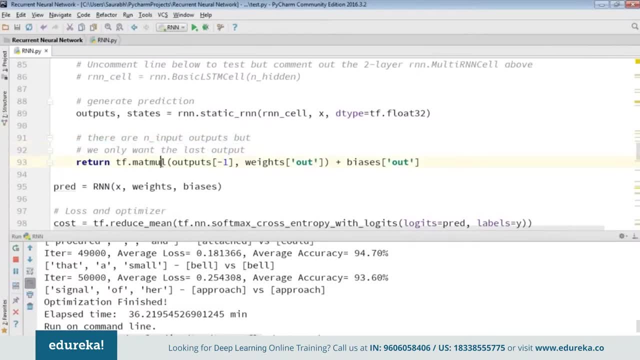 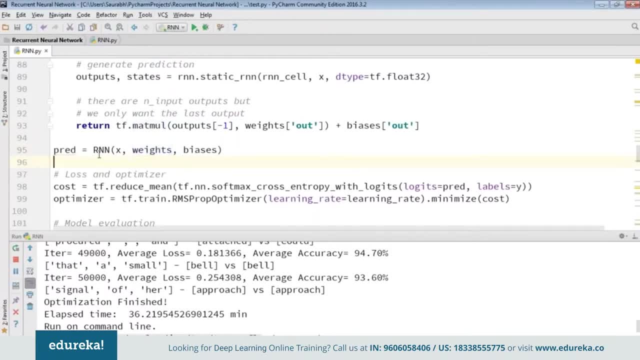 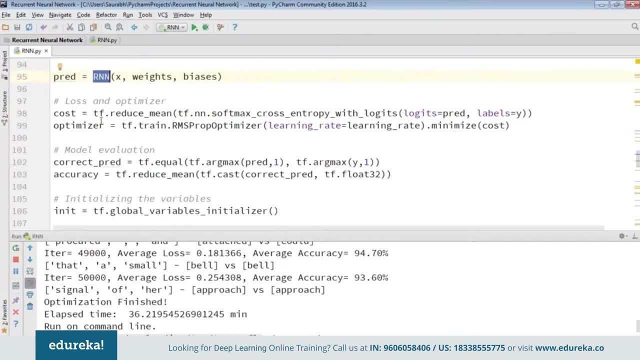 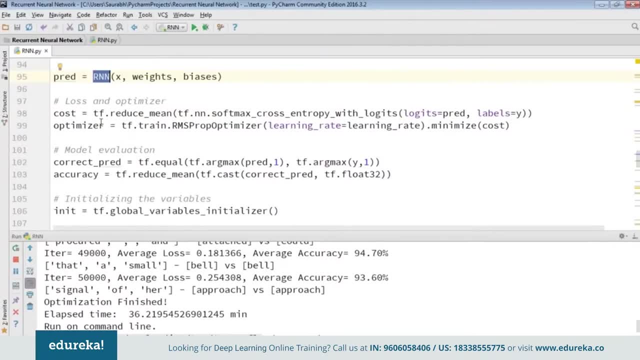 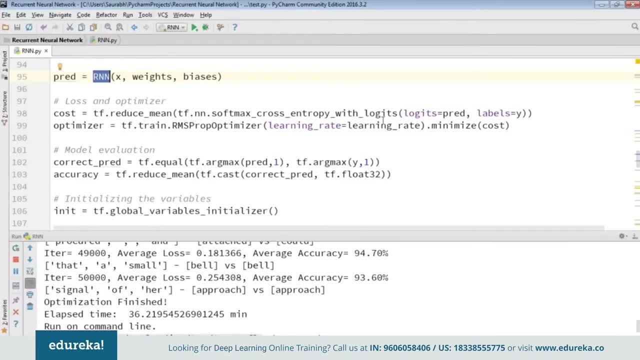 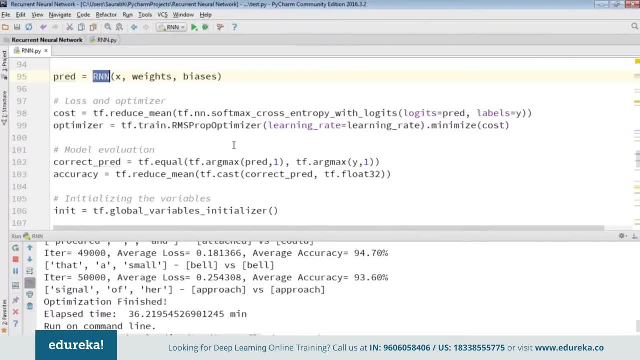 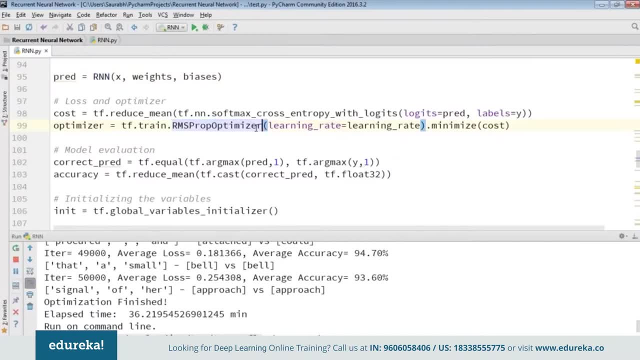 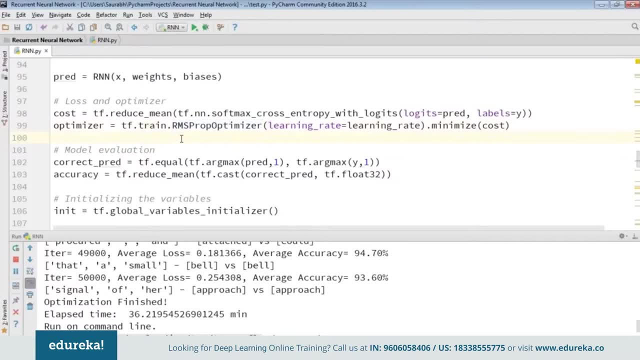 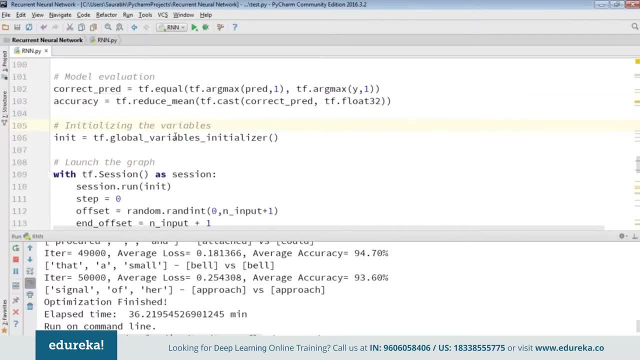 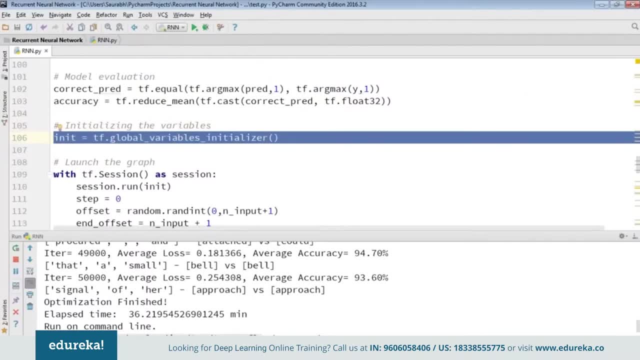 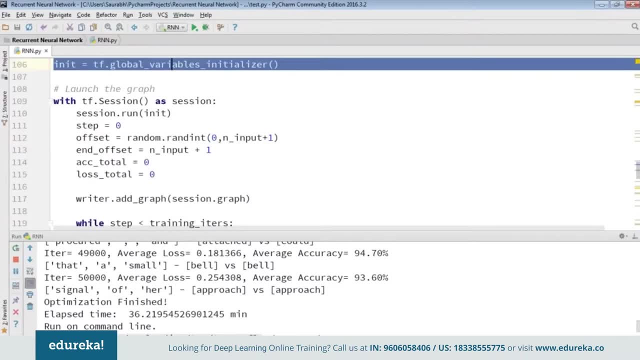 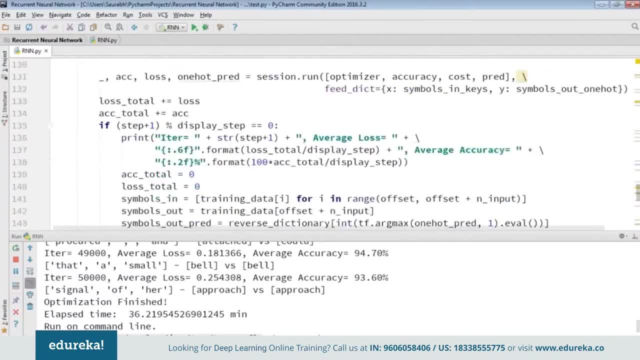 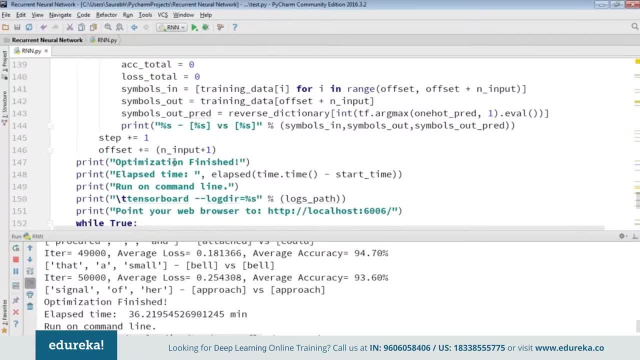 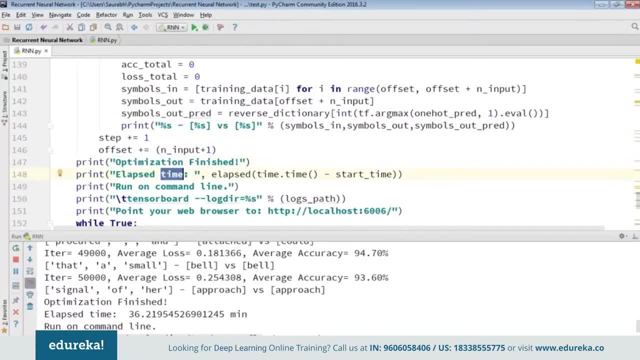 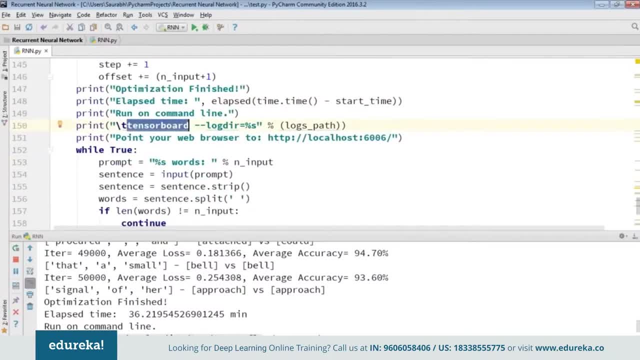 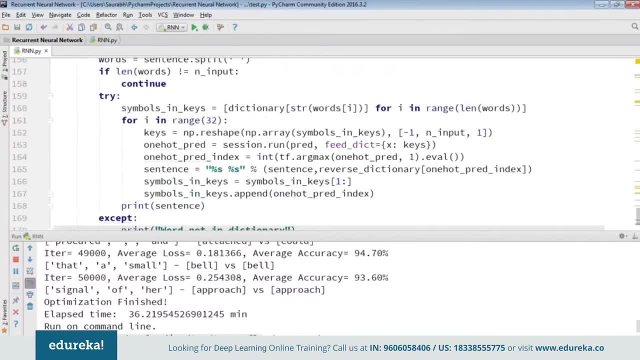 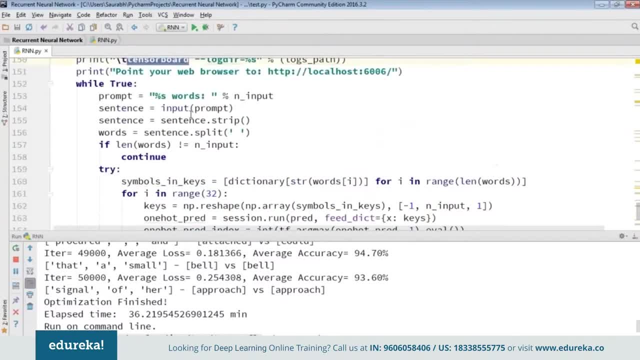 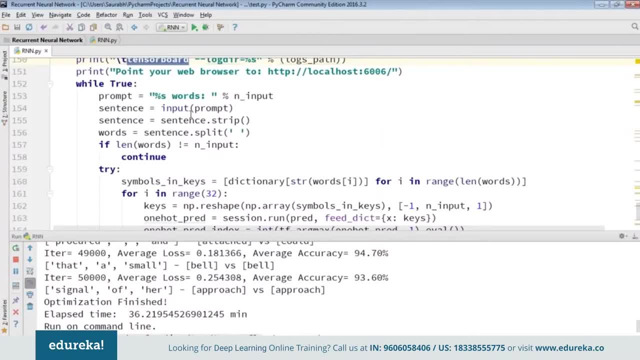 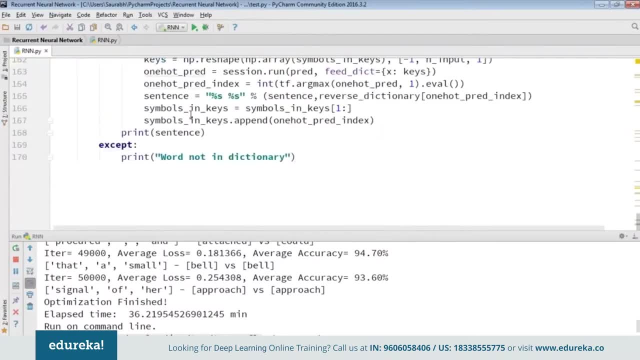 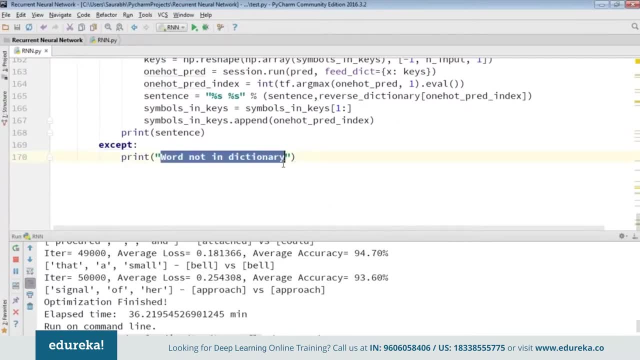 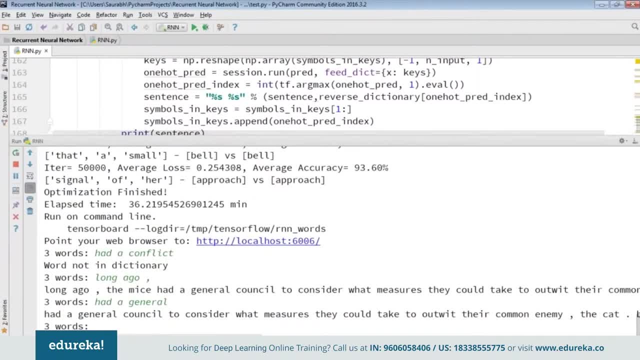 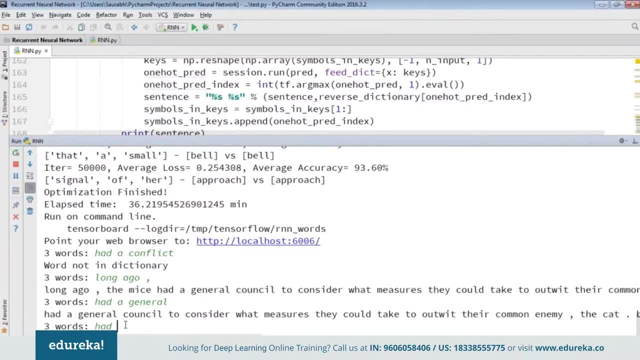 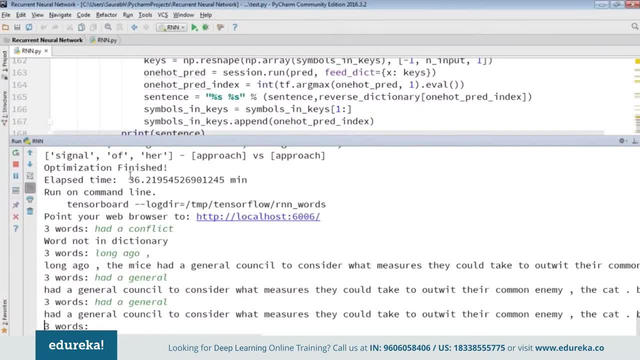 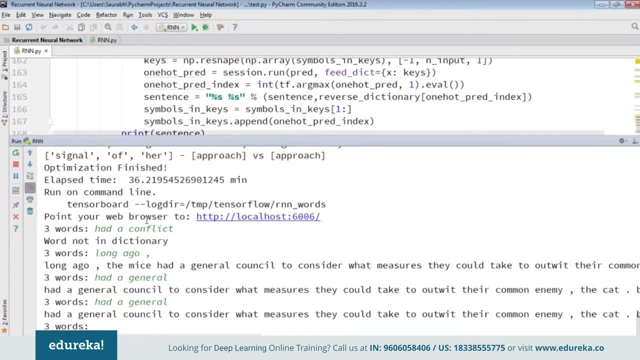 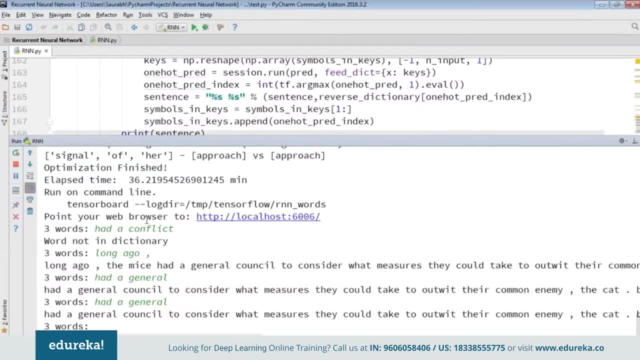 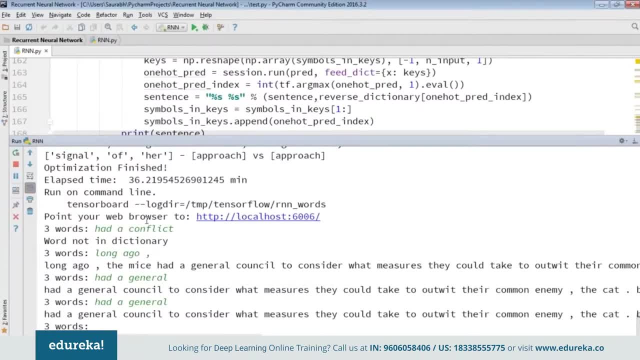 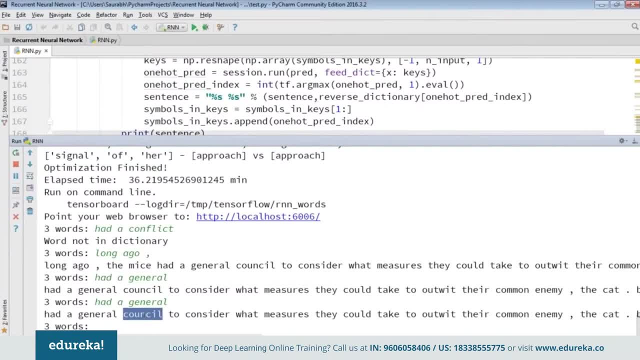 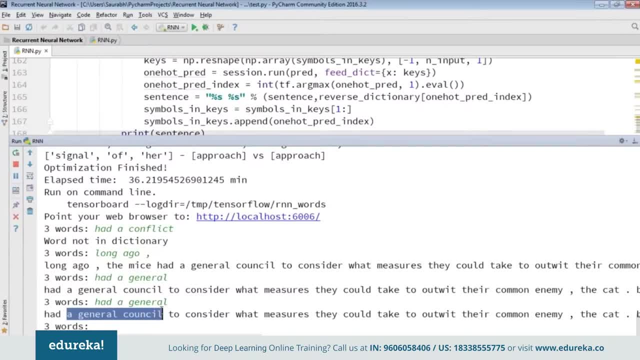 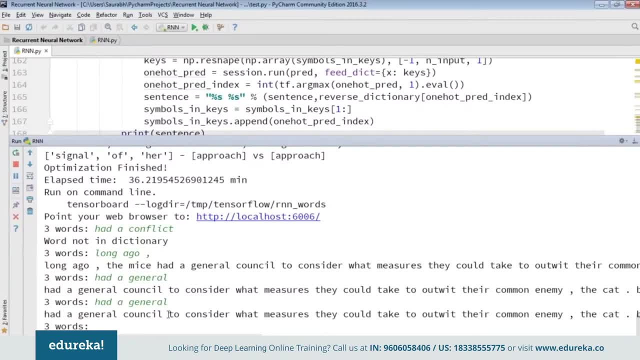 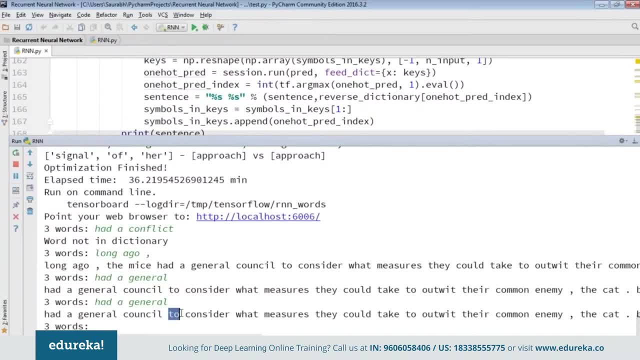 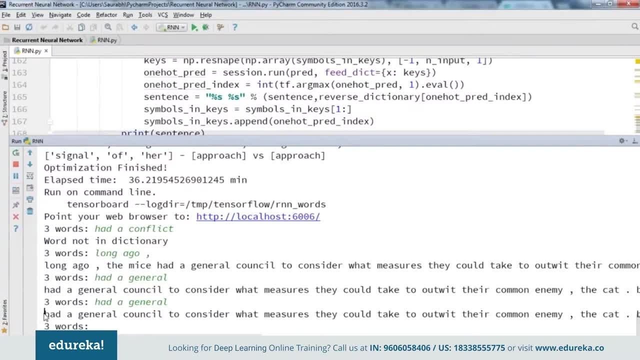 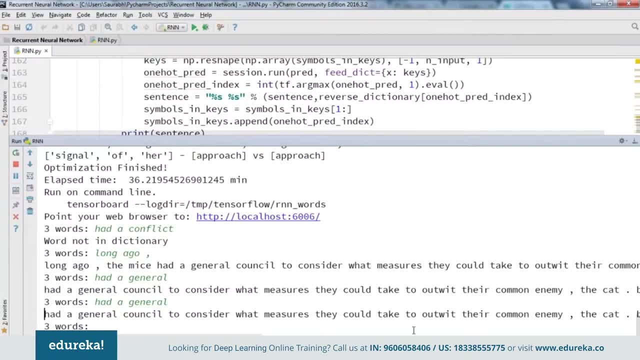 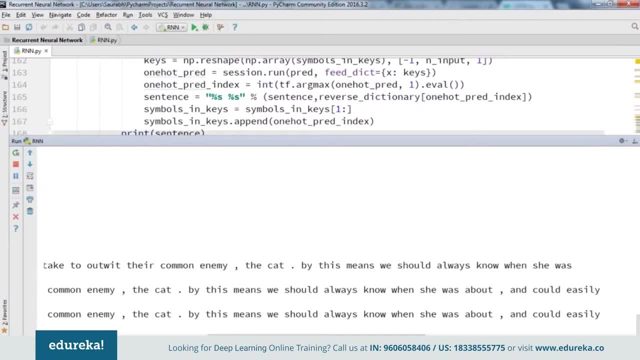 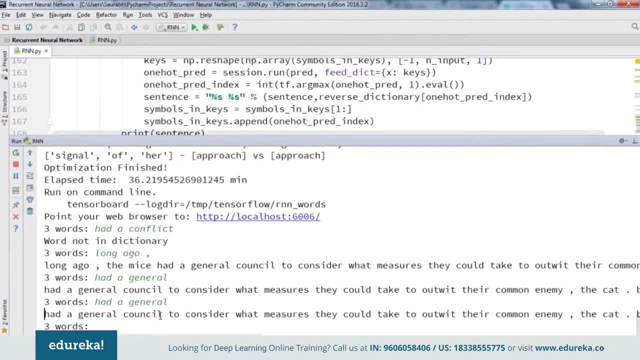 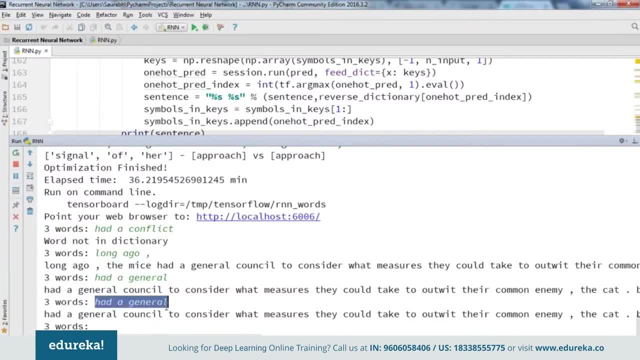 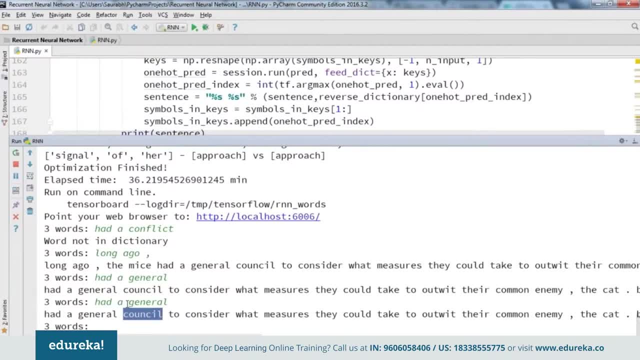 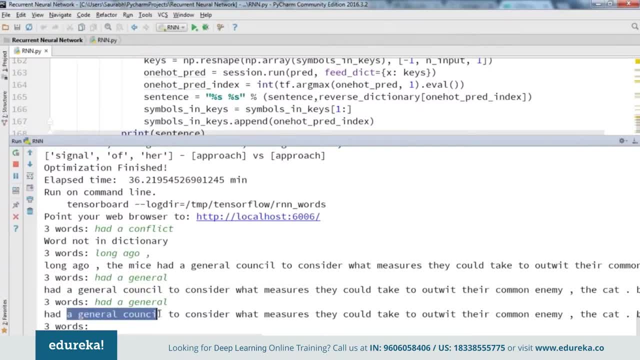 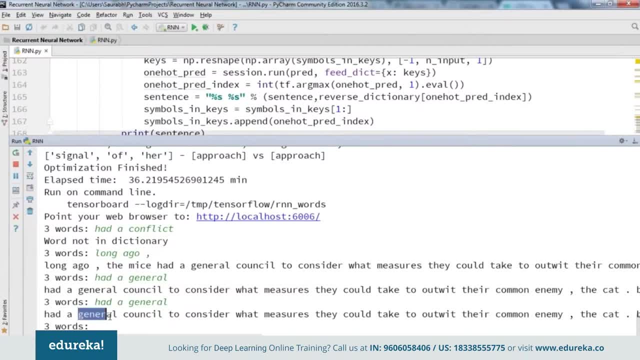 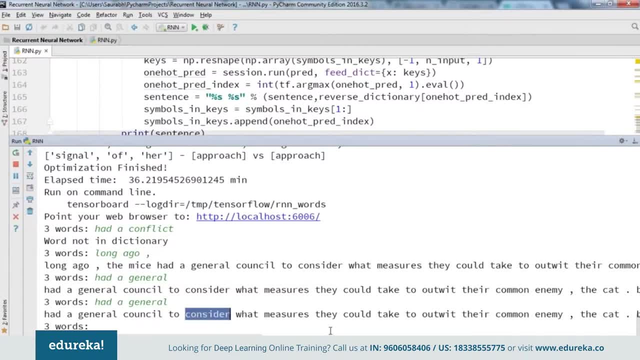 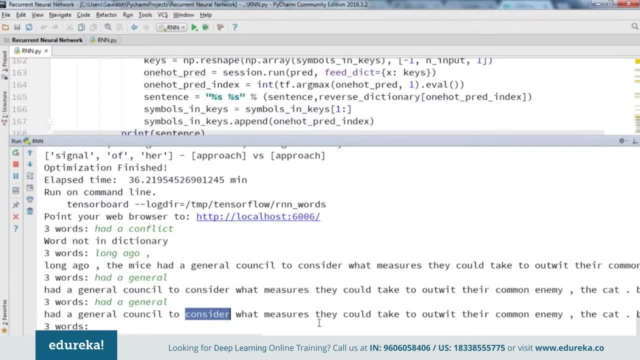 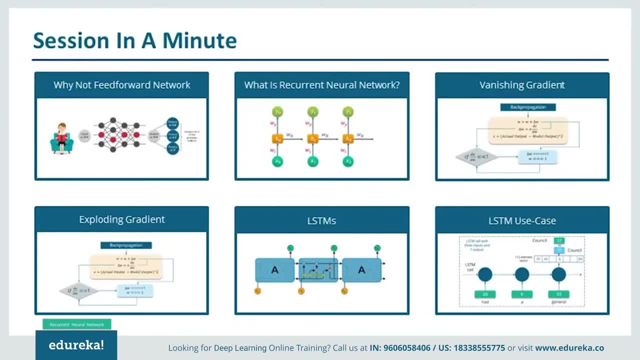 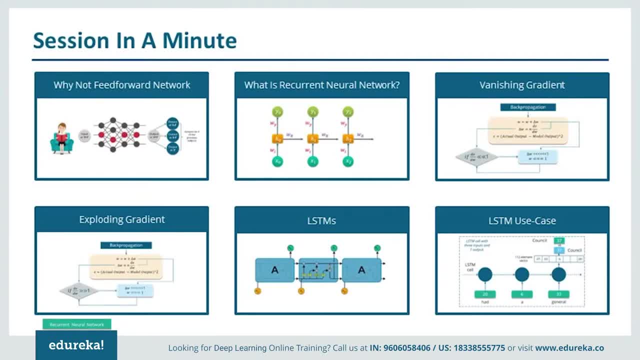 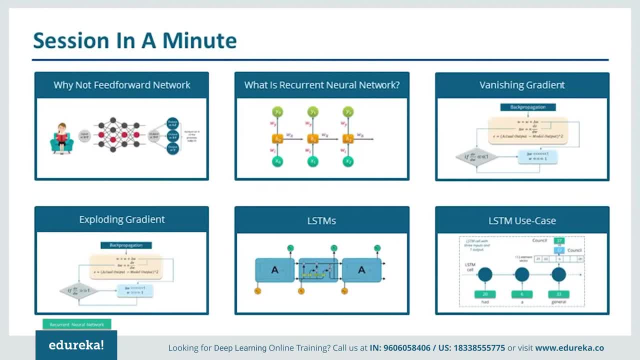 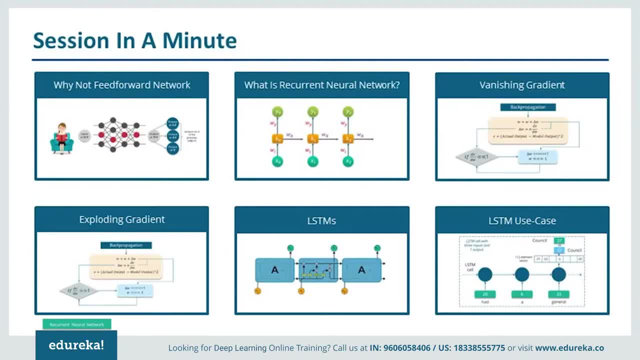 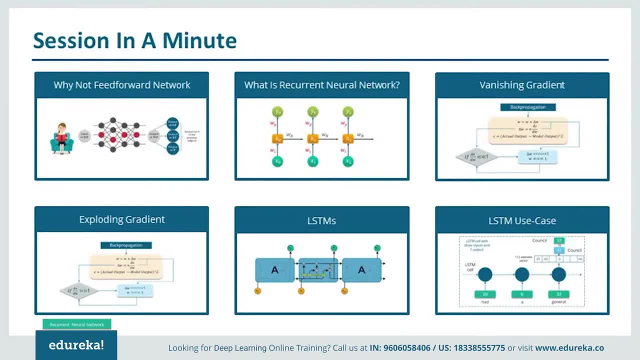 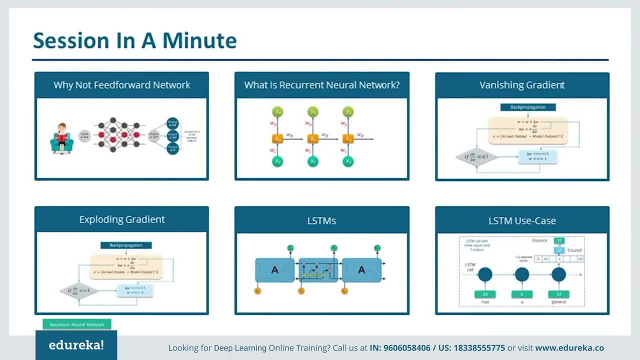 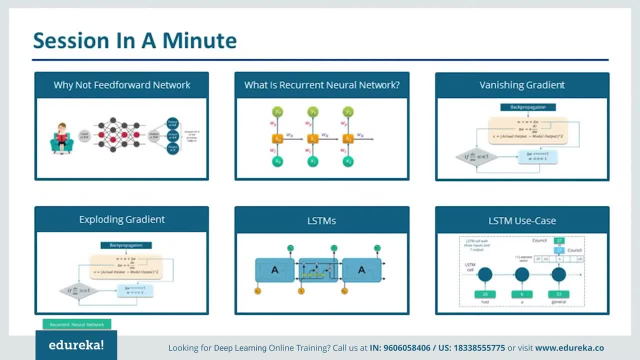 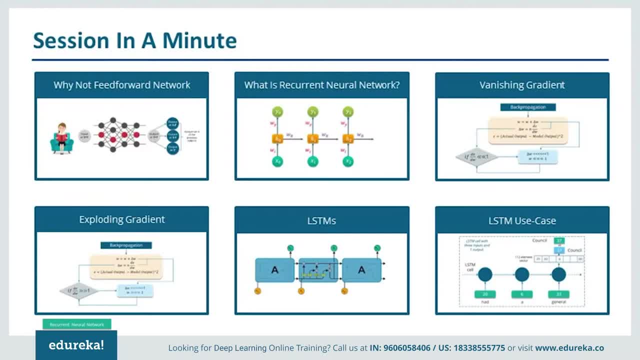 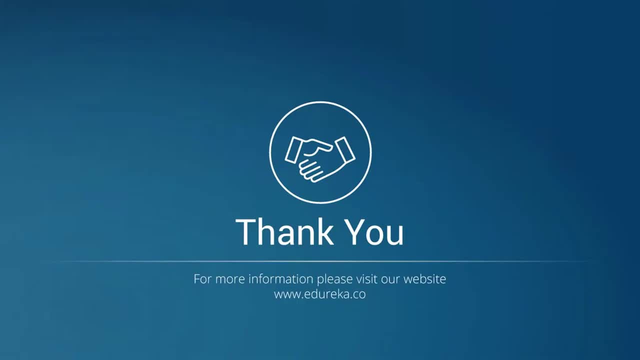 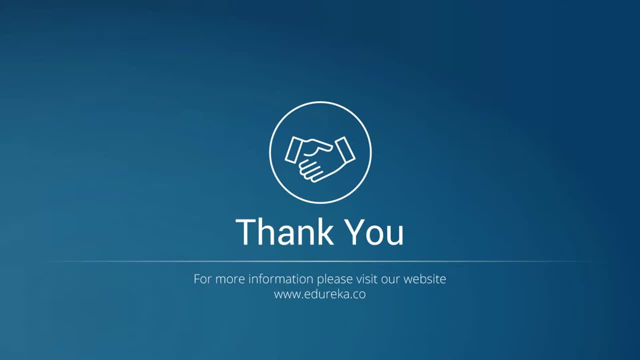 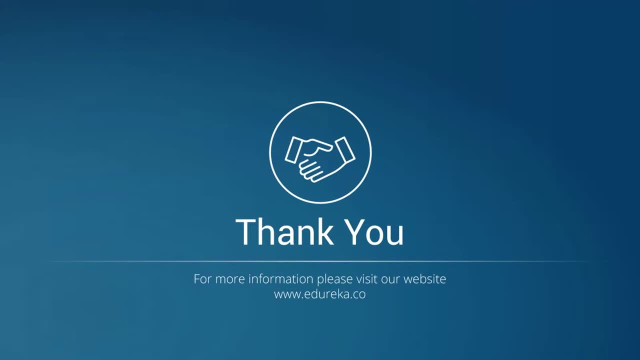 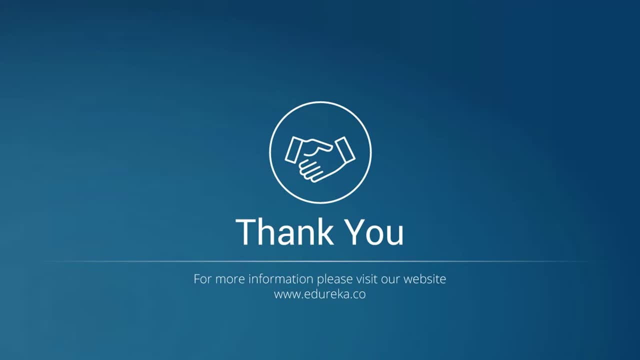 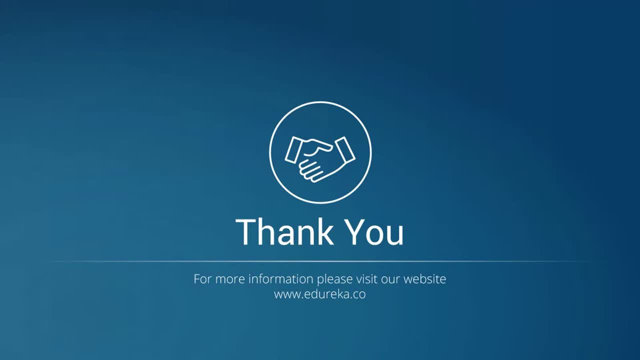 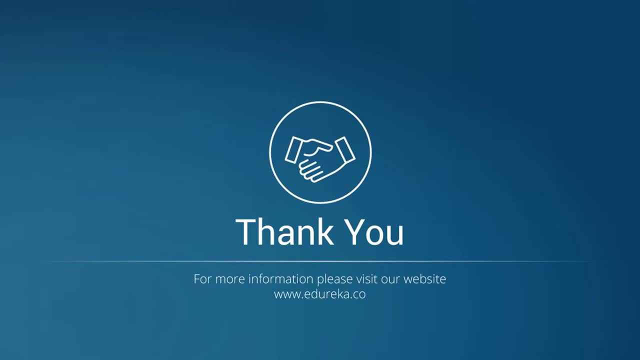 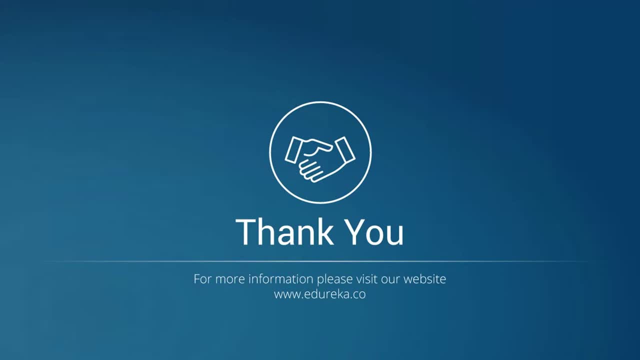 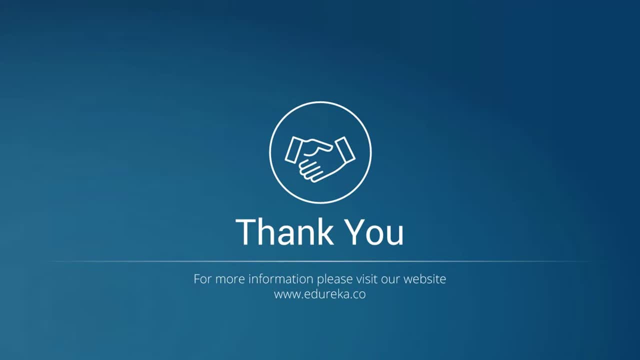 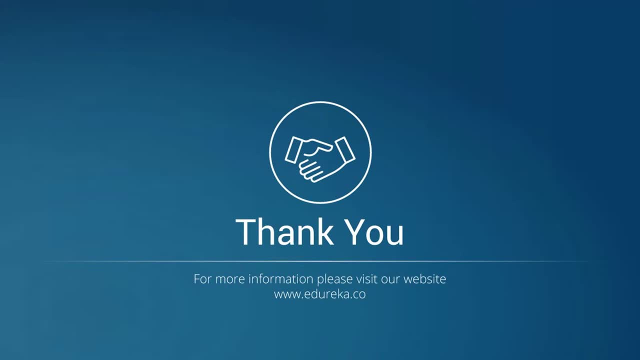 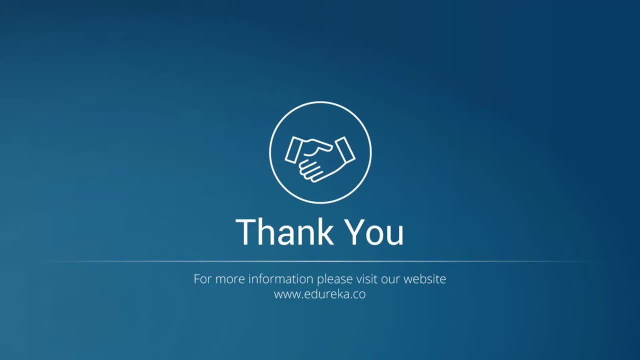 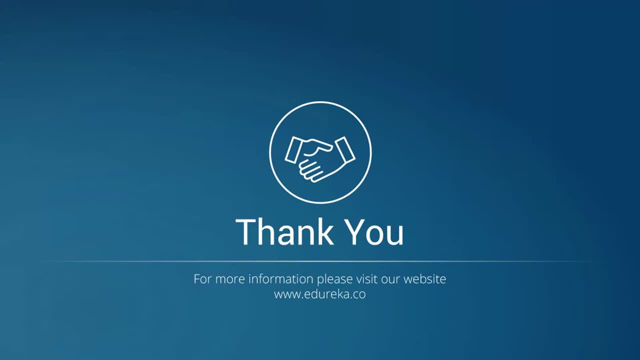 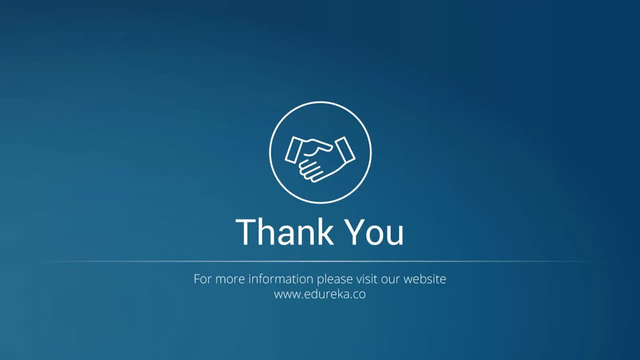 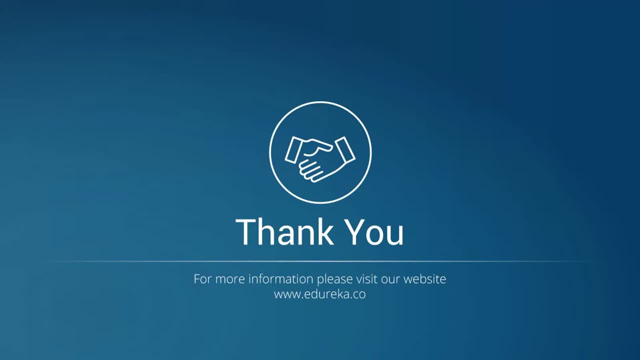 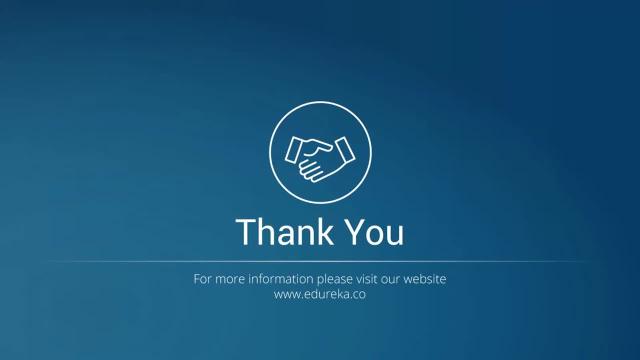 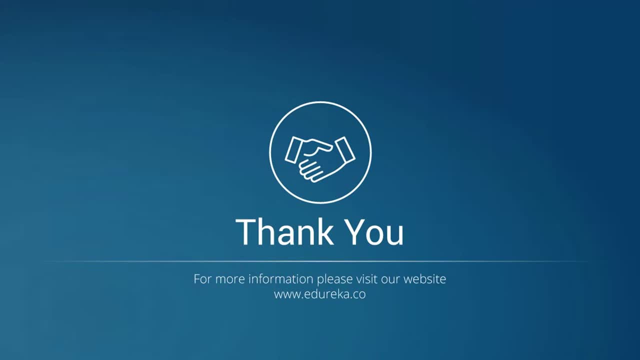 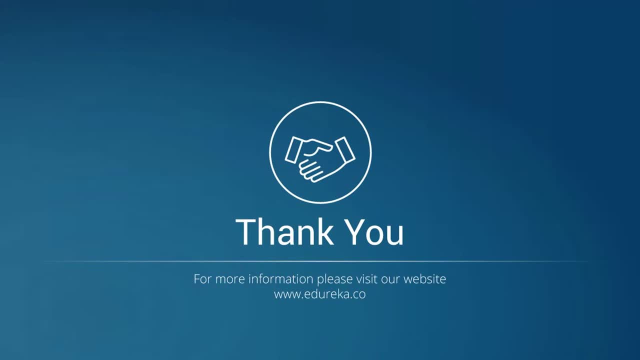